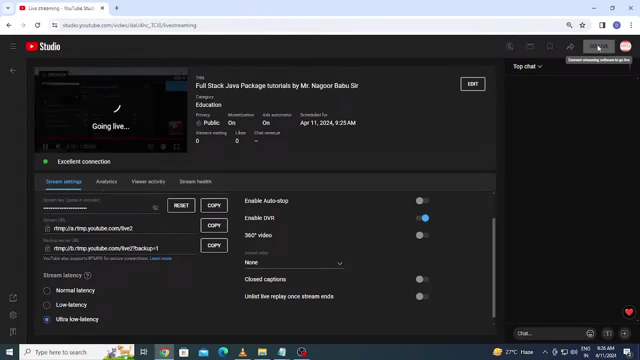 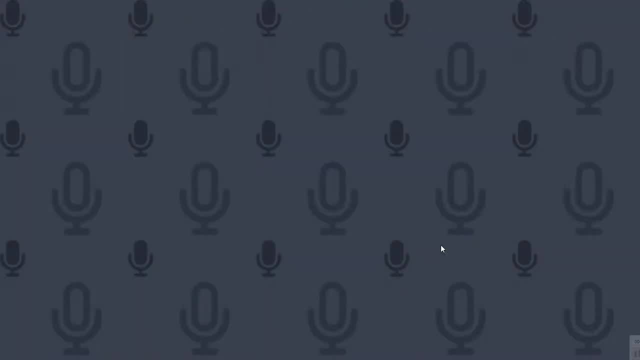 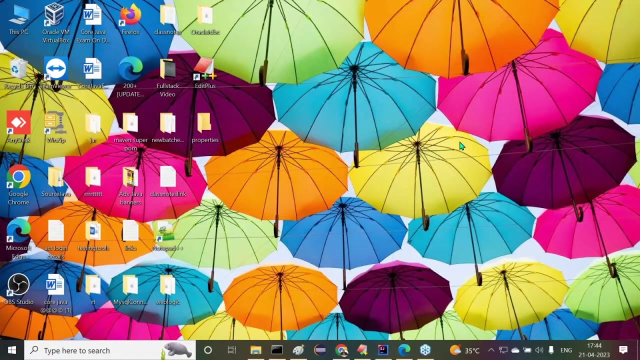 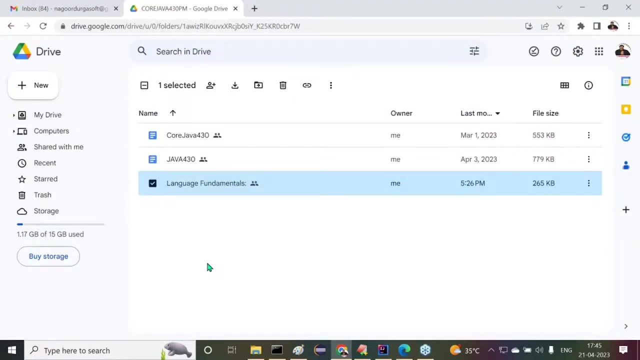 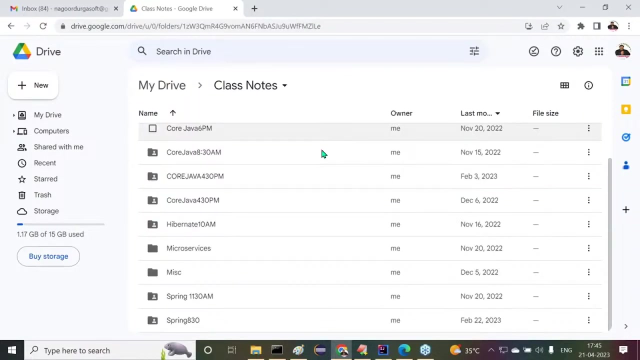 Please confirm to me those who are attending in online. to check it. you guys please confirm to me those who are attending in online. Thank you, Thank you, Thank you All right. Good evening guys. All right, sir, And today just I want to give a small introduction, part related to 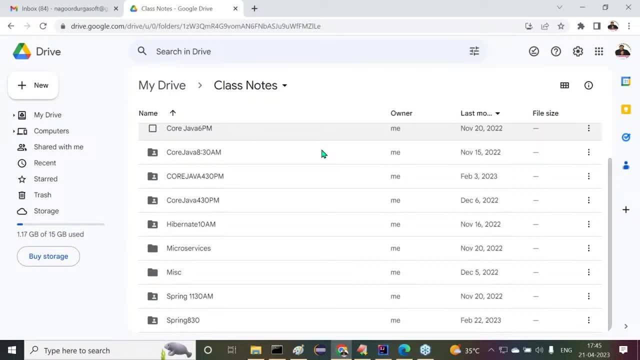 this Java. Just a brief overview of Java programming language. I'm going to give All right, All of you are coming for a demo class. only, right, Right, Thank you. And after that I want to give some clarity about our process, how I'm going to complete these classes, what. 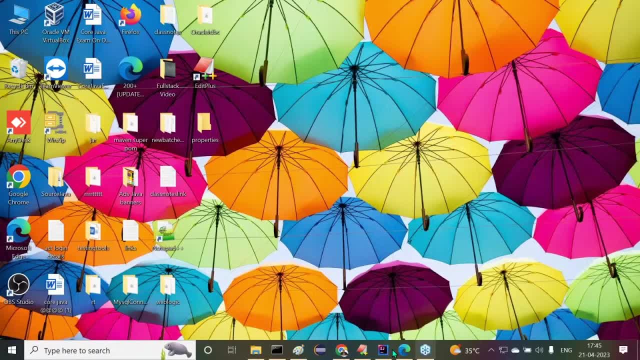 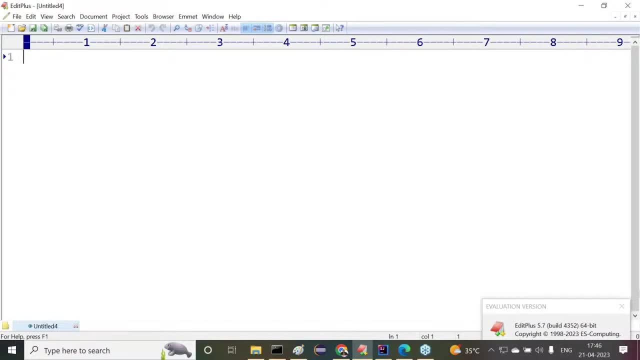 is my plan of conducting these classes, all the things we are going to understand there. All right, Now let's see this point here. First of all, I'm asking one direct question to all of you guys Now, today you're coming for Java demo class, right? Core Java, or whatever? 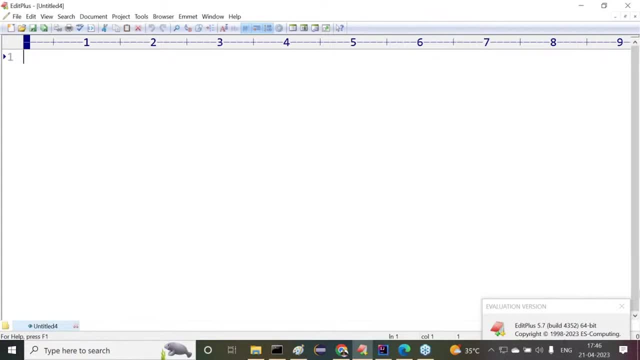 it may be full stack Java, Something else? Simple question, Strike question, Why you are selecting Java now. We have so many technologies, so many programming languages, but still, why we are selecting Java today? What is the need? Because of your parents' force? no, No, sir, My brother is working. with IBM, He earned per month 60,000.. So my parents are saying to us: so your brother is already earning 60,000,, but you're vacant after completion of the P-TECH, So go and join with the classes at Amirpet then. 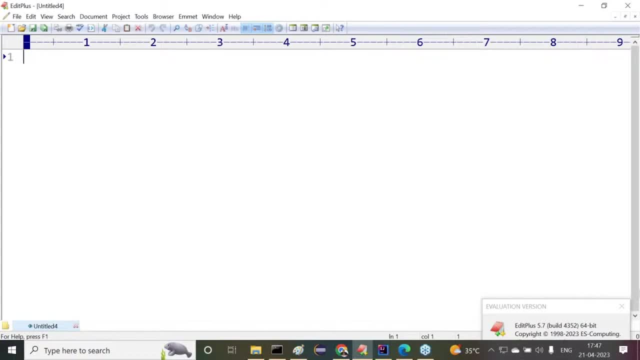 try to get job Because of this. you are coming right. No, sir, I completed my P-TECH four years back. After completion of my P-TECH, I joined with some colleagues there as a lab in church. 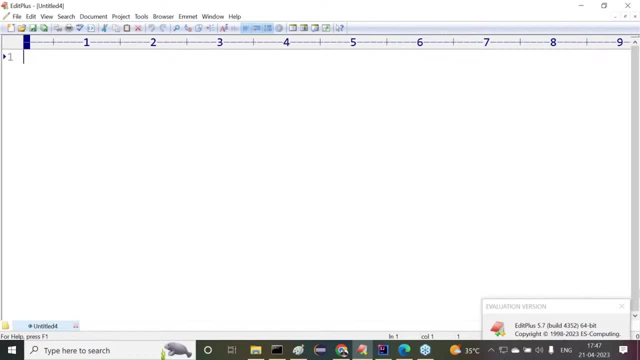 Now I want to go for marriage. Opposite side people are asking to me: if you're the lab coordinator, we don't want to give my girl to you, So try to get software job, then only come here. Is this the reason? Any other reason No. So then simple question: Why you are. 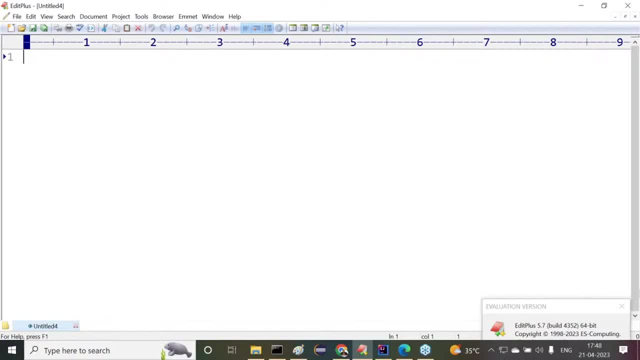 selecting Java. Any reason, Kirno? Definitely. I can give some reasons. All these reasons are funny reasons only, but I think so these reasons may not be available. I think so these reasons may not be available for you. Only one simple, straightforward answer For 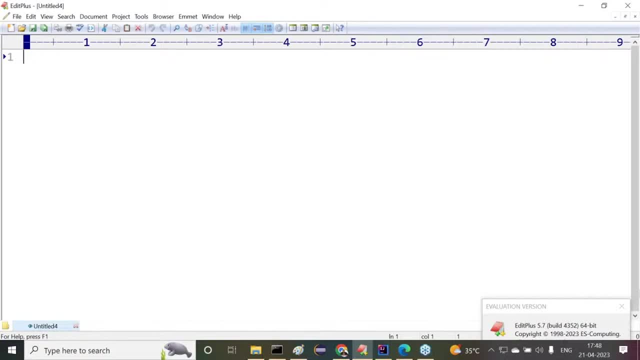 the sake of getting job, for the sake of getting good job. Why is that? Why job is required, Common sense only. I'm asking that I'm not thinking about too much technical questions. Why we need this job? No, because of two reasons. Because of very good identity, As I completed, 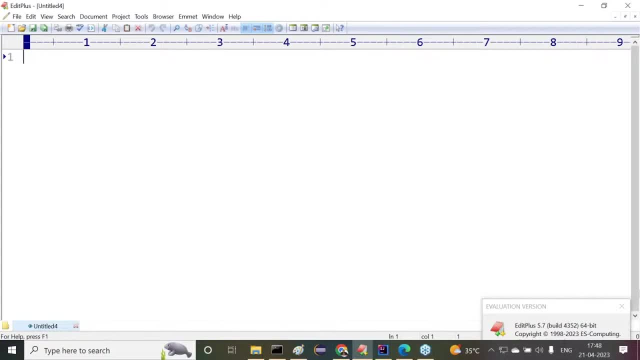 my academics. definitely I have to get some identity. I need some background. So one company background I required. So job is mandatory. That's one point Why job is mandatory, Why identity, Identity is mandatory. Sorry, We are able. 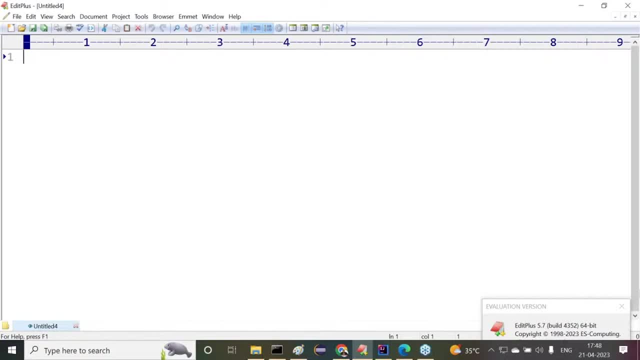 to get job at any field. That is not another deal, But with very good identity getting job is important. So identity recognition, that's one reason. Any other reason, Kir? Second reason, Ultimate reason we have. What is the second reason? Identity is okay. Respect and identity, both are at the same. 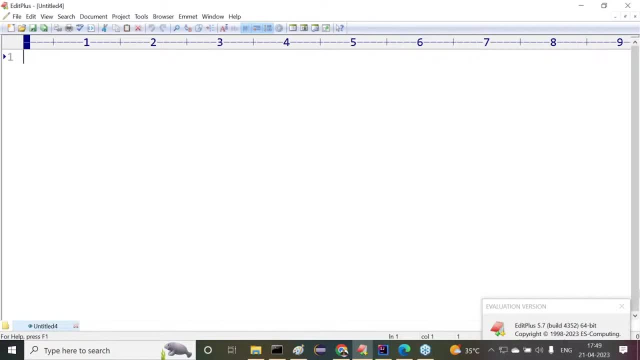 side. Second reason: is there? What is the second reason? Money. Am I right or not? Good amount of money Every month? survival- Definitely we need some money. See if we are giving answers like Sir. I'm very much crazy and programming. That's why I'm coming to this. 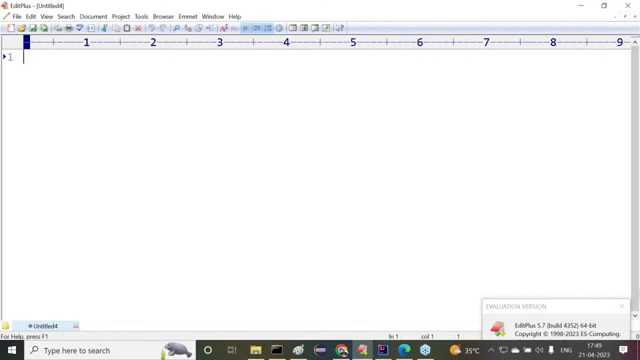 job. No, I don't want to go Believe all these kind of statements. They are over action statements Only. Yes, sir, Am I right or not? Identity with a good respect. And next one is what? Their money. They are the two important factors in our life. Without money, will you work? 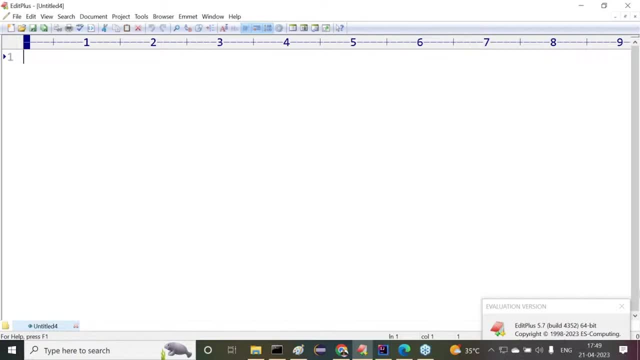 for the one year of time With any company. Will you work for one year of time with any company without money? No, So definitely. money is required or not. That is your fundamental right. We are working with a company for the sake of money only. At the same time, money. 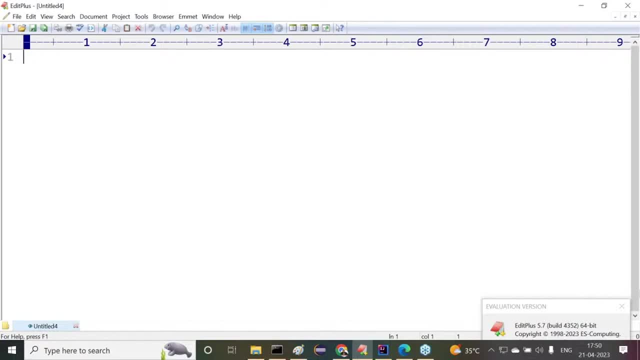 with respect, Money with identity, That both are required, Fine. Whatever it may be, Leave this one. Why I'm giving this kind of discussion here? The point is: watch, If you want to get very good job in order to get money and respect and identity, Java is a right platform, Java. 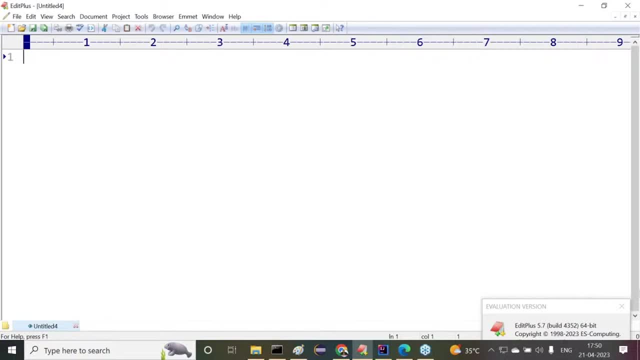 is a right platform at present, as per the outside market situation. Market is not much good. Somewhat dryness is going on there. Understand it what I'm telling you. So, even though this much of dryness is going on, but still, we can trust Java programming language when compared with other programming languages. 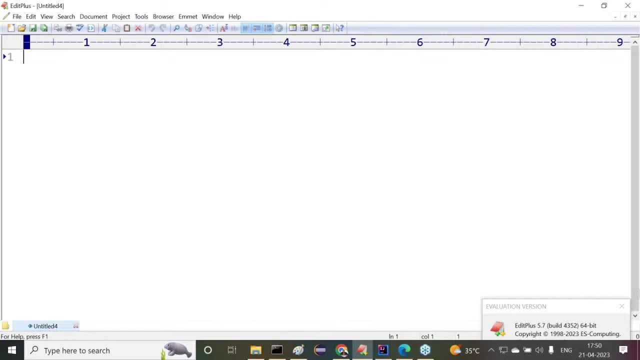 Understand it can. still, some companies are taking Java developers. Some companies are taking Java developers. As for my awareness, I'm telling to you, as for my analysis, as I'm observing that the outside market with the very much close, Maybe next to the next to 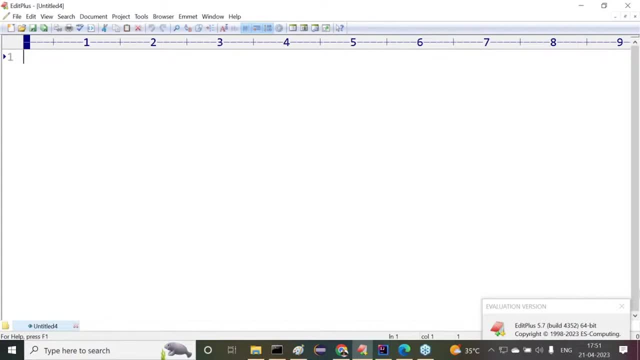 june or july month onwards again, recruitments are going to be start. actually i have 50 companies in my hand at present, regular. i'm in touch with their companies there then every three days, once or four days once. i used to send mails to them. why? because drugasoft is providing 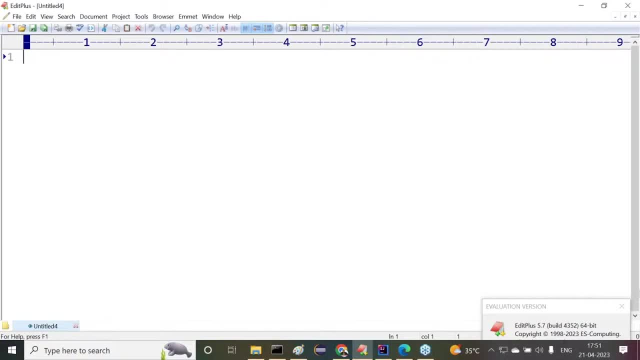 campus drives. also in drugasoft companies are coming. they are going to conduct some recruitment drives on. all understand it. so i'm in touch with almost 50 number of companies every three days, once or four days. once i'm in touch with them, i used to talk with them. 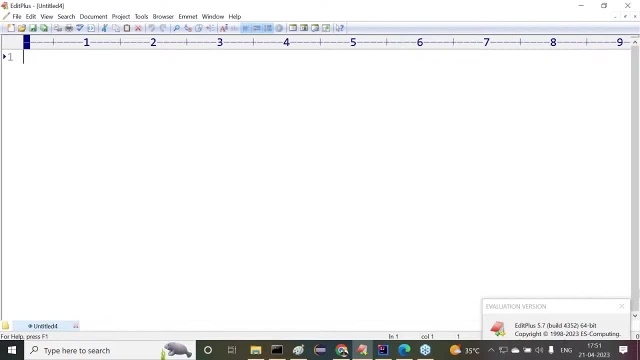 then, what is the status now? what is the status at present? what we have to do like this: i used to communicate with them, so they are giving reply to me, two companies. they are given reply to me on june or july. they want to come here. they are given confirmation even. 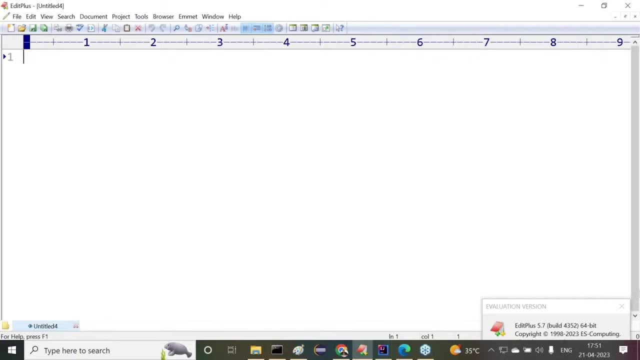 for me. so i'm expecting, in a june or july month onwards again, recruitments are going to be start. meanwhile, you should be ready to attend for recruitment drives in a june or july. now you, but that is the status, what i'm telling you. okay, leave it so, even though the market is. 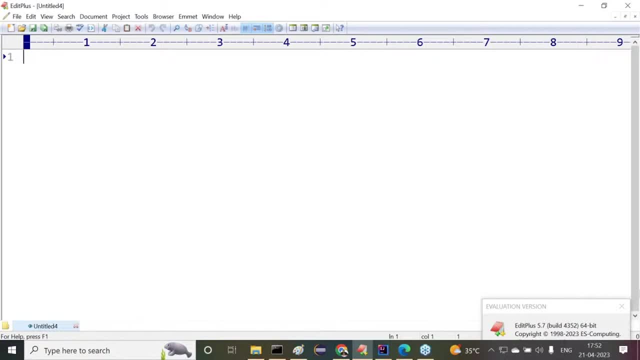 not much good, but still we can trust java. in a java domain, more and more number of recruitments are going to be happen in the companies. definitely, i'm sure about it. i'm giving one statement, i'm sure about it: if you learn java at present, next 20 to 25 years of time, you will not get. 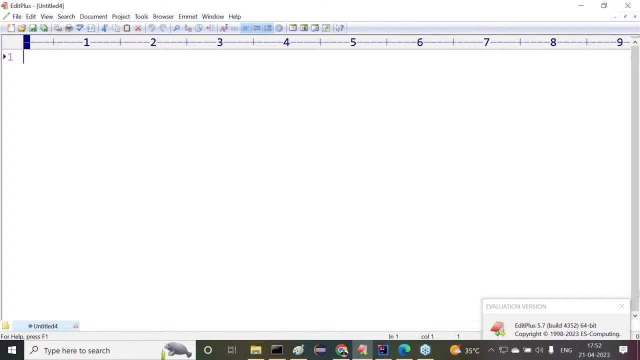 any problem. java is a straight line. see how many people afford that there are. 20 is now people by every year. it's a ahora, but it has front gener and now we are reaching between 15 and 20. monday is not. it's because this is our top 10 percentage. had a little bit of us doing here, no resultカット. 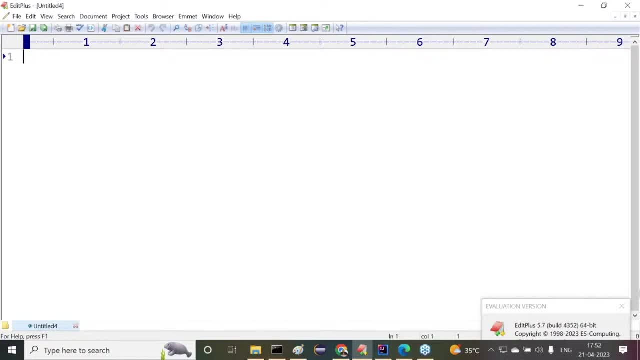 not in there, it's more aboutkę. we'll tell you if we can. can it's actually not. i ran and steel will be already invested now. no, no, we have taken now 30 or something like that. still, what you need now by the time, basically i'm telling in the 30 years to 20 years, in the 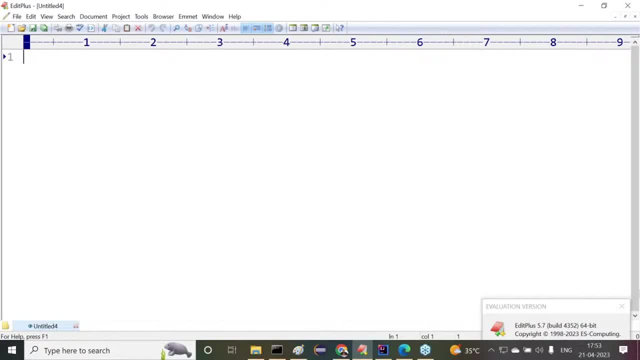 java. we have to determine that in time it has not been built yet and just under 20 years in the past 12 to 45 years. i am showing here you see the quality of it in always it is in of time you will not get any problem in a java domain. this much of requirements are going to. 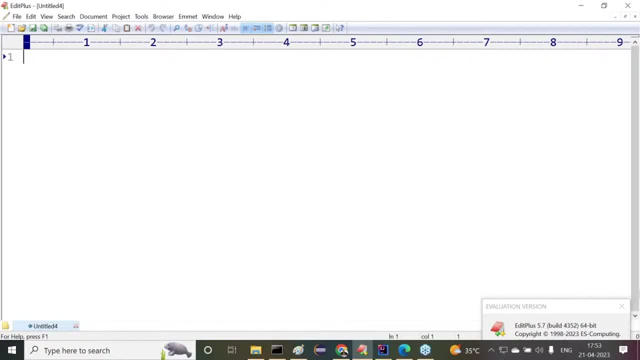 be happen as long as all banks are not using all. as long as all banks are using java application applications, as long as all insurance domain is using java, as long as that entire software industry is using java, you will not get any problem. how long this software industry is. 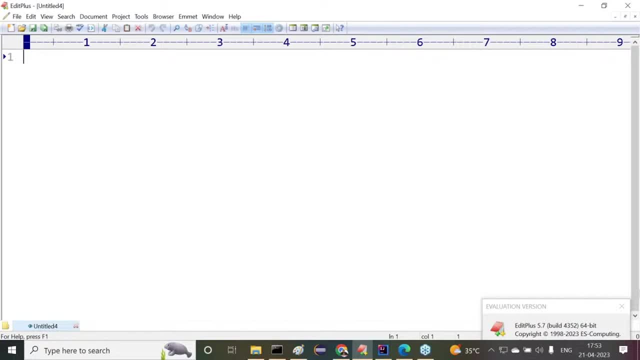 available up to the time java is getting demand. simple comparison: i'm telling that five years back. if you take now everybody, they are giving hype like what there? python is getting very good demand. no, java. nothing is there inside the java. java is totally down. python is getting 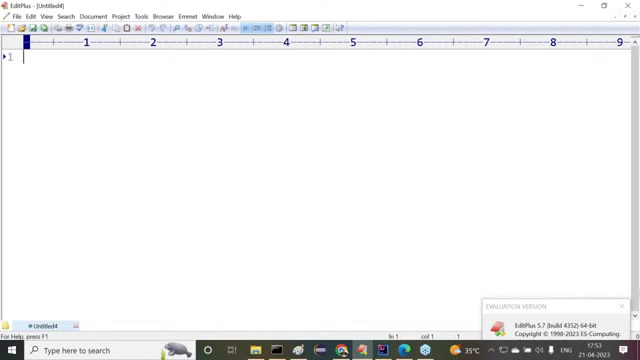 very good market. now see what is the status: no, or the stratus: no. python is not much in high position, python already down, but java is in still the same same situation. java is still in the same straight line even at present. i am telling that number of drives, number of 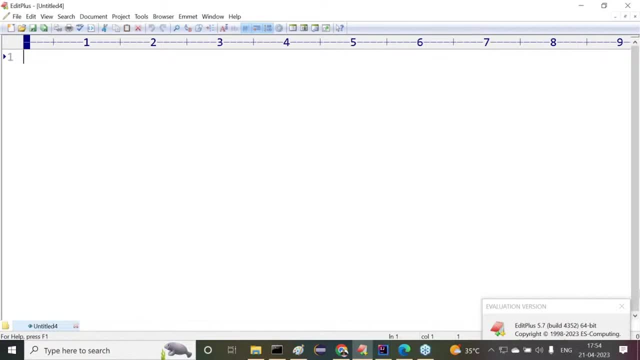 recruitments are going down, going on more in java when compared with other technologies. java and it's related not only- i'm not talking about only core java, java and it's related. there only that majority of the recruitments are going to be happening. because of that reason we are going to have chances to work with what? 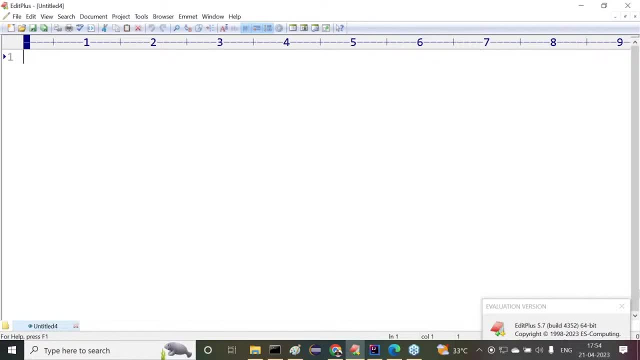 they're to to to have, uh, some opportunities on what? their java domain. so we can trust it. that's the first statement here, what i'm telling you. okay, fine, anyway, leave it here. so for what purpose? you are trying to land java? that's okay, leave it now, but once you have 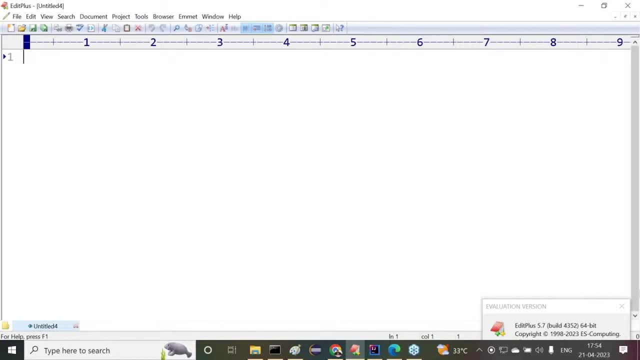 taken the step to land java, then you must bond with that. then we need to have some- like what i'm telling- their patience level and we need to complete it after that. if you try, for java definitely will have very good feature in java there's a confirmation care, what i'm telling. 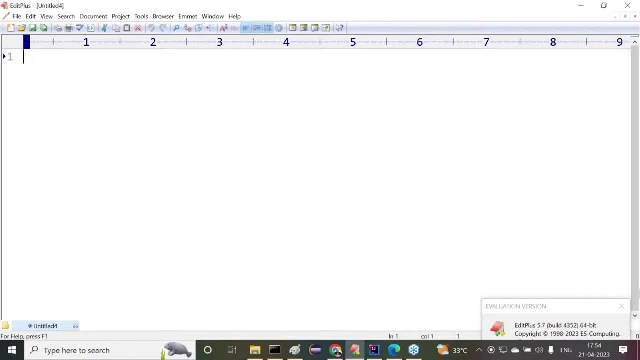 there as a first statement, all right, so before all these things, as you are going to learn java, first of all tell me what we have inside the java, what content that means, what exactly the parts, what exactly the concepts are available inside the java. do you have an awareness on it, what you are having inside the java, do you know anything about this? 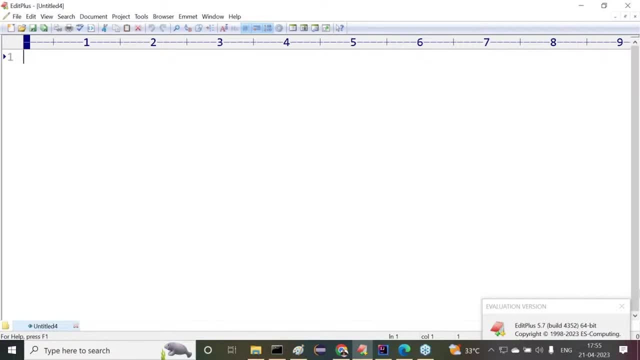 java. if you up to this one, java was provided by sun microsystems. what is the company name? sun microsystems is a company. it has introduced java programming language to outside, say, for example, windows operating system provided by microsoft, a regular database provided by oracle corporation. similarly, java is a programming language provided by sun microsystems. 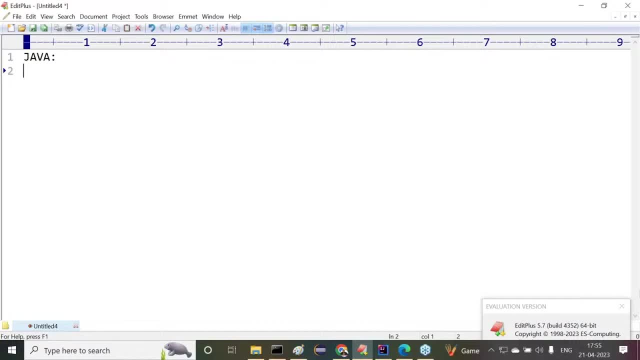 please come. java is a programming language provided by sun microsystems. so sun microsystems as a provided java, in the form of three parts. in the form of what? there three parts? what are the three parts which are provided by some micro systems inside the java, as per our awareness? i'm 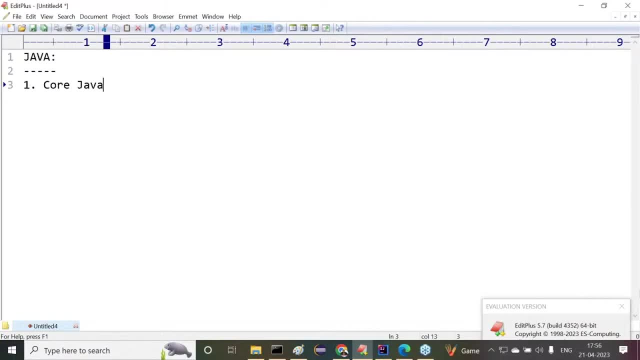 there. first one is what there come on. first one is: what there, core java. and the second one is what they now tell me, advanced java. and the third one is: like what there? j2e? don't write, don't write, don't write anything. understand, just try to understand. so your responsibility is what that? 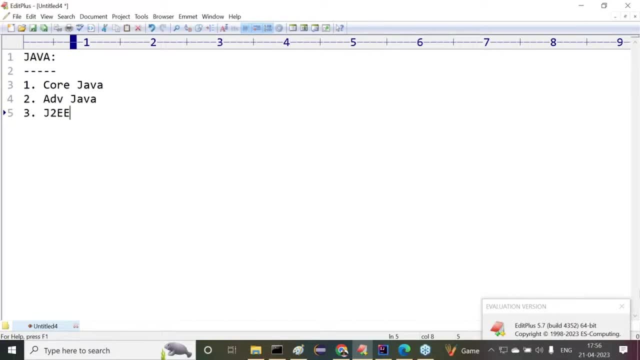 just sit, sit around, that means peaceful. try to understand whatever the points i'm saying, that that's it not required to write anything in my classes. why? because whatever the things you want to write in our notices, no, i will write in my laptop. i will share the document to you everything. 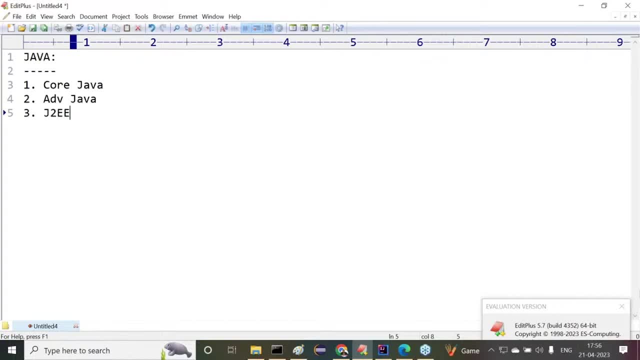 i will share, don't worry, at the end of this session i'm able to give some clear-cut picture for it. try to understand it now here. now the point is like what i am telling there. java was provided by sun microsystems in three parts. can you tell me what are the three parts? no core java advanced. 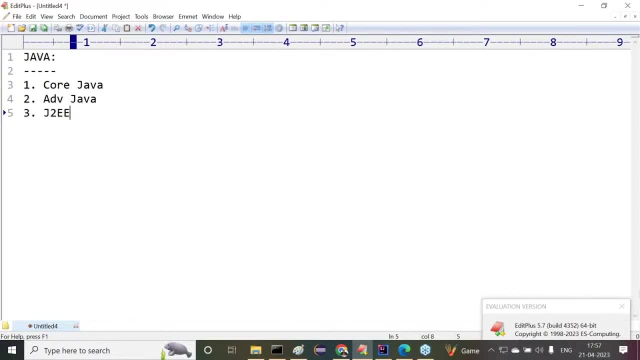 java. what is the third one, j2e, clear or not? this is totally wrong. classification was totally wrong. everybody is following this kind of terminology only, but this is wrong. this is unfortunate. this is wrong. this is not the right classification. what sun microsystems has given? this is only local terminology. more clearly, amirpet institutes have given this kind of 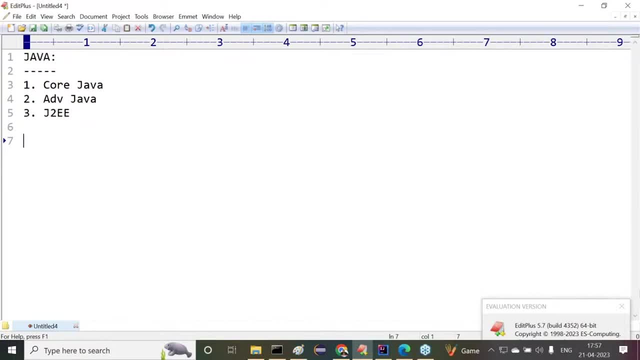 classification as per their business, of course, not only amirpet. i'm telling that institutes have given this kind of thing. bangalore institutes are maybe chennai institutes, whatever it may be now. so this is not the terminology which was provided by sun microsystems. okay, sir, good, this is not the right technology, but 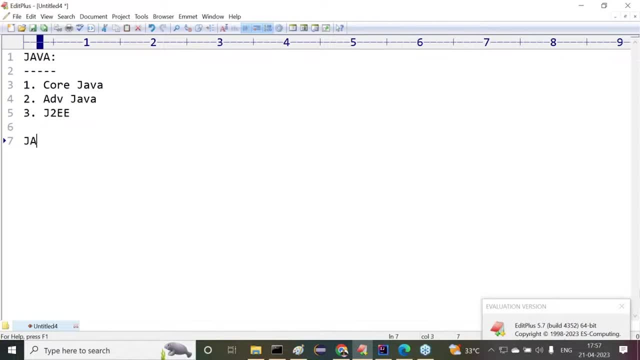 what is right terminology, what is right technology, if you have to. this java was provided by sun microsystems in the form of the same three parts. no, but what are the three parts? care, first one is j2ee or java se. of course, almost all we can say it is a core java. 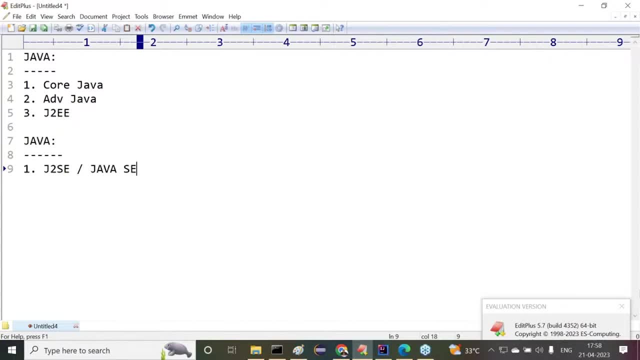 but that core java terminology is not available. but we can say it is a core java equivalent and the second one is what there. second one is j2ee or java ee. second one is what there- j2ee or java ee. and the third one is what there- j2ee. 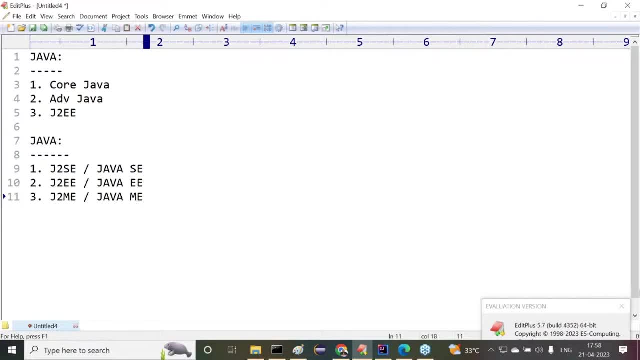 or java me j2me, or java me j2me, or what there? java md. so all of you are getting it or not? now tell me. now tell me. java was provided by sun microsystems in the form of three parts. what are the three parts? no, j2s, key, j2ee, j2me- what is not available. 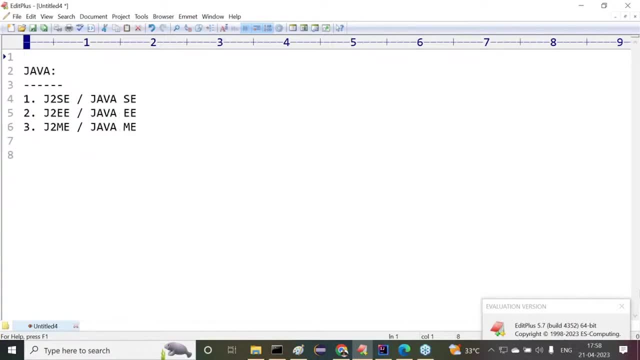 this is not available. i want to delete this. not right to understand it? no, just let me delete it. not required, that is a totally wrong terminology. but in outside, everybody is following the technology only because of the reason. as a first point in my classes, i am telling you clearly that 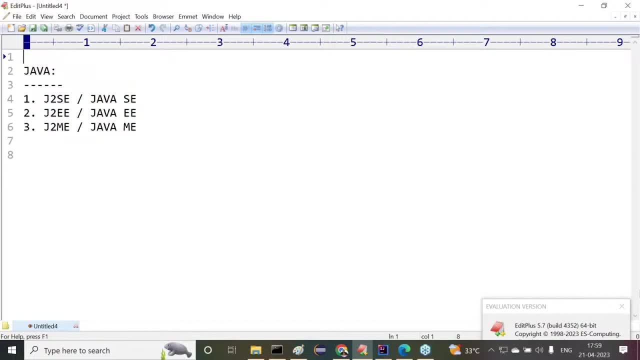 terminology is a wrong terminology. this is right terminology that we have to follow. clear, sir. j2 eski, j2ee and j2me. good, that's okay, fine, but what is this j2se actually, what it will cover, what we are able to get from this j2ee and j2me. 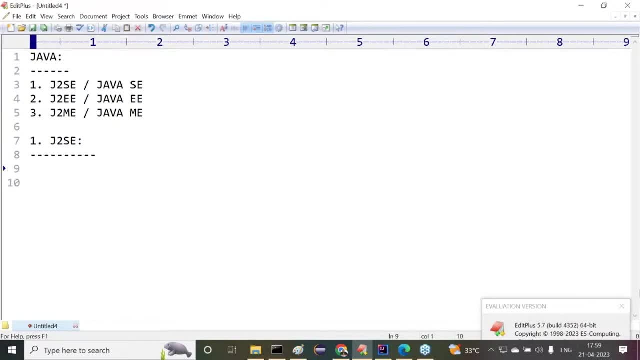 j2eski what we are able to get from j2eski. right simple points. try to understand it clearly. java 2 standard edition. java 2 standard edition abbreviation. i'm telling that good what it will provide. it will provide only, only fundamentals of the programming language. 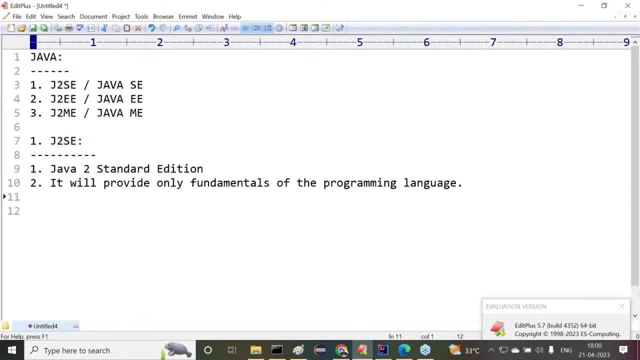 what it will cover. now tell me only fundamentals of the java programming, not complete java. see: if the total java is provided by j2sk, then what is the requirement to go for j2e and j2mg? i get my point, or not? so j2se is providing only fundamentals of the java. 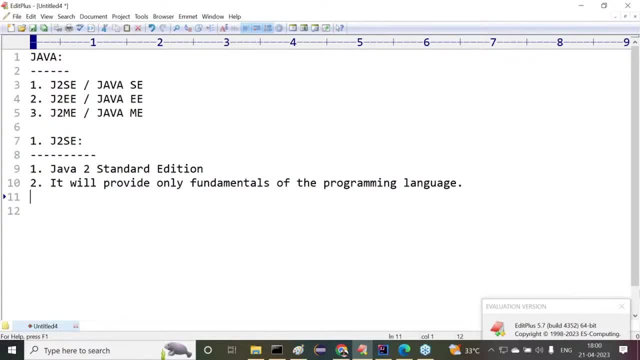 by using these fundamentals, what we are able to do? do you prepare any application by using fundamentals of the java? with only fundamentals of the java, is it possible to create any application? understand it clearly. by using j2se, we are able to create, we are able to prepare. listen, all of you know. 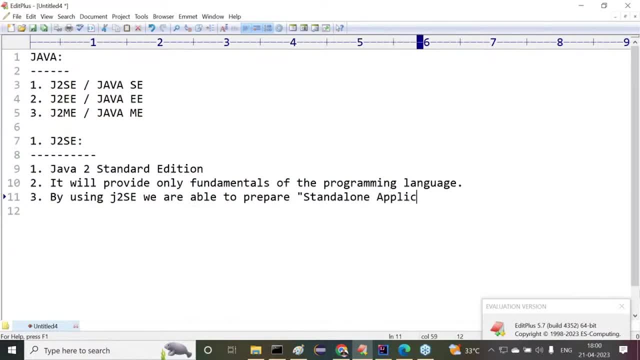 standalone applications. come on, guys. or what is this one here? actually? standalone applications. by using fundamentals of the java- and i'm saying that by using j2se, i'm telling there- or maybe by using fundas, by using fundus, by using fundamentals of the java, we are able to prepare what type of applications? they're not telling me. 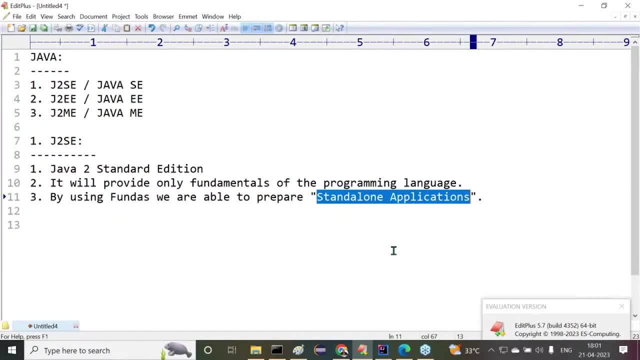 come on stand alone applications, then immediately i'm getting a question, sir, what is this standalone application? okay, j2se, only fundamentals of the java. by using fundamentals of java we are able to prepare standalone application. okay, i do agree that. but what is this standalone application? what is the meaning of the standalone application? answer is very clear. try to understand. 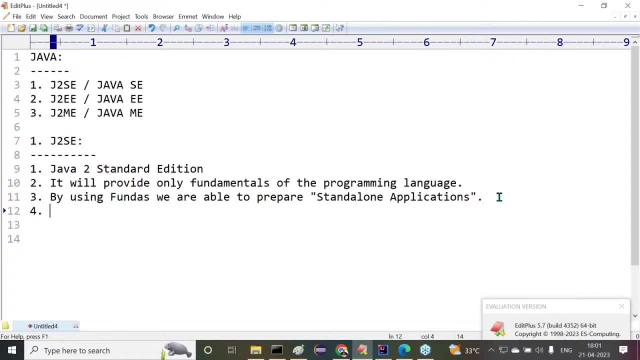 it now. listen, i'm giving clarity. try to understand it now. if we design, if we design and execute any application, all of a clear up to know, if we design and execute any application without using- come on, what is this? no, without using- client server architecture. you know there is a design architecture, client server architecture, client will. 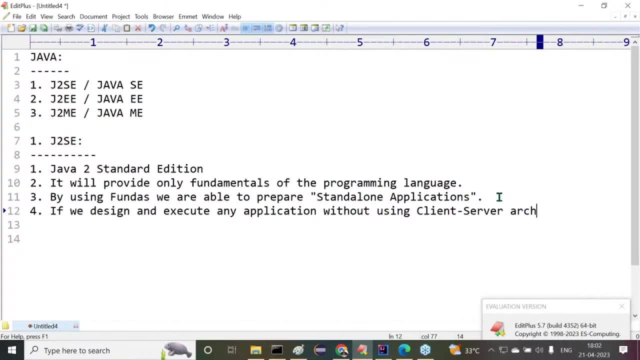 send request to the server. server will perform some process. server will send some response back to the client. this is what client server architecture. i'll forget my pointer: client server architecture. okay, if we design and execute any application without using client server architecture, or or listen carefully, without, without distributing. 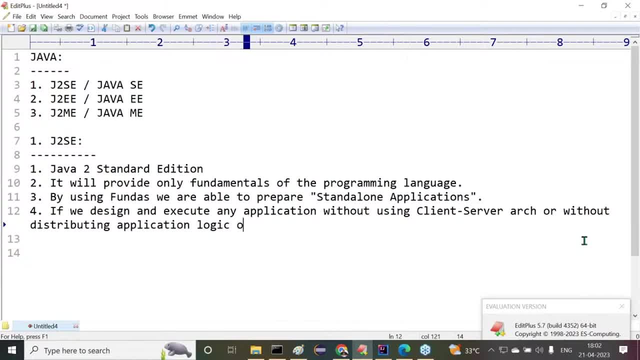 without distributing application logic over multiple missions- missions in the sense computers- without distributing multiple missions, then that application is. then that application is what their standalone application right. all of you understand this point clearly. please read out the definition here. whatever the definition you have given there, clearly understand it. it's very simple definition. 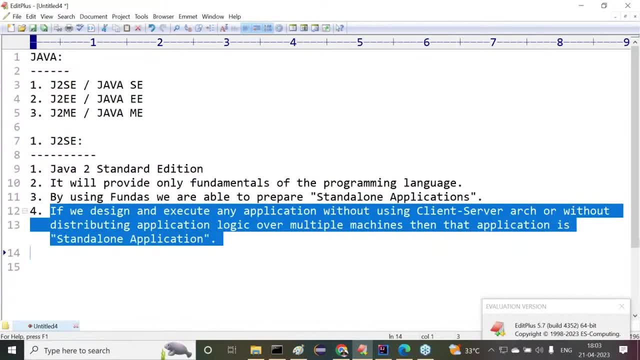 here. try to understand each. try to analyze, try to understand while reading the content. we have to understand what i'm telling them. if we design and execute any application without using client server architecture, hold on here. client is one mission, server is another mission. some program we have to write on client client mission. some other program we have to write on. 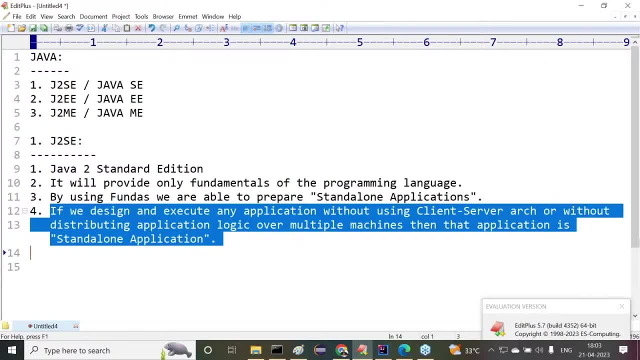 what their server mission means that my application is distributed over multiple computers or not. in a client server application my application logic must be provided: a client mission and server mission or not. that i don't require. that is not available in my application development. there is no concept like client to server application. there is no concept like what? 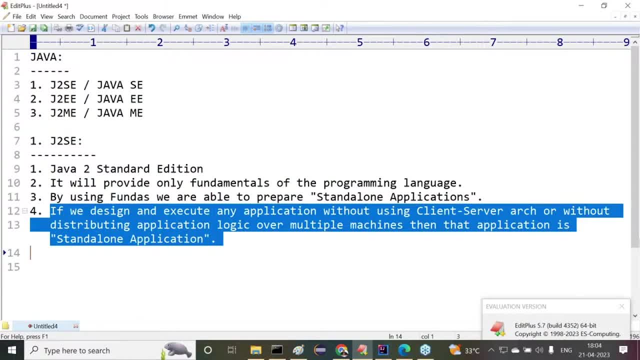 their client server architecture. so, without using client server architecture or without distributing application logic over multiple computers- my application logic must not be distributed over multiple computers- then that application is called as what? standalone application. it means that my entire application i have to write and i have to execute within a single computer. 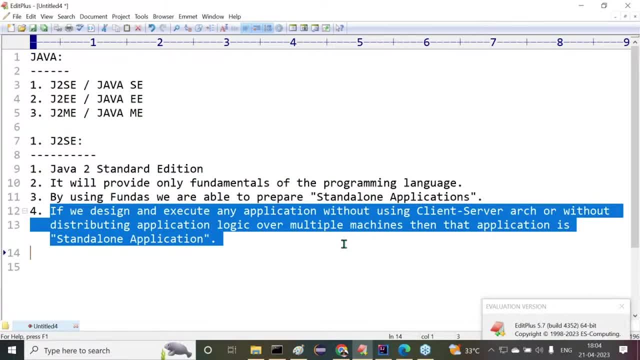 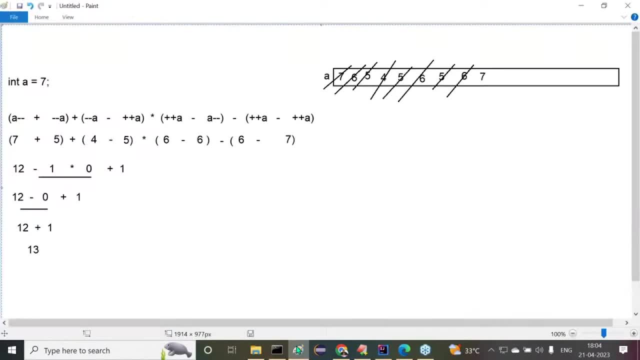 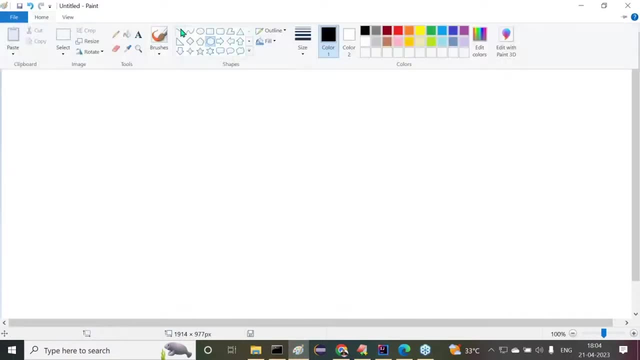 and directly what i am telling there. my complete application i am going to provide within a single computer. are you able to follow or not? see this punch? here i want to give a simple diagram, you know, try to understand this diagram. so this is one computer, so right, this is one computer. now, inside this computer only, I'm going to insert 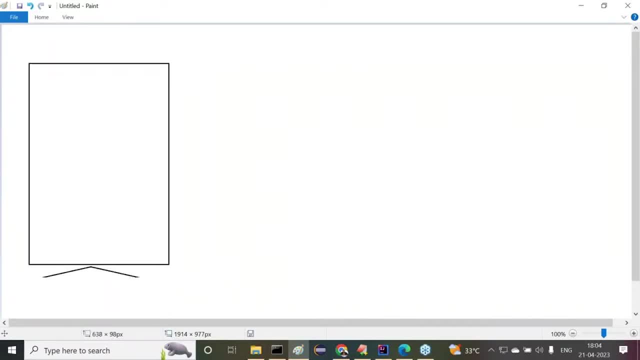 this computer. only. I'm going to prepare my entire program. now get, this is what I am telling here: my application. everybody understand this clearly. now here I am going to prepare what there? some application logic. my complete application is available inside this particular mission, only my total program. 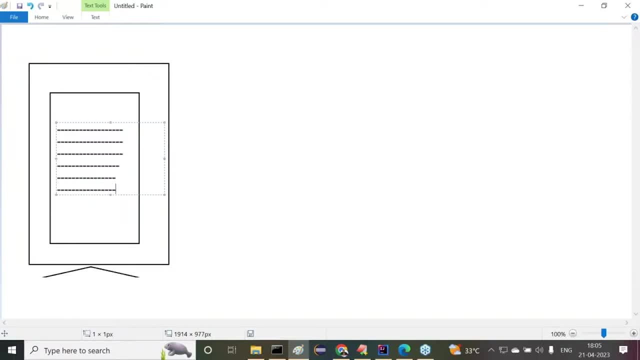 is available inside my computer only. this is the logic, this is my code. whatever the instructions get, I want to prepare. this is my coach, now computer. I want to say it is what their mission and this is my program program. I want to say it is what their application, total application, I have written within a 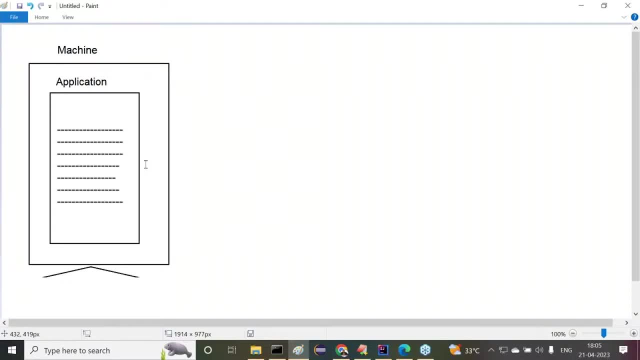 single computer. they roll. I am compiling my program. they roll. I am executing my program. my program is asking to me enter some input data. I entered input data in the same computer. my program is giving some output to me in the same computer. I am able to test my application within the same computer. everything about my. 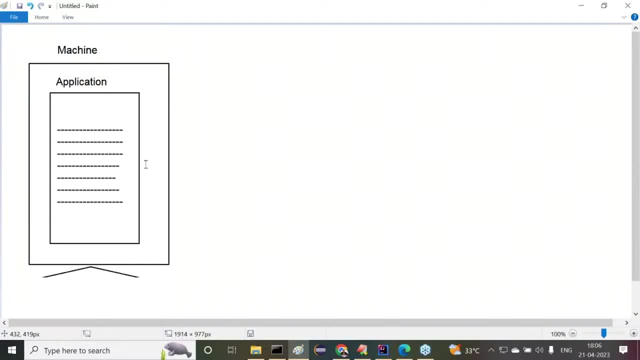 application is going on in a single computer and their application logic is provided in a single computer. this type of application is called standalone application. hello, if you're following or not, this type of application is called as what? their standalone application. to prepare the standalone applications we required, 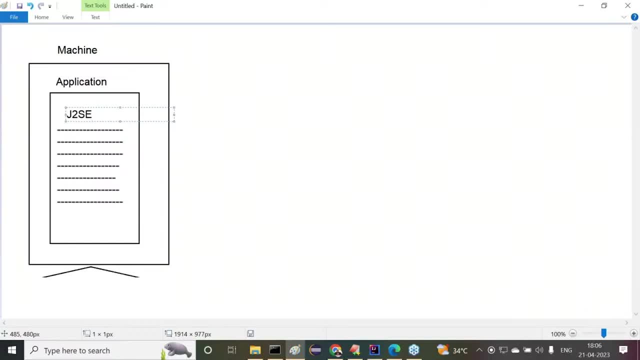 what technology, what programming language we require J2SE, Java 2 standard edition to prepare these applications? only fundamentals of the Java is a sufficient, only what is sufficient gear. fundamentals of the Java is a sufficient, not required to go for too much Java programming languages. is that all? if you're following or not? that's okay. now this is. 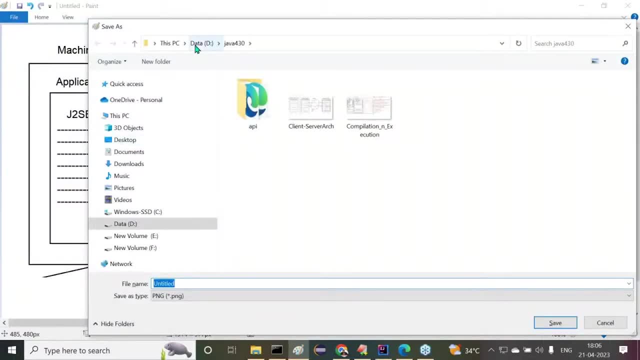 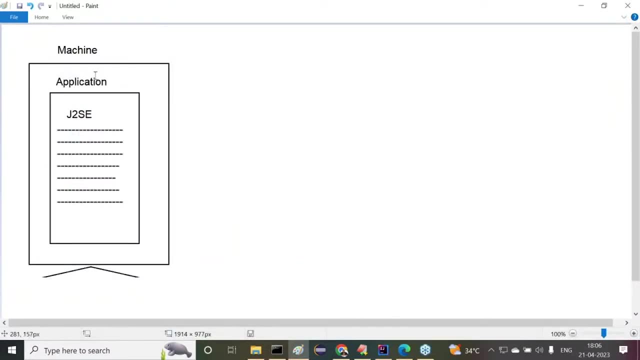 clearly the diagram. don't worry, this diagram also I'm going to include there. in the future I I'll provide even this diagram also to you in the document. right, sir, clear? this is exactly the meaning of what their standalone application. okay, sir, understood. sir, clearly I'm getting some point. 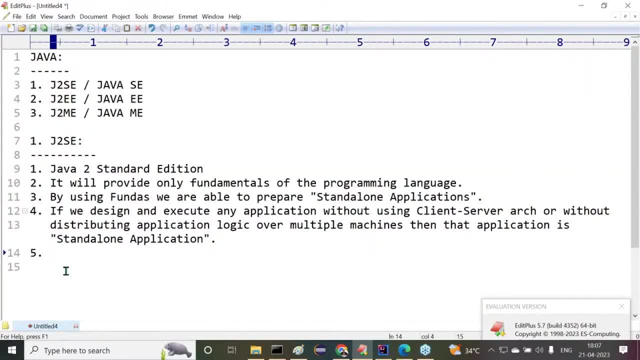 here. what is the point here? I'm getting there. J2SE is a Java 2 standard edition. it will provide only the fundamentals of the Java programming, not complete Java. with only fundamentals, I can prepare standalone applications. what is standalone application? design and execute Java application- any application- without using client server architecture or without distributing application. 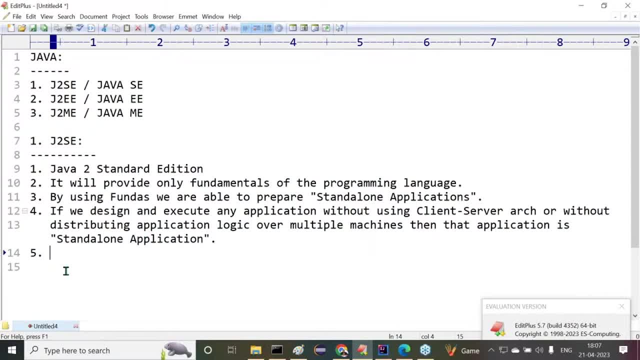 logic over multiple missions or by providing entire application logic in a single computer, then that application is what their standalone application. okay, good, up to that, okay understood that. now tell me, sir, how many applications are standalone applications in outside? in outside, so many applications are available. so many computer applications are available out of. 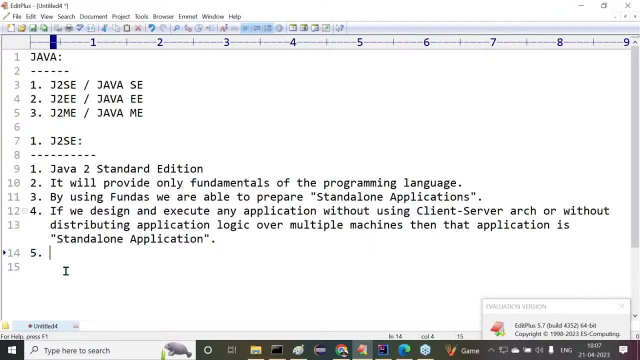 all these computer applications, software applications, how many applications are standalone applications? what are the examples for the standalone applications? can you tell me right? I can give some examples after that I will give ratio. understand it? what are the various examples? here I'm telling to you: laptop, right inside my laptop, inside my computer, calendar is available or not? 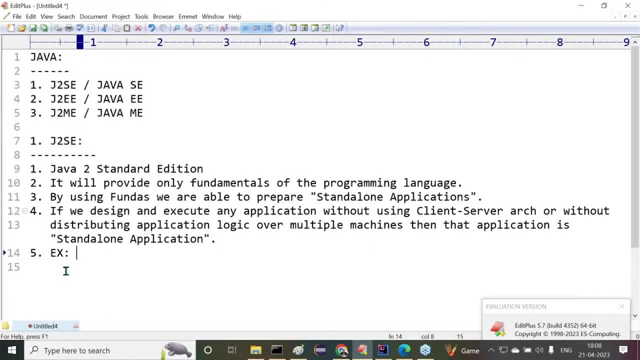 can I get calendar or not? come on, guys, that calendar is also an application. that application is available within the same computer. am I right or not? so that calendar, that calendar, is what there is an example for standalone application. leave this one inside my computer. calculator is available or not? 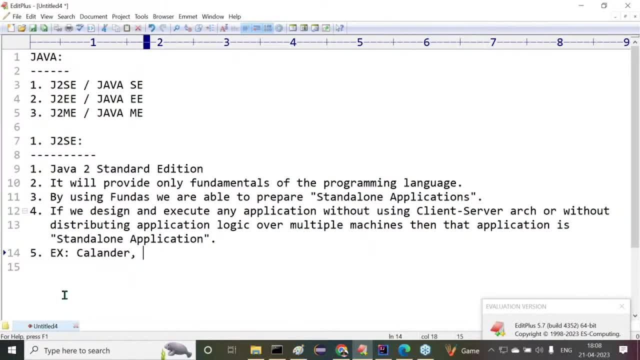 come on calculator. calculator doesn't distribute its logic over multiple missions. that doesn't require client server architecture. hidden my single computer. that calculator is running or not. alright, so now calculator is an example for a standalone application. say for example: for the sake of diagram, I open this paint shop. this is what they're. 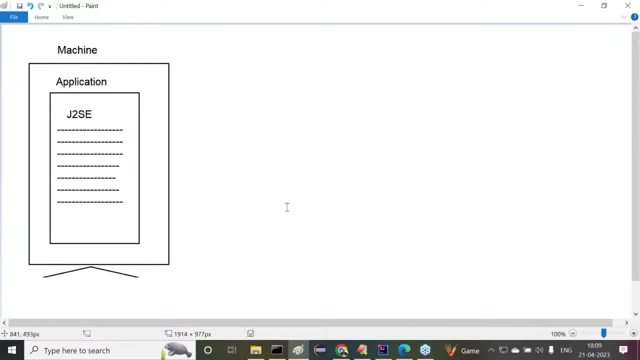 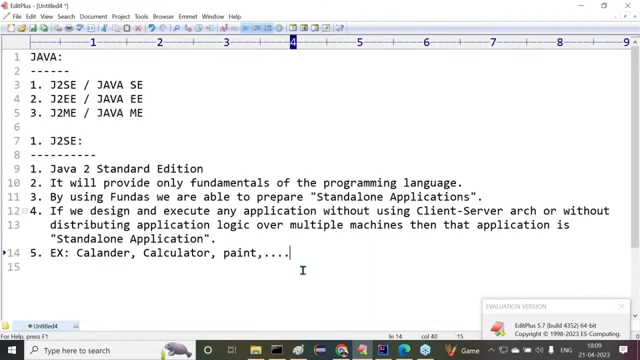 painted. I am right on, a paint is also an application. all right, this Inter is also be what their, a standalone application, and so on and so on and so on. so many things are available: calculator, calendar and so on. all these things are what their standalone applications clear. that's fine. all right, sir. good, these are the examples now, but how many? 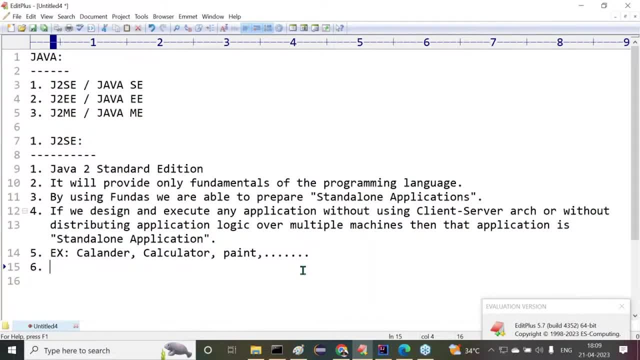 applications are standalone applications in outside. how many applications are standalone applications in outside? if you observe this punch here, I'm giving clarity now. try to understand it now. only only five personas of the applications are stand-alone applications only. how many applications? no five persons of the applications, or what stand alone applications? only five. 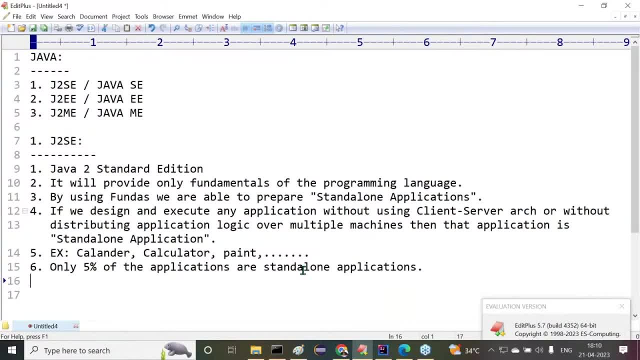 persons of the applications are what? standalone applications? yes, clear. all of you following these points. no good, remaining 95 percent of the applications are not a standalone applications. only five percent of the applications are what they're: standalone applications. clip now try to understand it clearly after this: 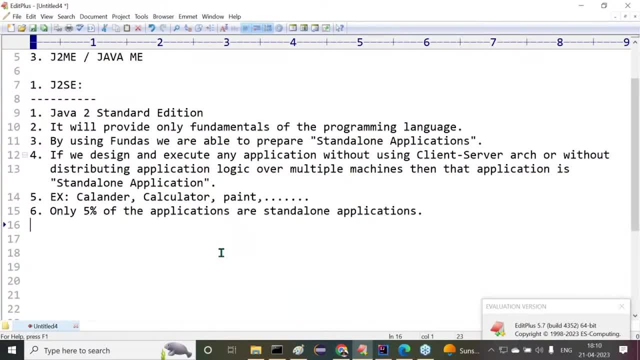 application development is only five percent about the standalone applications, about j2se, but it is a okay, it's a direct utilization. j2se direct utilization is only five percent, but it's a dependency level, but it's a dependency level, it's a dependency level, it's a dependency level. 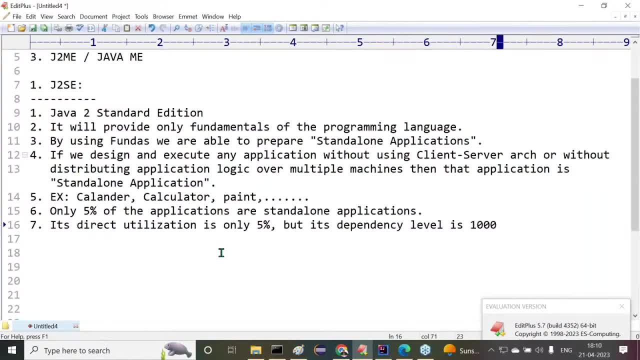 level is a thousand person is. that is this punch. it's direct utilization is what there only five person is, but it's a dependency level is what there thousand person is. sir, what is this mathematics today? five person is and thousand person is. I am not getting clarity. what is this actually? I will give some clarity. understand it now. 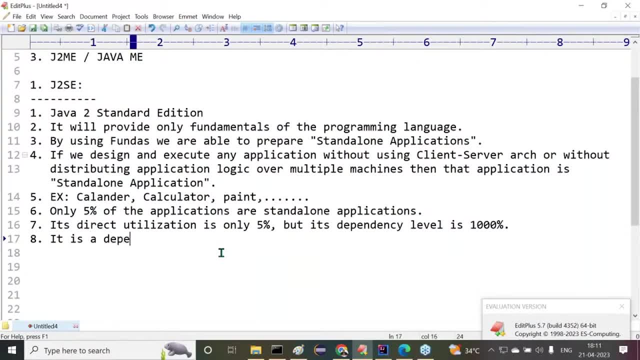 it is a dependent programming language, for it's a dependent programming languages for number one: to learn j2ee, instead of saying that learner to work with, to work with j2ee technologies. if you want to learn advanced level, we must require core level or not. if 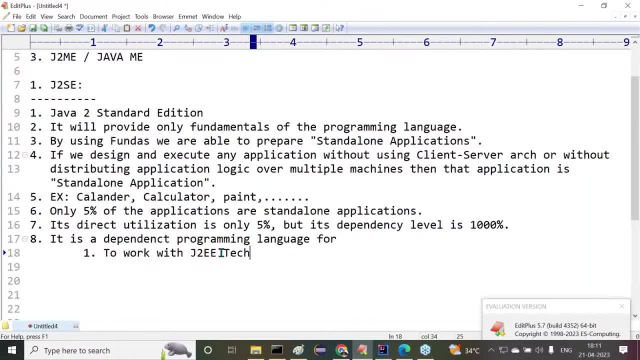 you want to construct a building, foundation is required or not. that foundation is what the j2ee- that remaining part of the building- is what their j2ee. if you want to work with the j2ee technologies, what is required- j2ee is required. that's why I am saying that it. 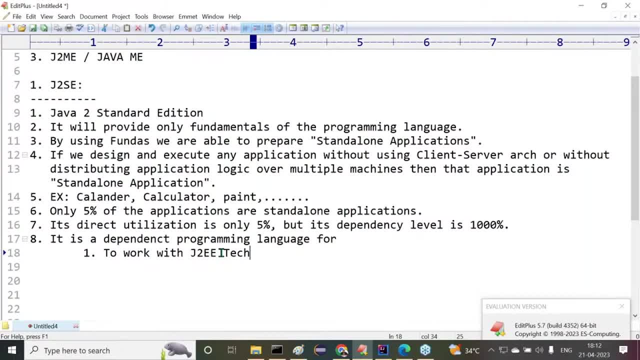 is a thousand person is dependency level. it is required. thousand person is for other technologies. I am so carefully and other one is like what I am telling there. apart from that, I am telling that the j2ee technology is required to work with, to work with selenium, selenium testing. 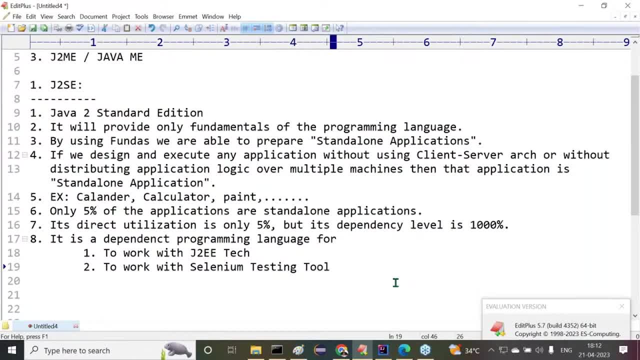 tool- I think you already aware about it- selenium testing tool. selenium is one of the tool for the sake of the automation right, automation testing. selenium is one of the tool. if you want to learn or if you want to work with the selenium, you must know j2ee without having 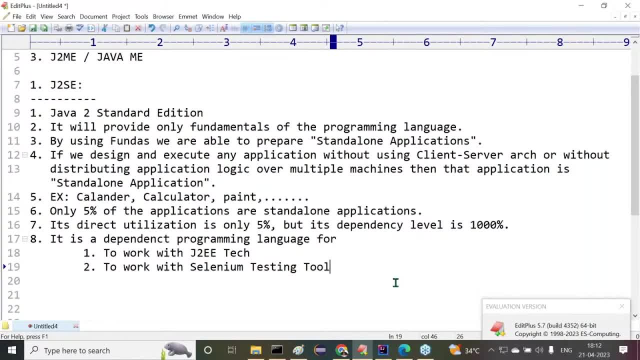 j2ee knowledge. you are unable to do anything with the selenium, but selenium is also another tool on there in outside. next one is what there? in the same way, sales force. if you want to work with the sales force or if you want to learn a sales force tool again you require 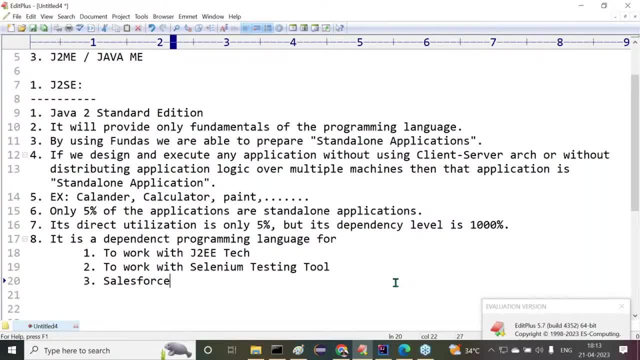 what there? j2ee is the part. not only that. if you want to work with the hadoop, do you aware about it? no, hadoop is a big data analysis. if you want to work with or if you want to learn hadoop again, what is required you know. j2ee. 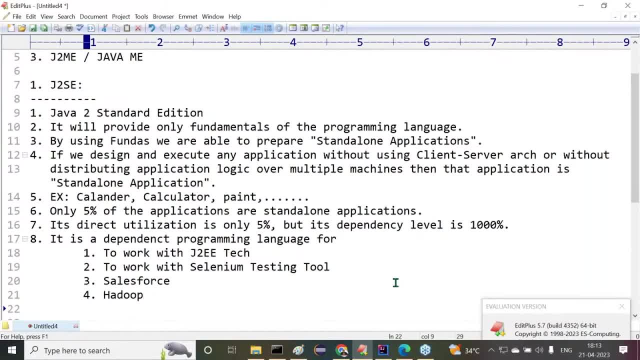 know j2ee is required. or if you want to work with or if you want to learn a seap related tools, abap, or maybe some hr or maybe something else, if you want to learn sap tools, sap tools- that again what is required. you know j2ee is required. not only that: if you want to work, 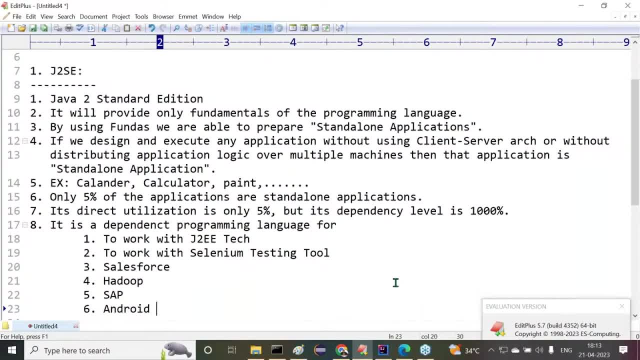 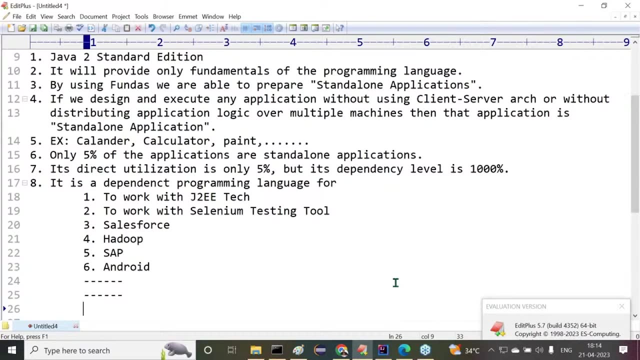 with the android mobile application development platform. if you want to work with the android mobile application platform there, definitely we require what? there j2ee, so many. not only this, just only some of the products list i have given there and so on. so many everything. almost all. 90 percent of the software products nowadays are depending 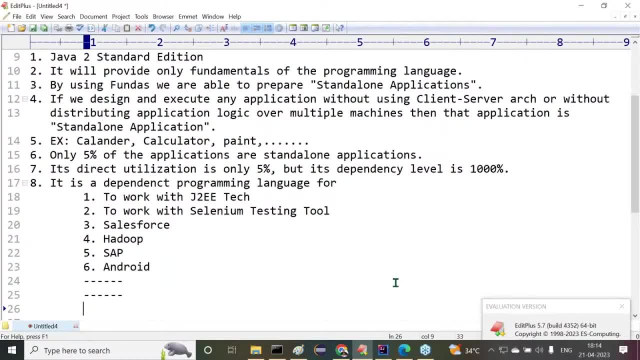 on what there j2ee is. but j2ee direct utilization, is only what five percent is, but it's a dependency level. is what there? thousand percent? because of all these many things, if you want to learn sales force, want to learn selenium testing, or if you want to go with sap tools, or if you want to learn adobe. 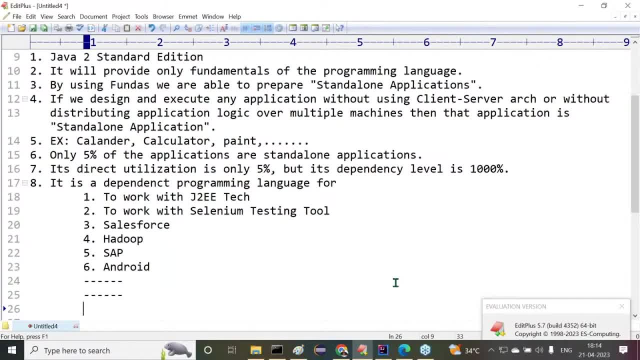 for all these things, one prerequisite is need. what is that prerequisite here? j2 sc patch. so it's a dependent programming language or not? that's where thousand person is dependency level is available over this particular programming language. yeah, because of this reason also, we might be. java is not having any downfall, always java is having what there. 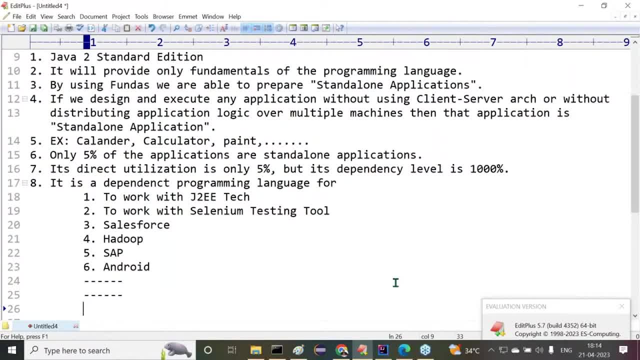 upgrade. that means the upward arrow. you can understand it clearly. that's enough. this is what exactly the information about. what are there? j2 se guys, tell me what i discussed here up to now, point by point. i have given that. first of all, tell me what is abbreviation for j2se. 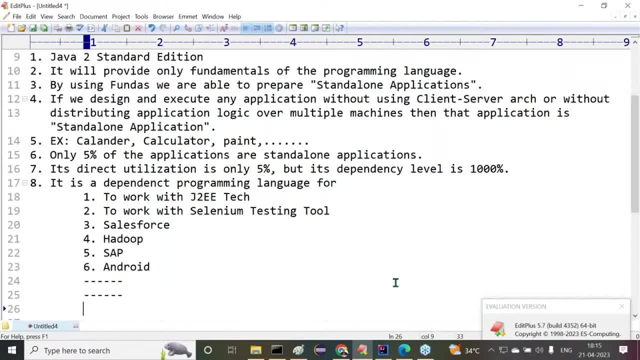 java 2 standard edition. what it will cover. what it will provide only fundamentals of the java by using these fundamentals. what it will provide only fundamentals of the java by using these fundamentals. what type of applications we are able to prepare standalone applications. standalone application is using client server architecture or not using client server architecture. come on, using client. 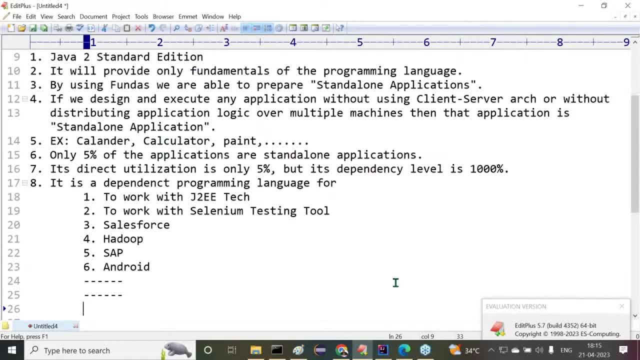 server architecture or not using client server architecture, not using client server architecture, without using client server architecture, without distributing application logic over multiple missions. if we design and execute any application on, if we design and execute any application, then that application is what their standalone application. can you tell me some examples? 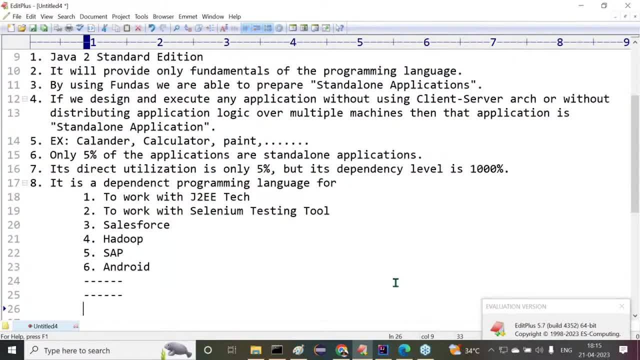 for standalone applications: no calculator, calendar page and so on. how many applications are standalone applications in outside? no five person is so jdse direct utilization is what five personnel? but it's the dependency level is what thousand person is? how can i say it's a thousand percent dependent programming language: how can you say it's a thousand percent dependent? 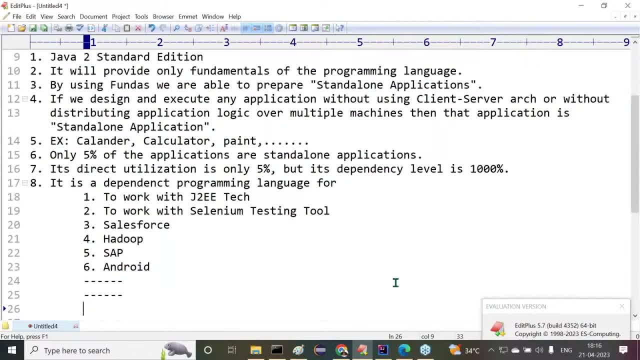 programming language. why? because it is required for working with the sales force, for working with the selenium testing, for working with the sap tools, for working with the jde applications. for all, almost 95 persons of the software products required what their j2se. because of that reason. 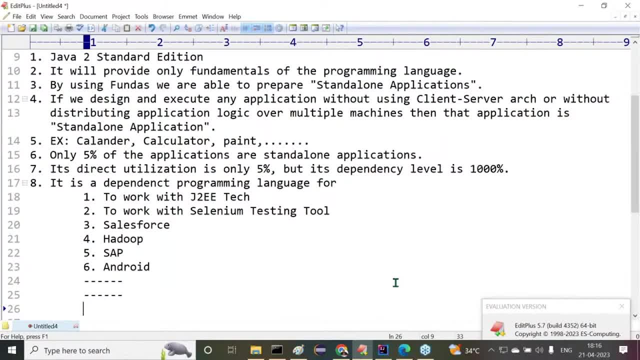 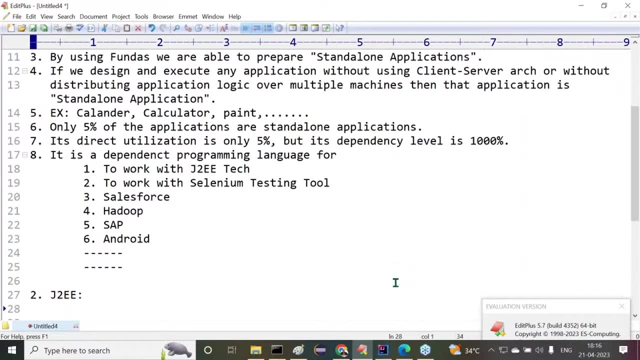 its dependency level is what their thousand person is, but its direct utilization is what their five person is. only all of you are clear, or not? can i move forward? can i go for the next one? you know? all right, what about this next one? get up so carefully, j2. ee. the next one is what there? 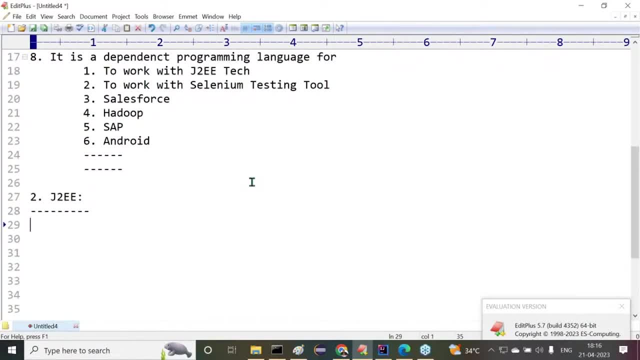 j2 ee. all right, sir, what is this j2 ee? actually, everybody put more concentration here. j2 ee is what i'm so carefully. first of all, abbreviation: what is this j2 ee? java 2 i, enterprise edition is it? what is the abbreviation j2 yes is what java 2 standard edition. j2 e is. 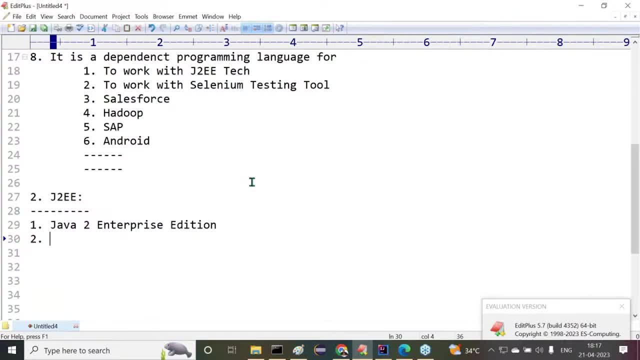 what java 2 enterprise edition clear. j2 se has provided fundamentals of the java. j2 se has provided what fundamentals of the java? but j2 ee will provide. j2 e will provide. j2 ee will provide server side programming. come on, j2 ee will provide. what side programming there? 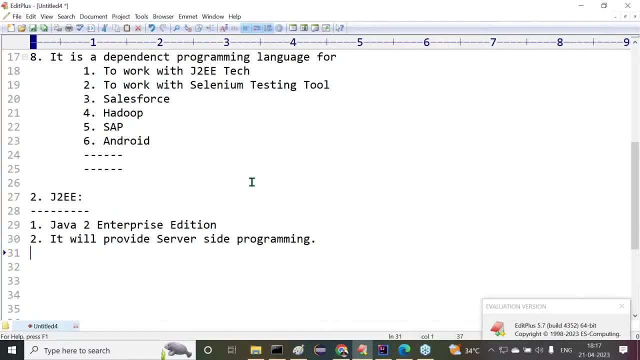 server side programming. server side programming in the sense client server architecture or not. it is using client server architecture or not. server side programming in the sense it is using client server architecture or not. all right, so next one point, number three: it will provide server-side programming. okay, by using j2se, by using j2se, by using j2se. what we prepared there, 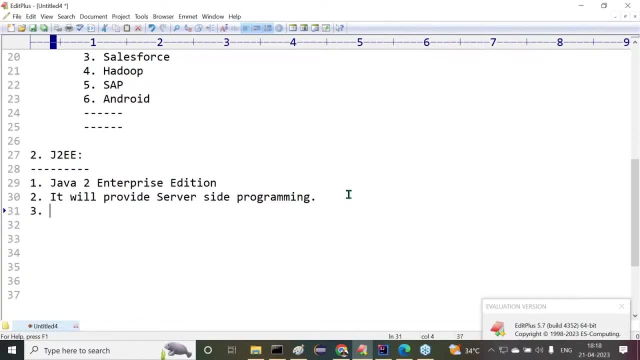 actually which type of applications we prepared there? standalone applications we prepared. that am i right or not? but by using j2ee. by using j2ee, it can be used to prepare. prepare what type of applications? no, enterprise applications are simply speaking distributed applications. by using j2e, what type of applications can we're able to prepare? 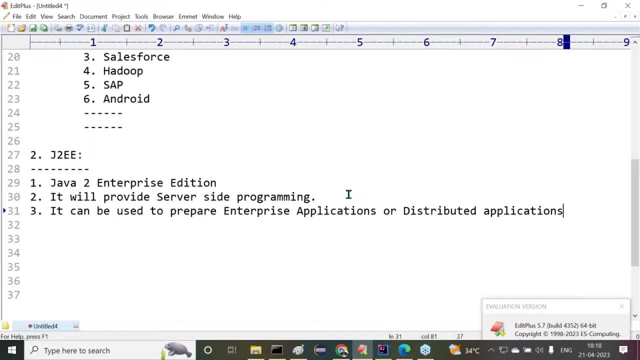 enterprise applications or we can prepare what their distributed applications. so all of you are getting my points, or not? enterprise applications are what they're: distributed application. now again, i have a question: what is this enterprise application? what is this distribute application? what's the meaning of it? right, the point is very clear. if we design and execute, 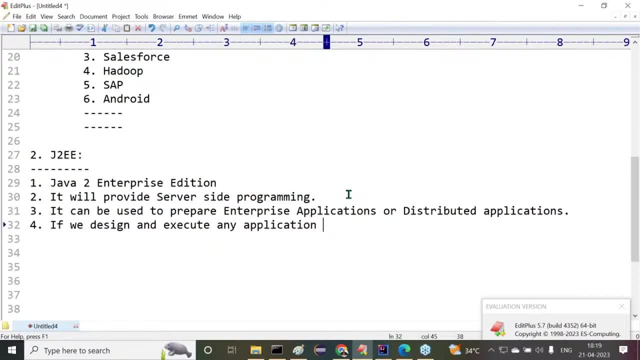 any application. quite opposite to standalone application, exactly opposite to standalone application. now tell me if we design and execute any application there without using client server architecture, but here, but here on the basis of? on the basis of what client server architecture are there without distributing application logic over multiple missions, but here what there? 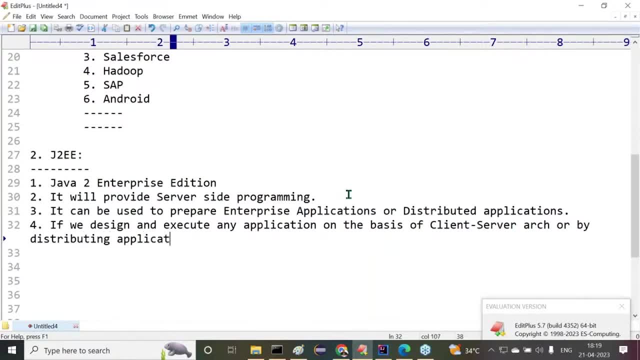 by distributing, by distributing application logic over multiple missions, then that application is called distributed application or what next one here are enterprise applications. don't worry, i'll share this document to you. just roughly. information, just roughly. i'm giving all the points here, but try to understand it now. 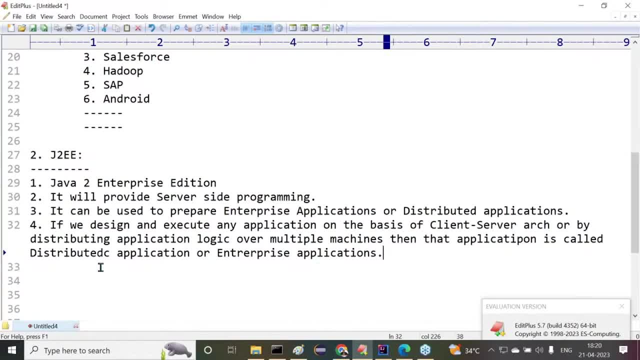 if we design and execute any application on the basis of client server architecture or by distributing application logic over multiple missions, then that application, then that application is called distributed application or enterprise application. that's it. this is what exactly the meaning of. like what they distribute application are an enterprise application. 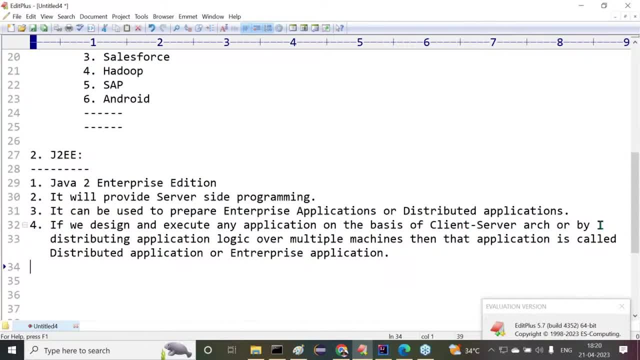 yes, all of you are getting clarity in this point. so that's okay, fine, but i have a question: how many applications are distributed applications? but i have a question: how many applications are distributed applications? right, if you want to see the diagrammatic representation, you know easily we can understand. 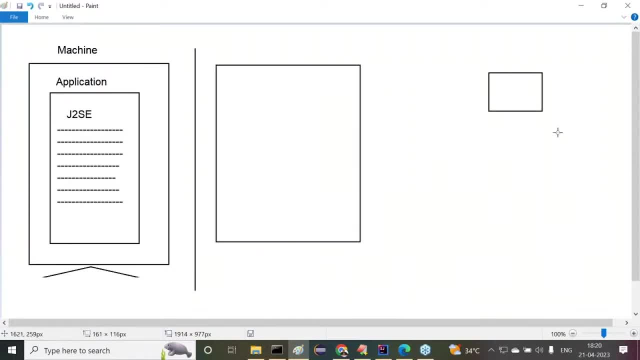 i'm so carefully now, this is one computer and this is another computer. all right, this is one computer. all right, so you can see. that is the screen. our net GPU is��. we gonna try to understand the video. actually, i have thought of something else. once again, wait for a minute next, etc. this will be an additional screen. 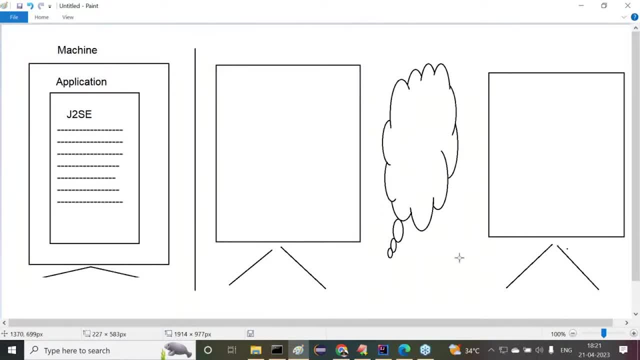 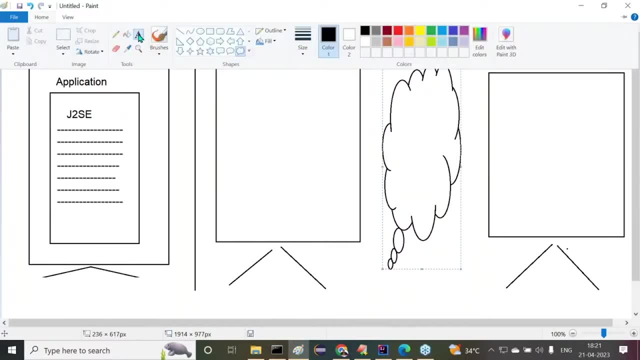 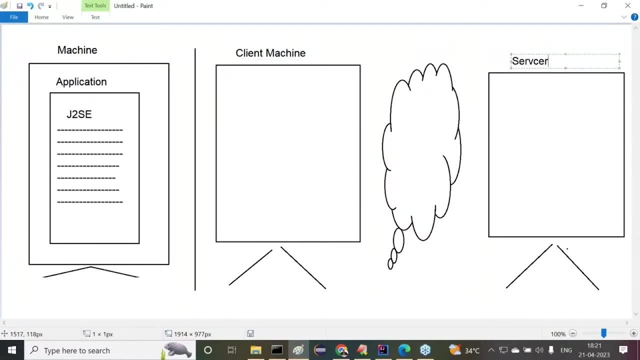 all right, sir, in between these two computers, what is required? network is required, am i right or not? network is required, protocol is required, communication point of you know. now this, i want to say client mission. now this, i want to say what their server mission. all right, sir, now again at the client mission. we are going to write a program. 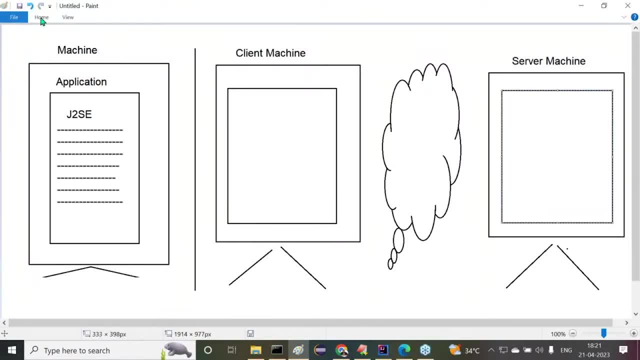 client application. at server mission we are going to write a program server side application. now, this is like what i'm telling their client application and this is like what i'm telling their server side application. i'll forget my pointer notch. all right, now this is like what their network. so here we have some coding parts at client program. we have some. 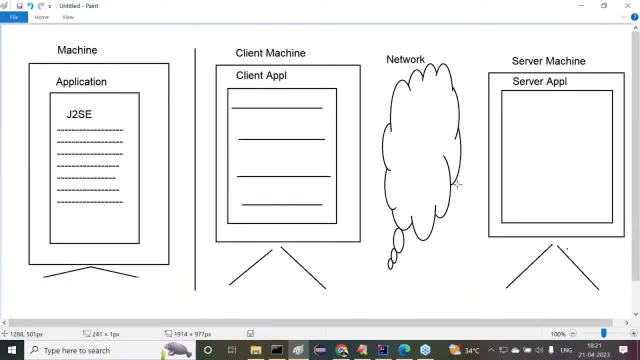 coding part here. these are the number of intersections. similarly, here also we are having what? their number of intersections. all right, then, first of all, what? what we are to understand here now. first of all, client will send request to the server, that is, to the network. then network will submit that request to what there, the respective server mission. 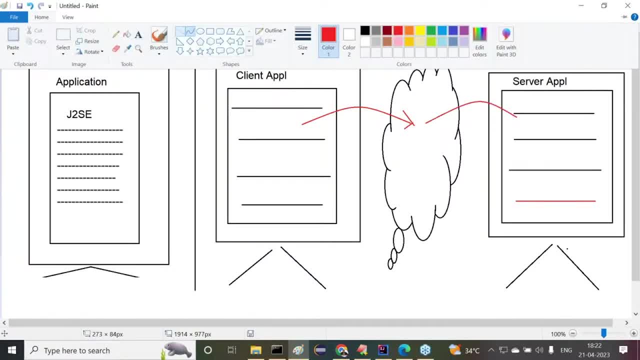 server side program will be executed. server side program will be executed when this program is executed. whenever this program is executed, automatically some response will be generated. that response will be given back to the network. the response will be given to given back to the network. so carefully, your network will send the required response back toward their respective clients. 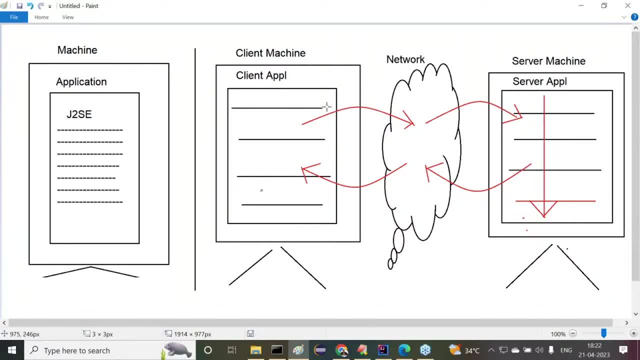 now tell me: application is designed on the base of client server architecture or not? application logic is distributed over multiple missions or not? come on, guys, so this type of application is called as what their distributed application. are an enterprise application, clear, okay, fine, this is okay fine. but how many applications are enterprise? 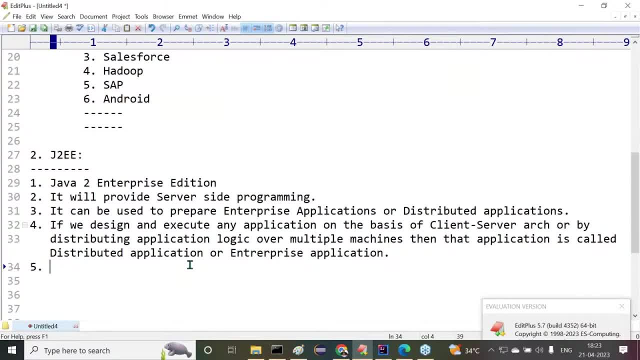 applications. how many applications are distributed applications? if you want to know that, now try to understand it clearly. 95% of the applications are distributed applications. 95% of the applications are what they're: distributed applications. any examples, any examples of all banking applications or distribute applications are not very good. then what next one? 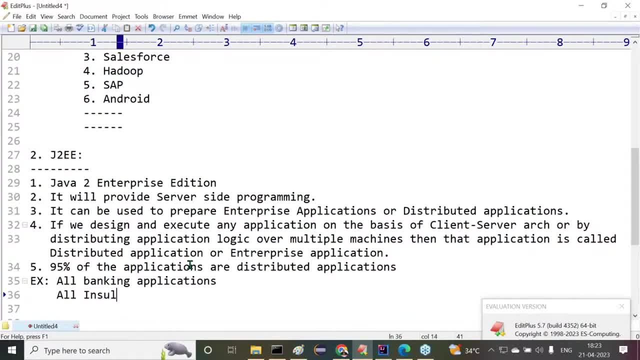 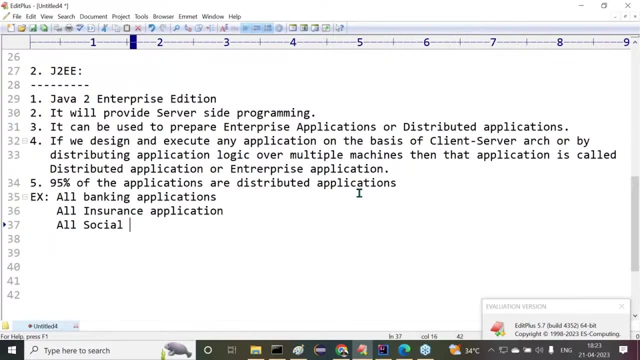 again offer this. know all insurance applications, Tata insurance application, maybe then by judge insurance, like so many insurance applications are available. all these are like what they're like. oh, next one is offer this all ok. social media applications. social network applications are what they're: directly distributed applications. now, i think very much you already aware about it. like what they're. 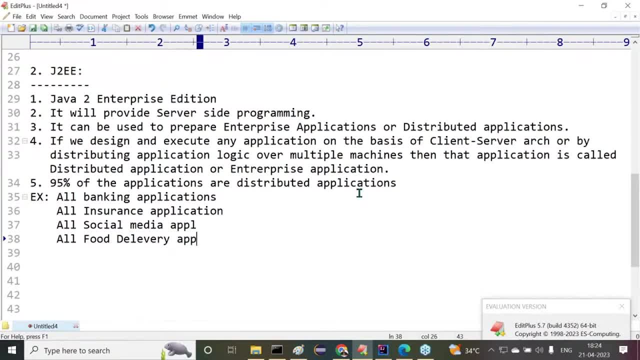 all food delivery applications, for delivery applications. now, all these are like swiggy jomoto. all these are what they're like, what they're distributed applications only. maybe whatsapp, maybe youtube, or maybe social media network or maybe social network applications. all these are like what they're distributed applications only right apart from this. 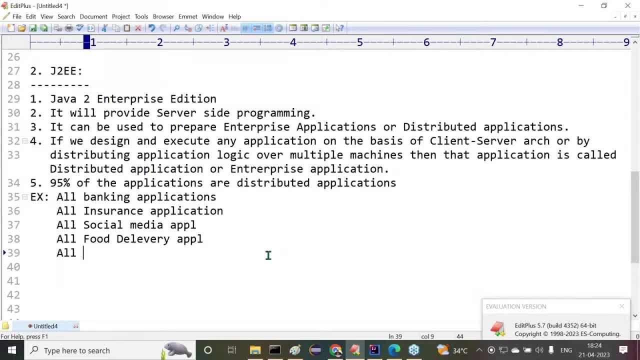 like this, so many, every domain. healthcare, all healthcare applications are what they're: distributed- applications only. all healthcare applications are what they're distributed applications only. take any apollo hospitals, maybe care hospitals, maybe they're where there's some applications are going on for the sake of tracing, for the sake of tracking patients, for the sake of 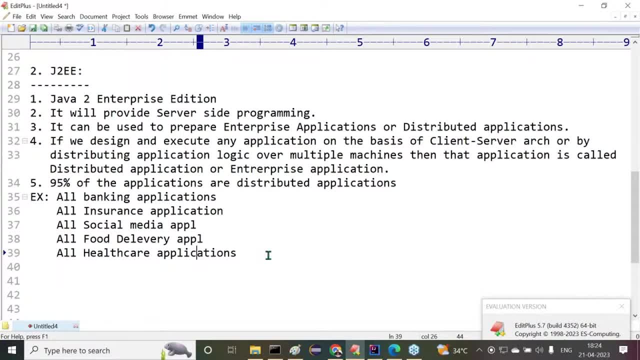 tracking doctors for the sake of tracking like what they're, then all these are like what they're- details now, prescriptions and everything. then there also be distributed applications are going to happen everywhere nowadays, everywhere, distributed applications are going to be happen. yes, clear to all of you know, right, sir? that's okay. fine, after completion of this 95 percent. 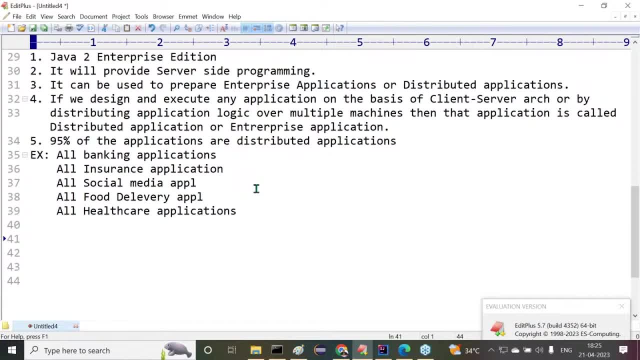 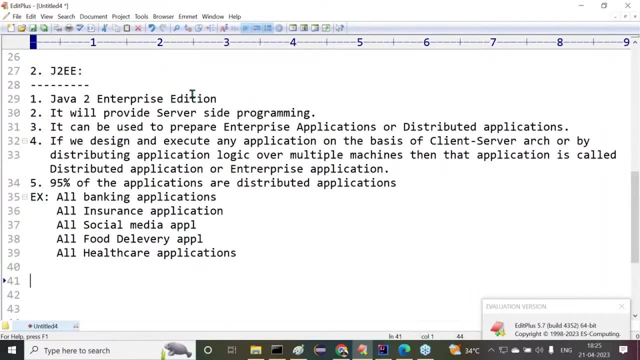 of the applications are what they're, distributed applications only. these are somewhat information about, like what they're. j2ee java meant for j2ee, not only j2sc java meant for what they're. j2ee java meant for enterprise application development clear. next, one third one. what about this third one again? now tell me. 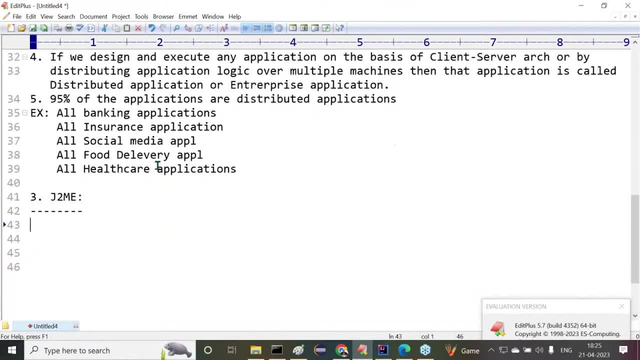 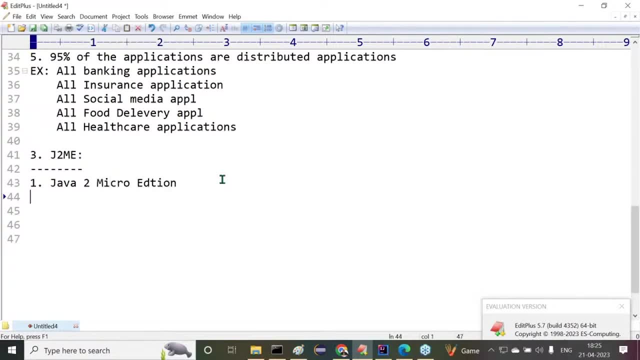 j2me java 2. now tell me what is abbreviation for it. no, java 2 micro edition, not mobile edition. please remember this. m is not, is not your mobile, m is what their micro. java 2 micro edition clear what it will provide. j2s is providing fundamentals of the java, j2e is providing server. 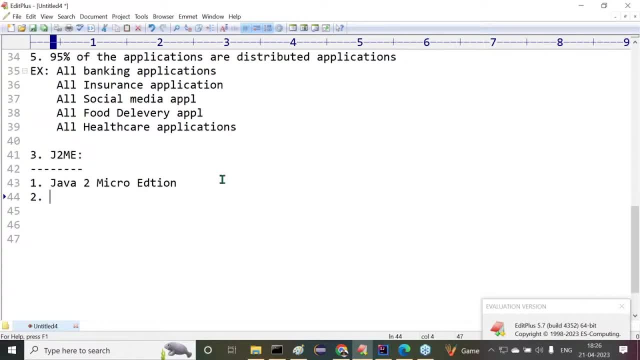 side programming. what is micro programming? what this jdm is providing there? it is able to provide micro programming, chip level programming, micro programming, chip level programming- okay, j2se. by using j2se, we are able to prepare standalone applications. by using j2ee, we are able to prepare enterprise. 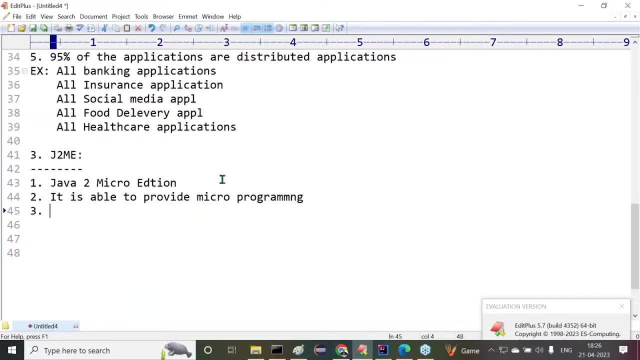 applications. similarly, by using j2me, what type of application scale we are able to prepare? no, by using j2me we are able to prepare. we are able to prepare, like a mobile based applications, simply speaking, mobile applications. how many applications are mobile applications nowadays in outside? 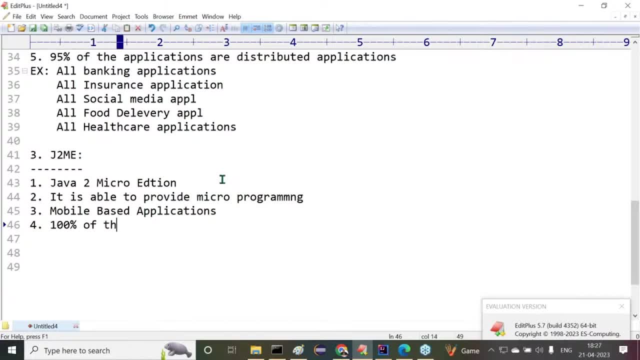 100 percent of the applications are what their mobile applications. am i right or not? 100 percent of the applications are what their mobile applications? clear, good, nice, then after this, out of after completion of this, 100 percent of the applications are what their mobile application. that's okay, we understood that. but remember one point. 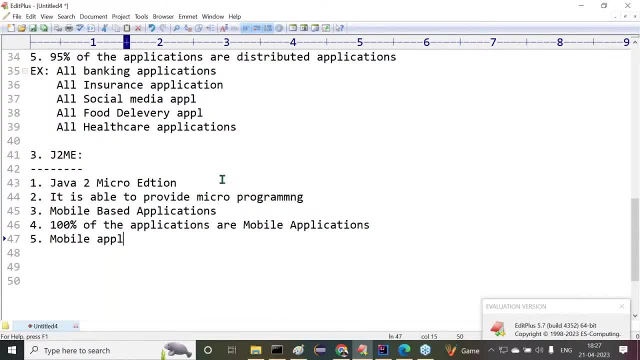 mobile application development has very good demand. mobile application development has very good demand in outside. why? because you could, if you take any domain, any location, mobile application development has very good demand in outside. why? because you could, if you take any domain, any location. mobile application development, mobile application support is. 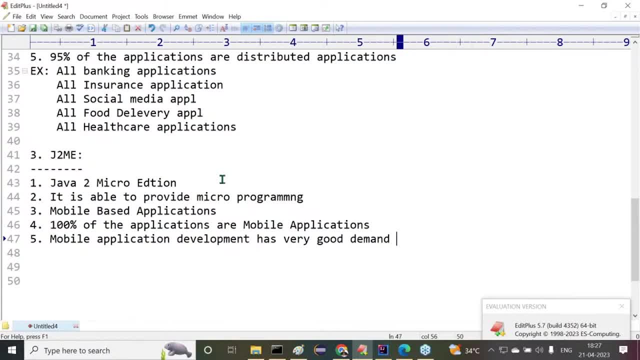 mobile application development. mobile application support is mobile application development. mobile application support is available. available. available. go for hospitals: mobile application. go for hospitals: mobile application. go for hospitals: mobile application development. mobile application support is development. mobile application support is development. mobile application support is available. go for banks: no. 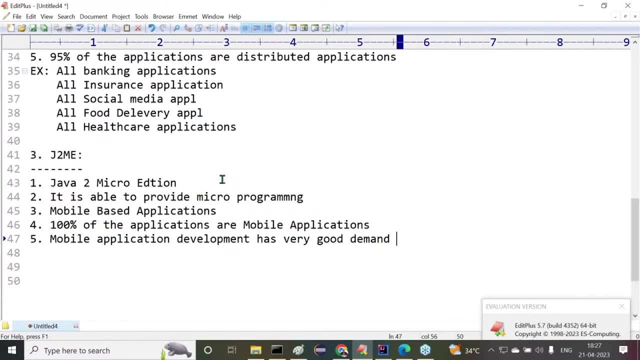 available. go for banks: no available. go for banks: no mobile application: see, for example. i have mobile application. see, for example. i have mobile application. see, for example: i have an icsa bank account, an icsa bank account, an icsa bank account. imobile app is available. 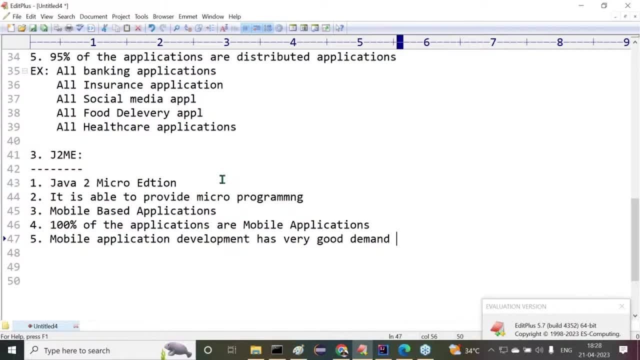 imobile app is available. imobile app is available. am i right or not for the sake of for? am i right or not for the sake of for? am i right or not for the sake of? for example i have, might be what there. example i have might be what there. 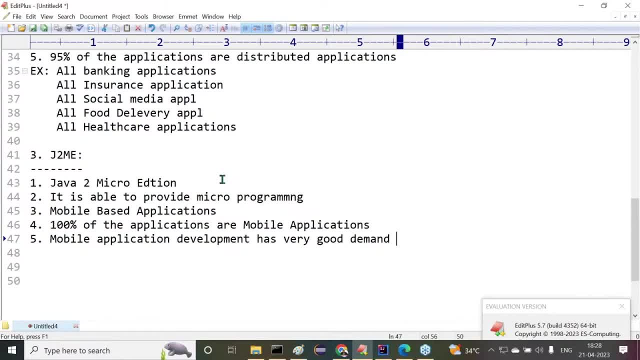 uh, airtel. i have a sim sim card that means communication communicator, airtel communication. i'm using them for the sake of airtel payments and all these things. now my airtel app is available. my idea, my vodafone app, hdmi bank application, whatsapp mobile application. 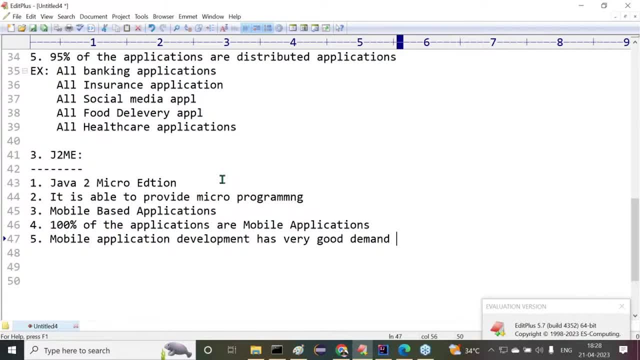 youtube. i'm going to see all videos through youtube. if i want to see all videos through youtube, in the sense, what we have to do, we need to install that, app or not, youtube app or not. of course, by default it is coming along with our mobile phones now. but if it is not available, we 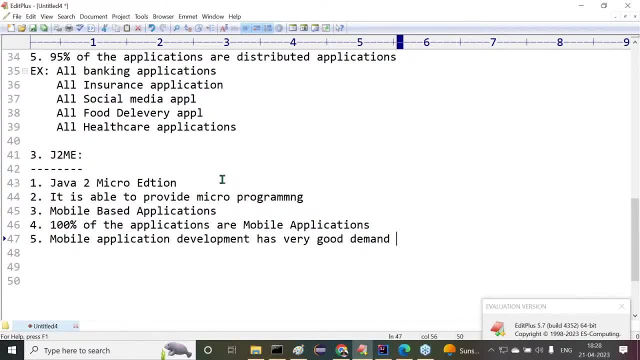 are able to install it or not. facebook: i want to watch facebook. i want to see. i have to install that facebook app or not? i was carefully speaking. all these things: i have to install my mobile phone or not? all these are what their mobile applications are nowadays, in every sector: mobile application. 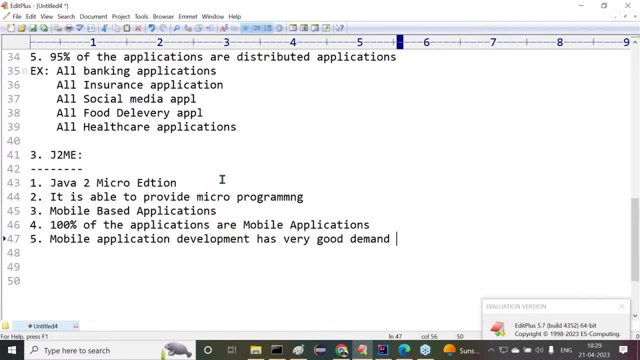 development is available. so that's why 100 of the applications are what their mobile applications only. but understand my point here. fifth point is important now try to understand it. no, mobile application developer has very good demand but but no demand is available for no demand is available for j2me. it's almost all dead in outside. 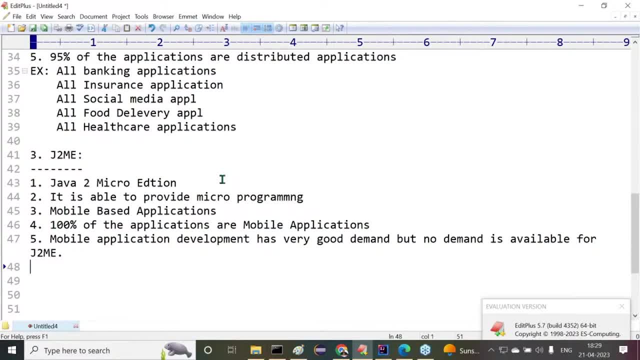 not available. no demand is available for j2me when the alternatives are coming into the picture, when android application development, when android is available in outside of the market, when android was introduced, when iphone technologies are introduced, automatically demand was reduced. demand was fall down. for what their 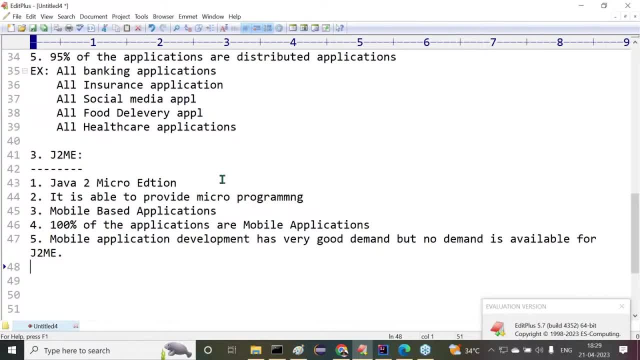 no demand is available for jdmb nowadays. why? because number of alternatives are available for mobile application development. that's why nobody is thinking about j2me. watch i'll if you're getting my point or not. so this is a clear-cut information care i'm telling there. 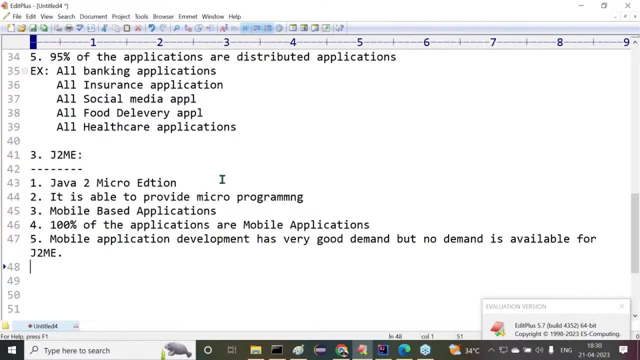 about all the content here. we have to understand them, right, sir? finally, now tell me, all of you, now tell me, java is available in how many parts? no, three parts. what are the three parts? no, j2se. then what next one can offer this? no, j2ee. third one: is what there? j2me. 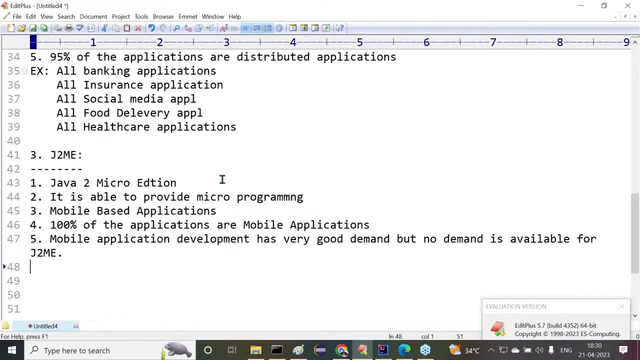 m e. out of all the three things now, which one is very good: j2 s e and j2 e e. if you want to learn j2 e e, we require what j2s, so we have to understand both. nobody is thinking about what j2. 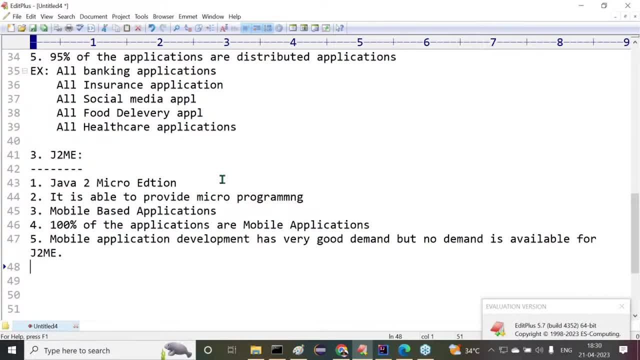 m e being the java developer. if you want to become as a java developer, your target is very clear: j2 s e and j2 e e. that we have to learn. is that all forgetting it, or not? okay, leave this one all right now. just a few minutes of time. a few minutes of time just. i want to discuss about like. 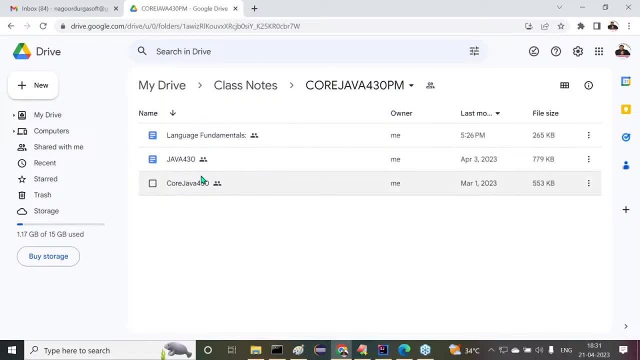 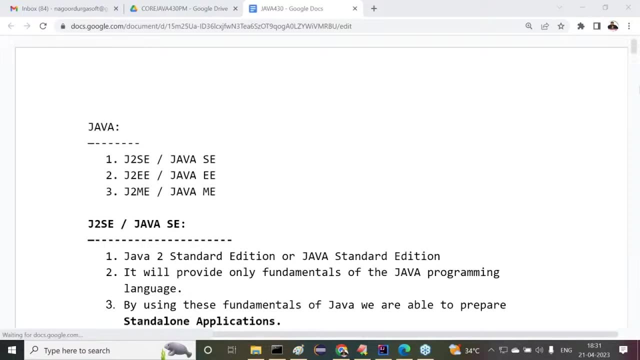 what there, what exactly the content here i'm going to discuss with you, what exactly my plan of discussing all the content here just two minutes of time. i want to give some clarity. of course, already the document i created here, what are the content i discussed today also? 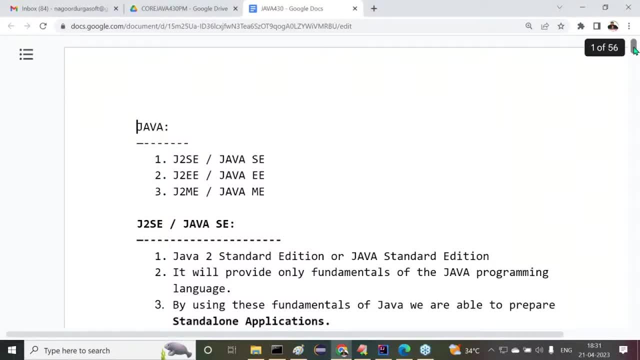 i'll share this document to you, okay, but not immediately, right? i? i need to take one more class there. in that, one more class there, i'm going to share all the resources and on on what, what exactly the content i want to provide there, everything i'm going to provide to you. 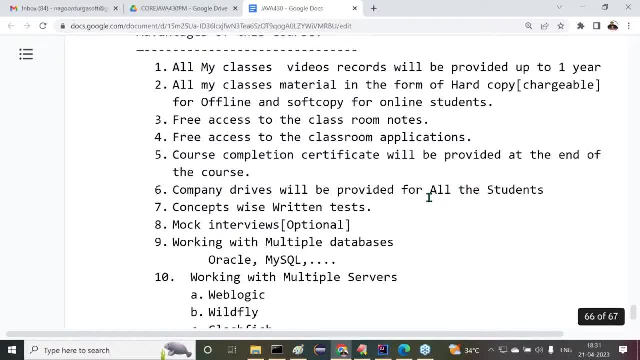 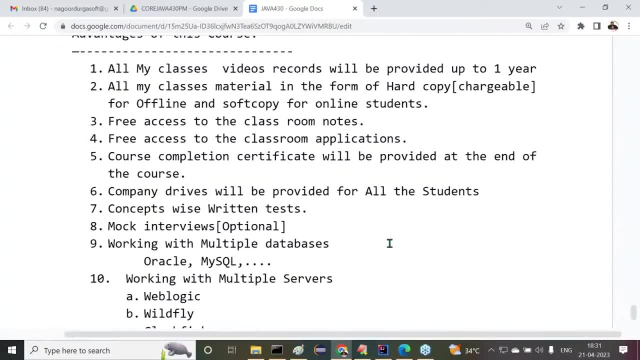 but before that, now let us have some clarity. all right, sir, mainly i'm going to provide this clarity: if we join with my classes, if you want to join with my classes, what advantages we are able to get everybody understand it clearly. you know, all my classes are recording record might be being recorded here every class. now. 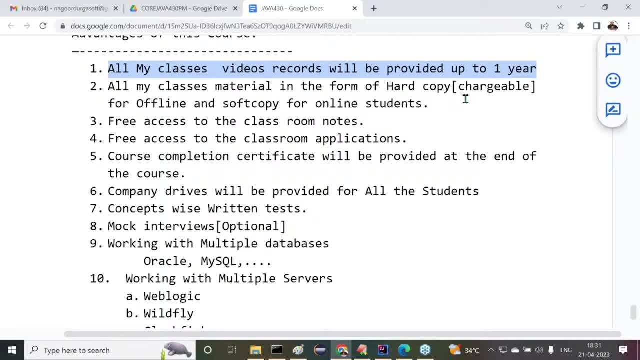 recorded videos will be provided for everybody up to one year of time after completion of the course. one year of time, not right from today. that means what is the meaning of it? no, every class regarding will be shared to you. even today's classes also share it within one hour after completion of the. 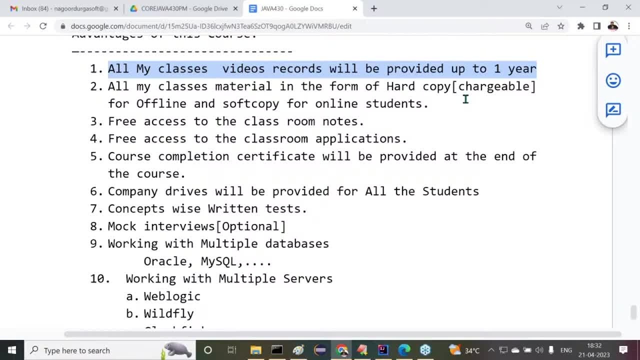 class. that recording will be shared with everybody, so it's going to be available up to one year of time to you. that one year of time we can calculate after completion of the course, but right from today onwards, videos are. videos are going to be available for everybody. 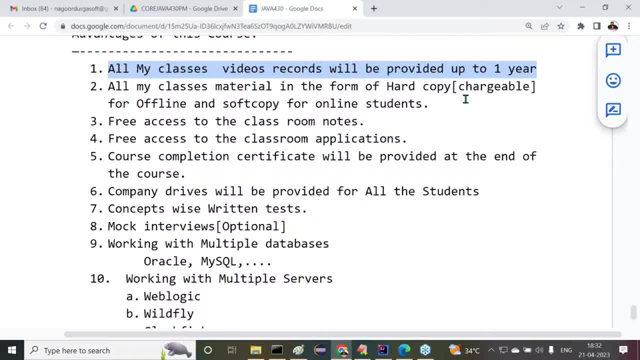 observe carefully. this is very good support, what durga shop is providing at present. other institutes are not providing this much of support. but because of this, giving this much of support, why? because multiple advantages are available by sharing this. recorded videos. yes, sir, all of you are getting it. what i'm telling you is a backup, completely back up, if you want to. 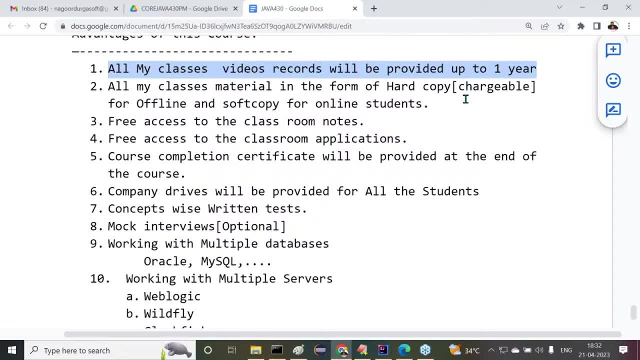 watch again the same class, no need to wait for other batch. now, directly on the on the same day, open that video and try to watch the content. that's my point here. if you are unable to start adiabat, if you want to go outside there, yes, videos are available within one hour. we are able to see. 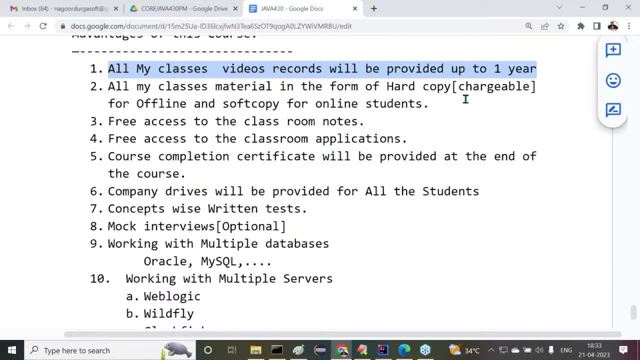 that video support. we're able to get each alifare getting it or not. okay, fine, all my classes materials are available in the form of soft copy and if you want to get hard copy, some charges are going to be happen, just so you can check it at our office there, but soft copy will be provided for everybody. 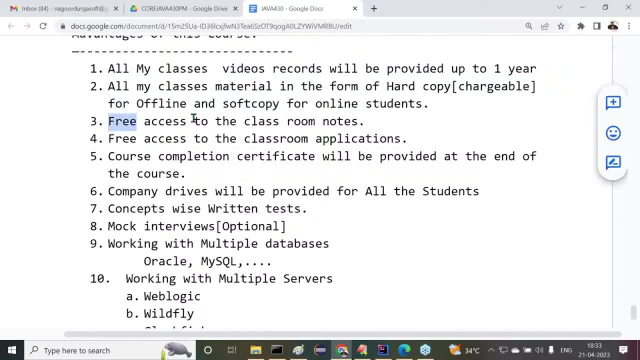 okay, right, sir. free access to the classroom notes. whatever the notes i'm typing there, everything i will share with you, no need to worry for it. free access to the classroom applications. whatever the programs i'm going to provide, everything i will show live applications in front of you. i will type everything, even notes also, i'm going to type in front of you. 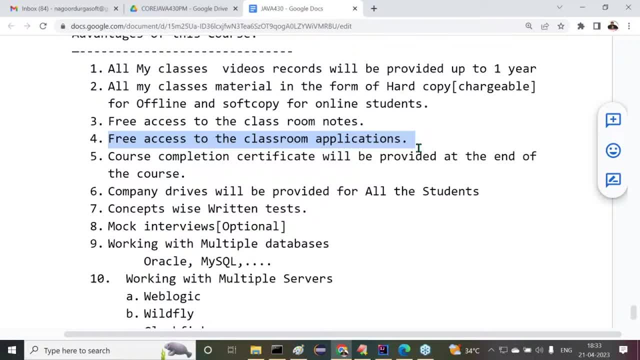 now today how i'm going to type the content while explaining the concept. i'm able to type the content here. multiple tasks i can do at a time here. i don't have any problem there. that notes i'm able to share with you. okay, all right, sir. course completion certificate. 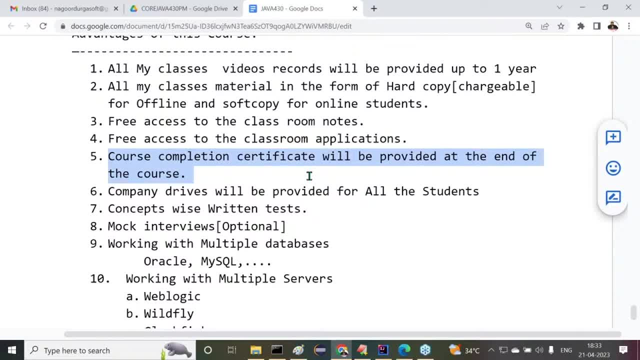 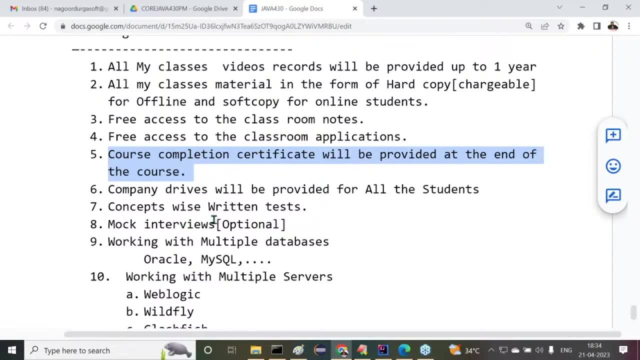 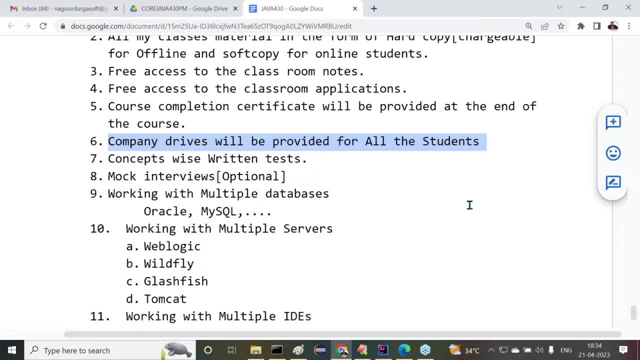 will be provided at the end of the course. you can utilize the durga soft brand also in our search. definitely some waiters will come to your resume. next one is: yeah, this is important, durga soft is providing company drives, company dress, but, depending on the situation, all right, we have some clients with us. 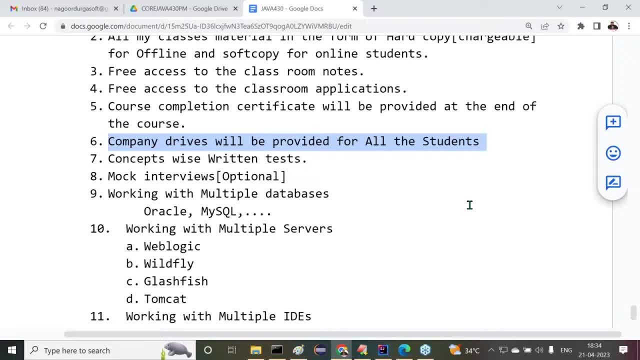 i'm going to get their companies there, then company drives are going to be connected. understand my point, what i'm telling you? so this is not like any job guarantee kind of program there. this is clearly technology based program, content guarantee, not job guarantee content guarantee. if you understand my total content, getting job is nothing, very simple. 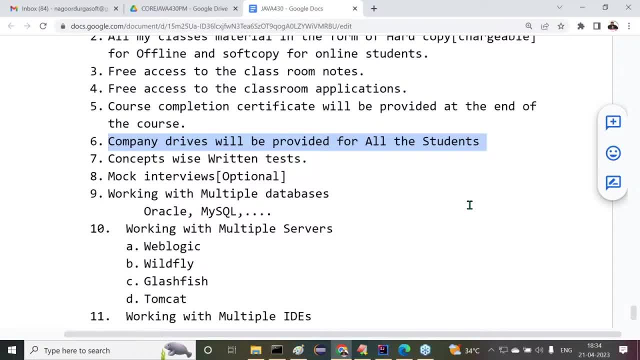 in my classes. 80 percent is a success rate, definitely 80 percent is a success rate. for every 100 members, 80 members are going to get jobs. sure, but one month before that i'm going to get the job, or i'm going to do one month later, before or one month later, okay. 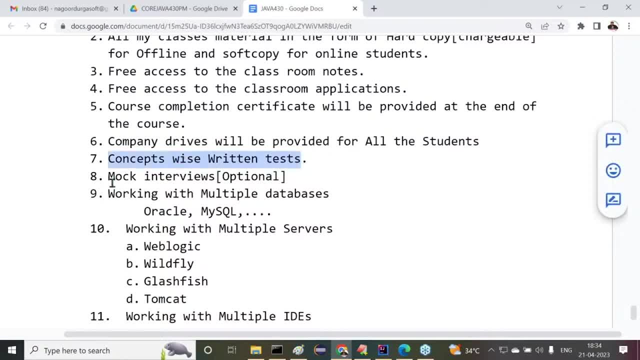 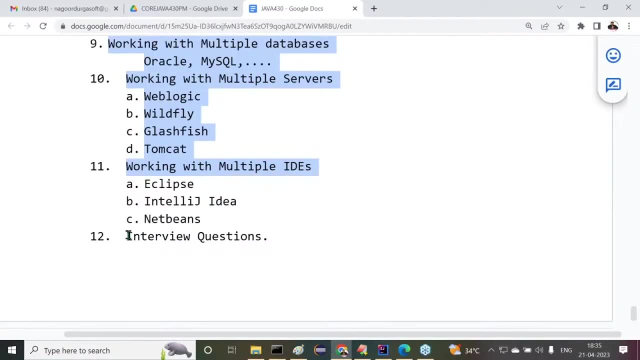 leave it now. concepts. wise written test we are going to be conducted on every topic. if it is possible, i'm able to plan for what their mark. interviews, okay. working with multiple database: okay. these are the technology related things. no, by moving on to the concepts, we are able to understand it clearly. no need to worry for it, right, sir? part of the notes. 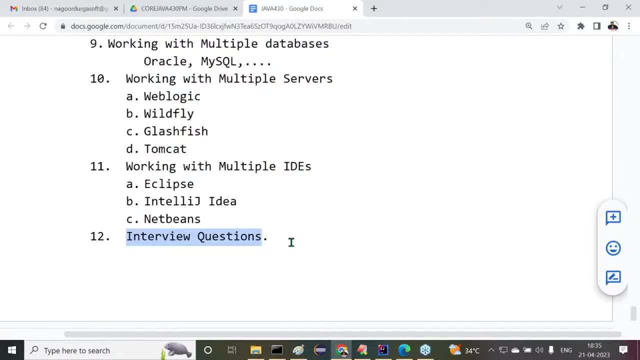 itself. i'm going to include interview questions also question and answer format. we are able to get it. so there's multiple advantages scale. we are able to get. that's okay. all right, so do the actual test there. these are the techniques available here. okay for advanced courses before. 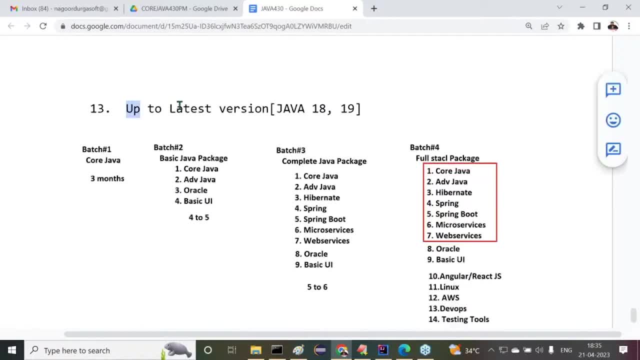 and there are also training and materials available, so it is very suitable for not having okay coming to the okay. the next one is one more thing here, which version i am going to discuss. what is the latest version of the java? at present latest version of the java is: what is the 19? 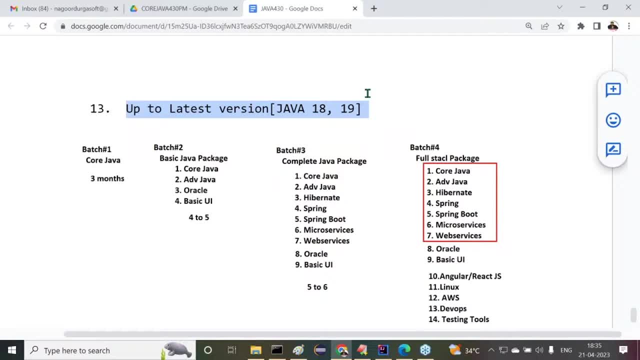 20 is coming now. okay, i didn't check it last 10 days of time. i was totally off actually. so if 20 is available, i'll discuss about 20 also, don't worry for it, it's a matter of one day to update myself, right? what features are available? new features inside the 20? i'll discuss with you. 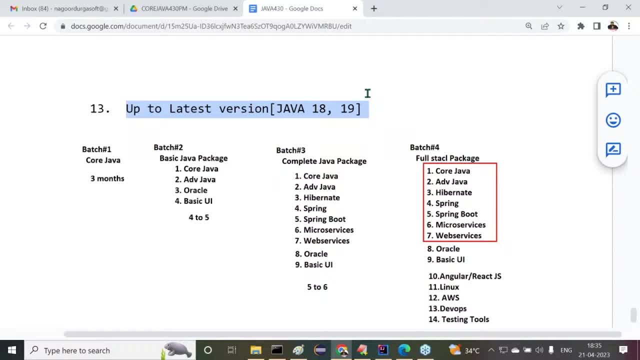 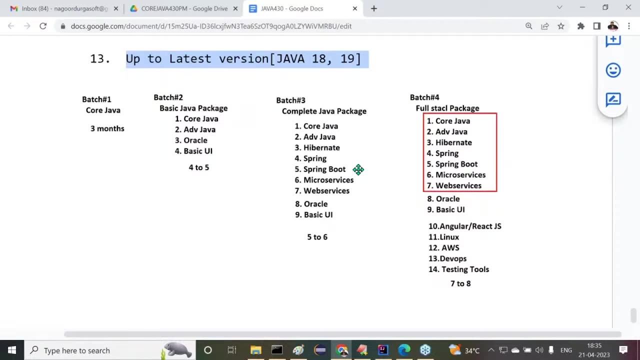 but at the end of the course, not immediately up to the latest version. up to what? their latest version, right from starting point to ending point. anyone is what their latest version? okay, all right. so today, what batches we are offering from durga's option today is a general. 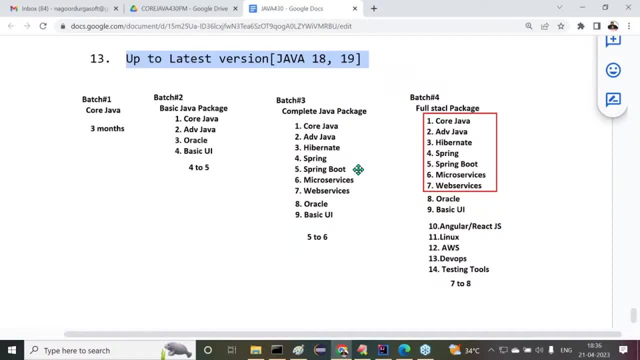 demo class i am conducting here. this is a demo for these multiple batches. only core java: if you want to learn, we can come for this. bachelor is a basic java. core java: advantage of oracle and basic ui. batch 3. complete java package. core advanced hypernet. spring spring about micro services. 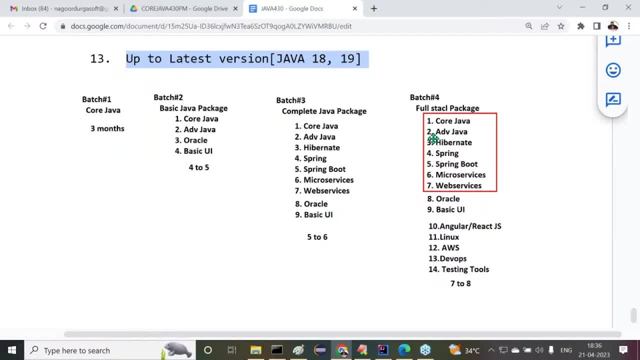 web services are agile and basic ui. next one is what their full stack java, core java, advanced java, hybrid, spring, springboard, microservices, web services, oracle, basic ui, angular or react, linux, aws, devops and testing tools- this is full stack java. nowadays, this is a trending in our search. 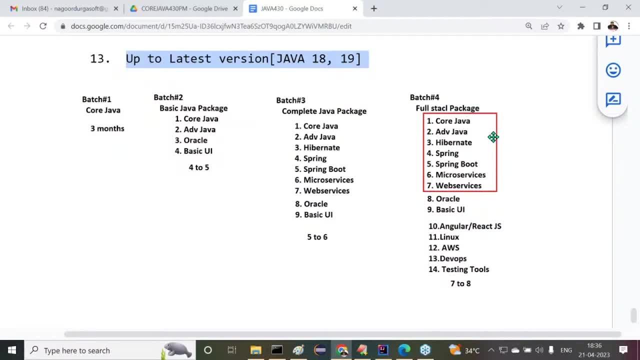 every company is looking for watch. every company is looking for full stack java developers only. nowadays, every company is looking for what? their full stack java developers only. but these packages we provided names like: no, but this is main package. everybody is looking for it. understand it what i'm. 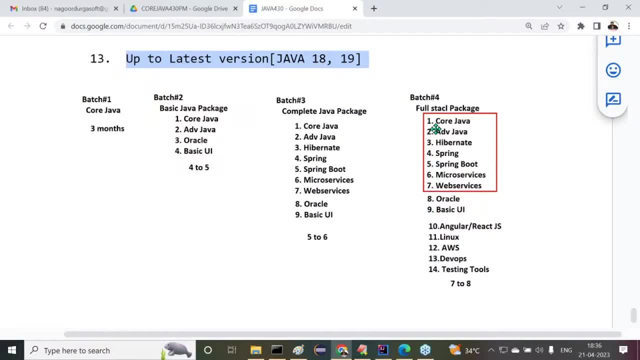 telling them. but after completion of this course, everybody you are able to get full stack java total content. nearly 60 pages document is available in a 60 pages document. the total syllabus are included there so you are able to get that 60 pages document through your whatsapp after completion. 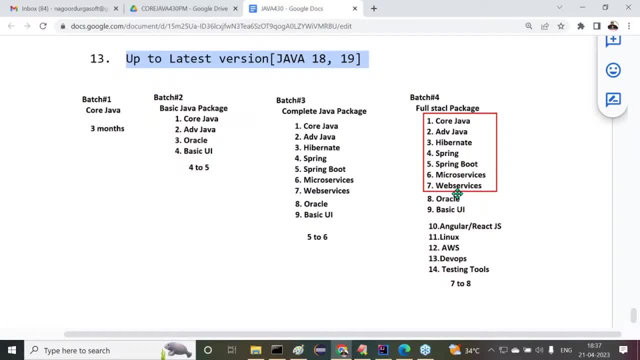 of this class. our admin people will send the document to you. there we can see the total syllabus. whatever the syllabus i am going to discuss inside the classroom, the total syllabus you are able to catch. okay, in full strike, java. what is my participation in full strike java? what is my? 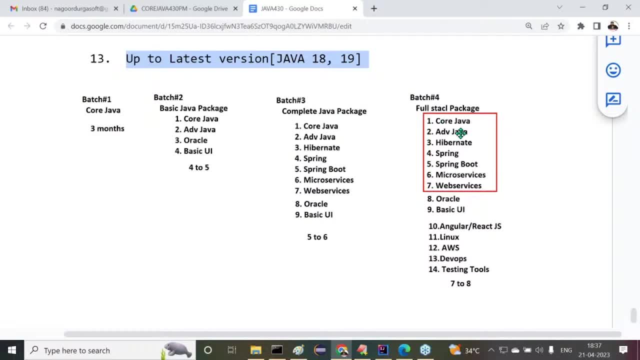 participation. if you have to this, this red color symbol, this total red color box, up to total java, java related: i will take the responsibility. remaining non-java related things are available. remaining part: some other trainers will take that control. some other trainers will take that control, but my part is what they're. this total: almost all 70 to 80 percent of the full stack java i will cover. 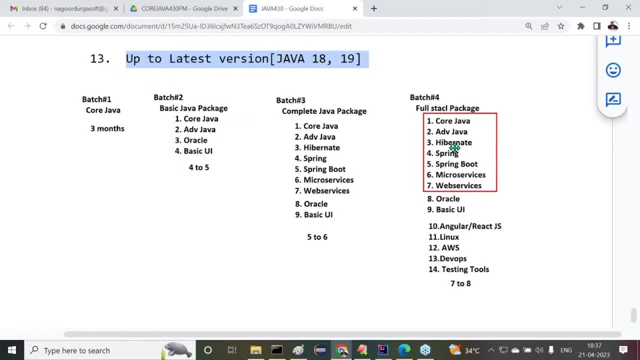 that java is the main content and my things are what they're sideways technologies, but they're also important for us. we have to land it. some expert trainers will take that content here, but these things here i'm going to take, you know, is that, if you're getting it or not, what i'm 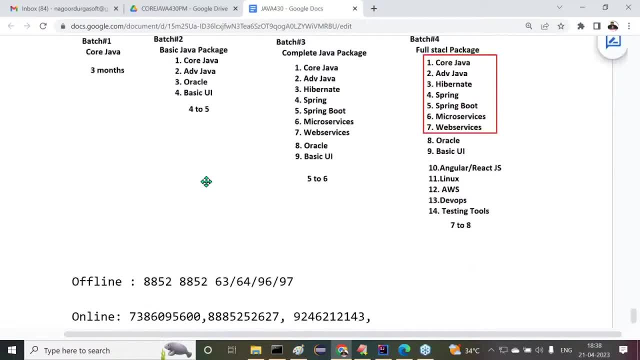 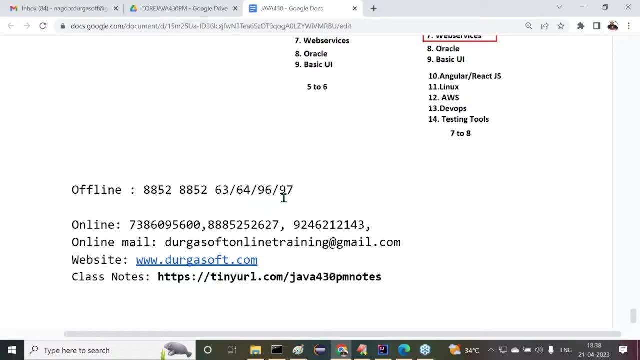 telling you: okay, all right. so now then, um, all right regarding this remaining further details, okay, we'll just click here. so the content will be for you to add our values to. but what i'm telling you for the java, we can only combine. the هنا, we can Manipulate at the end of the course. 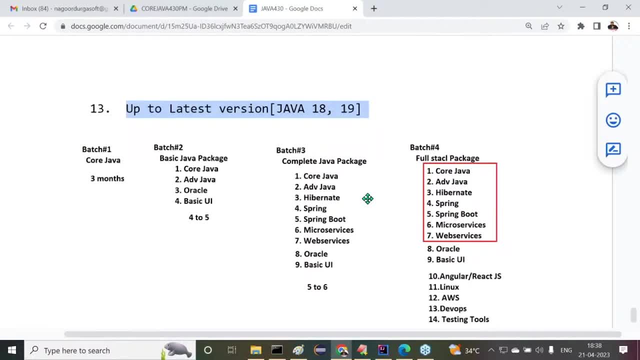 across all these colleges, even for different classes. only we are ceramics in card. what we also have other features. we can fix the quality. we can tomato sort the J filming. consider any position to teach java to somebody else. getting job is nothing you can play with interviewer. so i will increase confidence, i'll inject more content. that is my main philosophy. 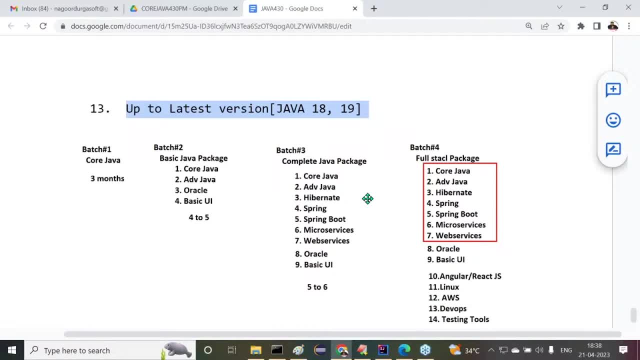 see the shortcut way to get job in the sense, everywhere it is available. just we can go for it. if you want to get job in a shortcut way, no need to come to turkish option. really, if you want to learn subject, then come to me, then come to my classes. 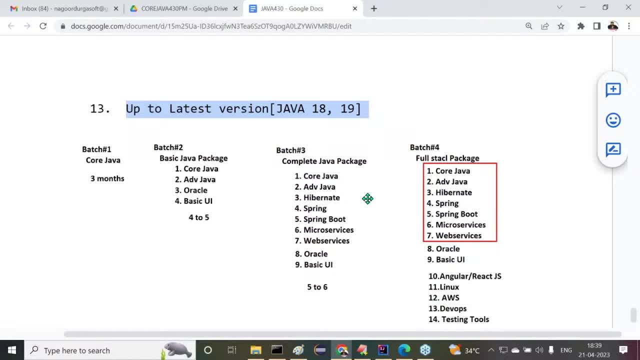 so it's totally subject based, totally content based. i'm going to improve your subject level. that's my actual target. if you are subject full, if you are contentful, getting job is nothing. at any location, you can survive. that is a simple philosophy here. what i'm telling you to know. 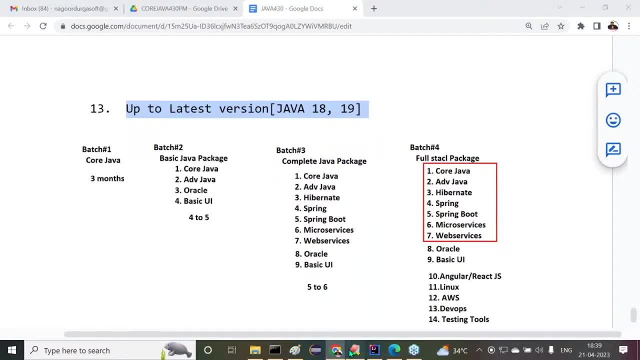 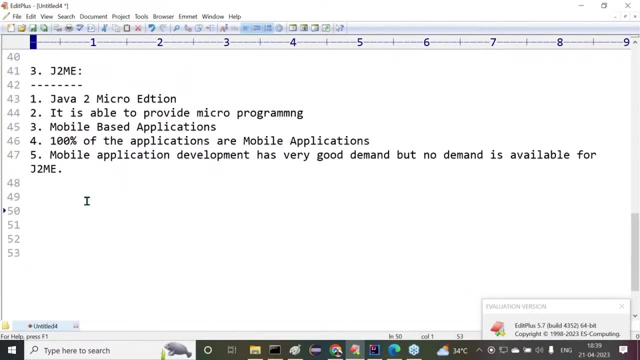 okay, all right, sir, this is one thing. and, uh, lastly, one simple point here. i'm telling you, observe carefully, all of you guys understand it. no, today is one demo class- i i discussed it here- but tomorrow actually i need to take this session. no, but tomorrow is a festival, i think so right. 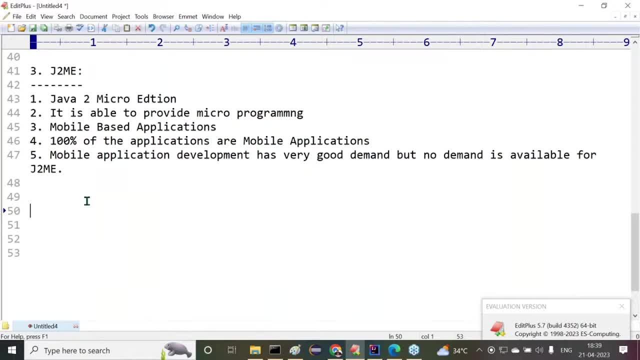 even myself also, i'm not going to be available there then tomorrow i'm not going to take the class there. sunday- anyway, half sunday- is also not available. next class will be on monday. next class will be on monday. at what time we have to come there? next class: no, on monday 5: 30 we have to come. 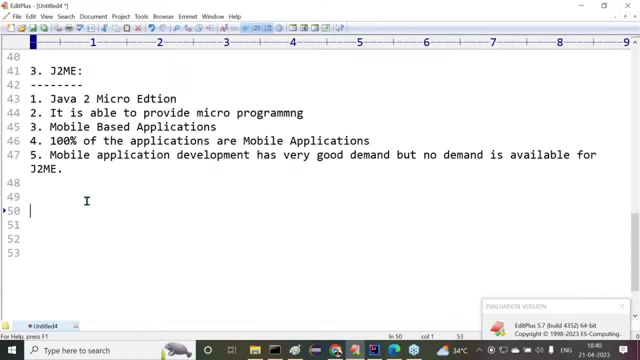 there. please remember this: at 5: 30 we have to come next class. please remember this. after few days of time, after few days of time, i want to take your classes right from 4- 30, not only 5: 30. please remember this. after a few days of time, i'm going to conduct your classes right from what 4- 30. understand guys what? 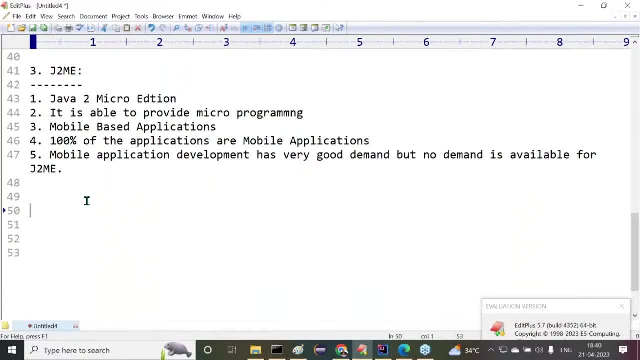 i'm telling a few days of demo. i'm going to take your class at 5: 30 why? because that uh schedule is not available. actually, i need to start our class at 4: 30, but schedule is not available. after a few days of time i will start our classes from what they're: 4: 30, 4 30 to 6. i'm going to take it. 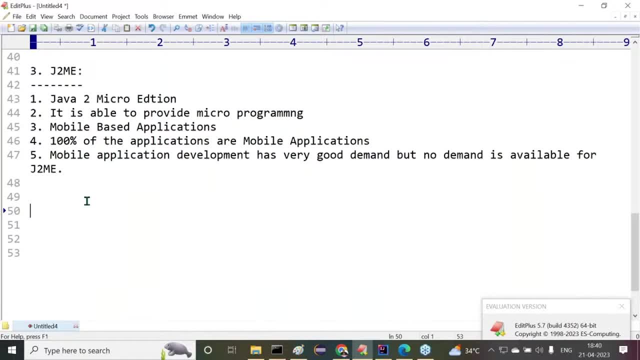 remaining classes: full stack job. if you take no evening starts you can assign to me. regarding this: java: total java- remaining time we can attend for other courses in full stack java: up to seven courses. i'm going to take remaining courses you have to take now. in the remaining time we can. 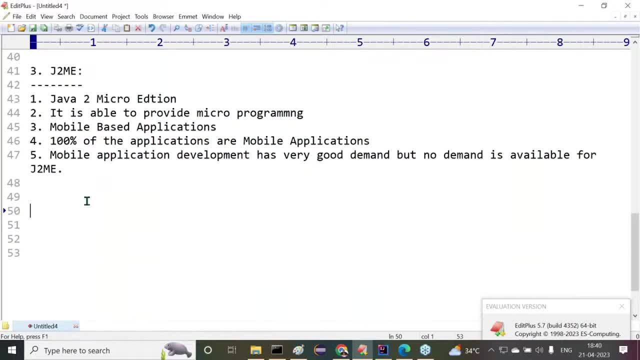 take that courses, though, but up to full stack java, up to java stream i'm going to take at evening time only. i'll give the time to time schedules to you, no need to worry for it. so all if you're getting clarity or not, okay, almost alone. the time is 6: 41. at 6: 30 i have to start other classes. 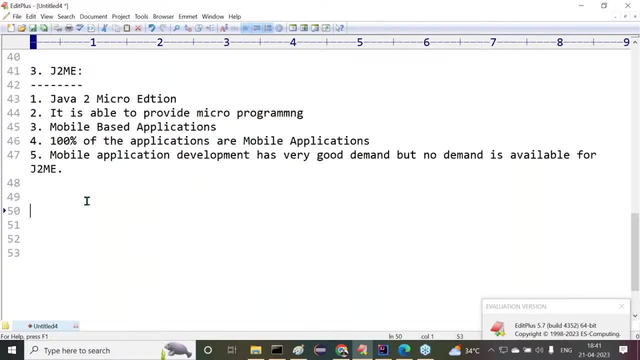 students are waiting in outside now. so on monday i'm going to take your class there few days of time, 5, 30 to 6: 30 only. but after that i'm going to take your classes. from what time? they're not 4: 30, 4, 32, 6 o'clock. i'm going to take your classes here itself. i'm giving confirmation for it, okay. 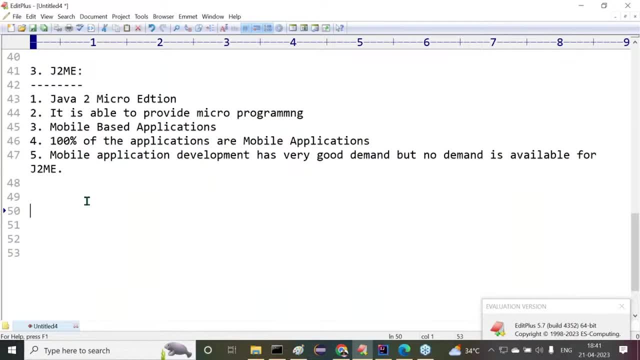 shall we meet on monday, right, sir? thank you, thanks a lot for attending this demo. we'll meet on monday. monday at 5: 30 only. monday at 5: 30 only. after that i'll give information to you on which date onwards you have to come: at 4: 30.. monday at 5: 30 only. we have to. 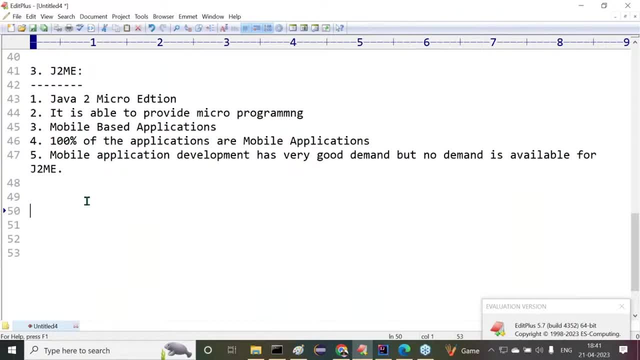 come. thank you, thanks a lot. we'll meet on monday, oh guys. uh, those are attending in online there then already time is completed. uh, don't worry, then on monday i will put some time for you for the sake of your daughter's clarification, if you have any doubt. 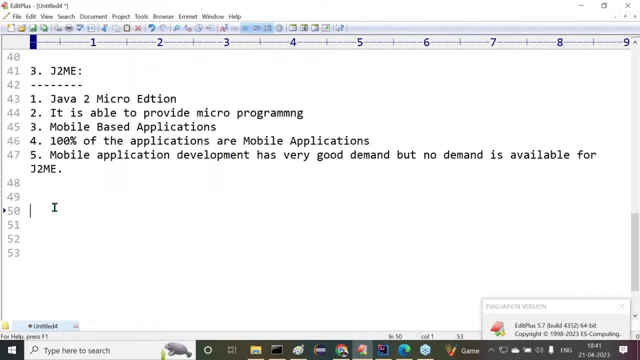 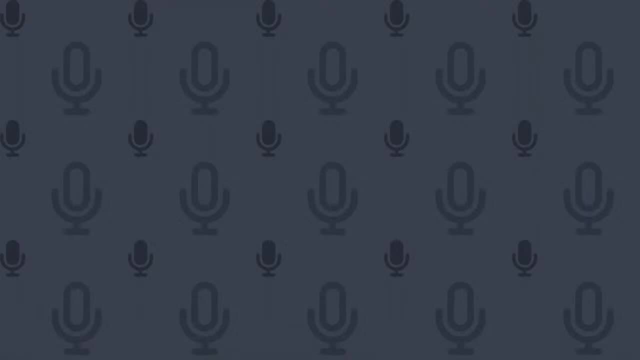 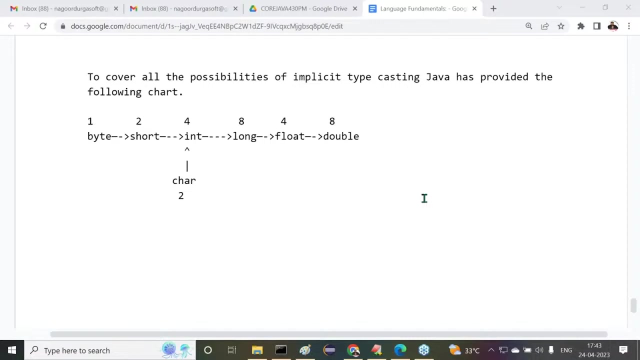 then definitely, i'll clarify it on monday, okay, thank you. thanks so much. please confirm to me all of you get my voice on screen. those who are attending in online. guys, please check it. all of you get my voice on the screen, guys. please confirm to me all of you get my voice on screen. those who are attending in online. 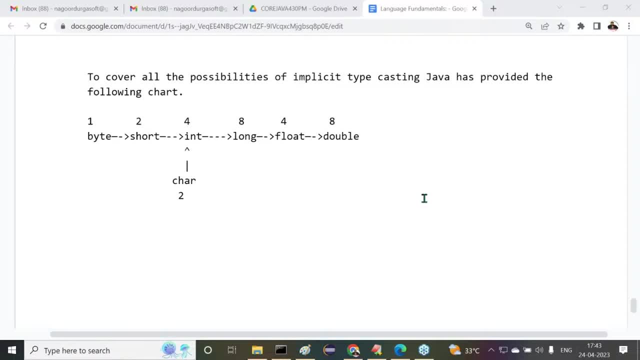 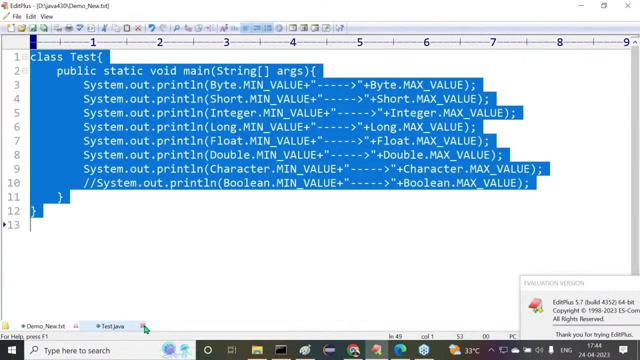 okay, guys, please confirm to me. all of you get my voice on screen. guys, everybody, please respond for me, all of your, get my voice and screen you. yes, right, thank you, thank you, thank you, All right, good morning, guys, and this on Friday, I think. so I have taken one demo class. 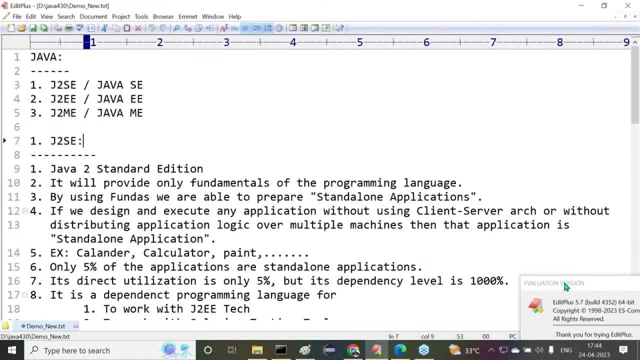 The continuation part here. we have to discuss that anyway. So let us check the content. what I discussed it there on the Friday class. See this: Java is available in how many parts there come on: Java is available in how many parts, three parts. What are the three parts there? J2SE, J2EE and J2MEE. J2SE is providing only fundamentals. 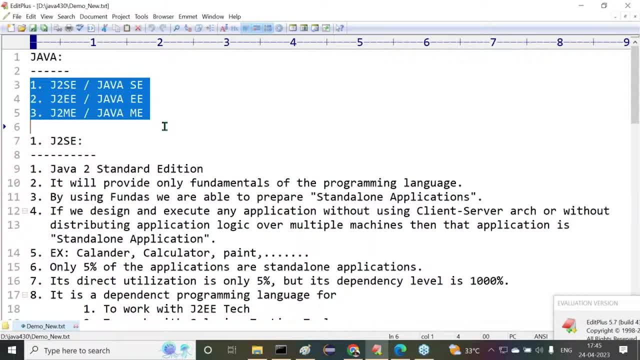 of the Java, by using fundamentals, were able to prepare standalone applications. Standalone application are like: what calendar in our computer, calculator in our computer like this: how many applications are standalone applications? there, only 5% of the applications are what their standalone application. what is standalone application if you have to this? 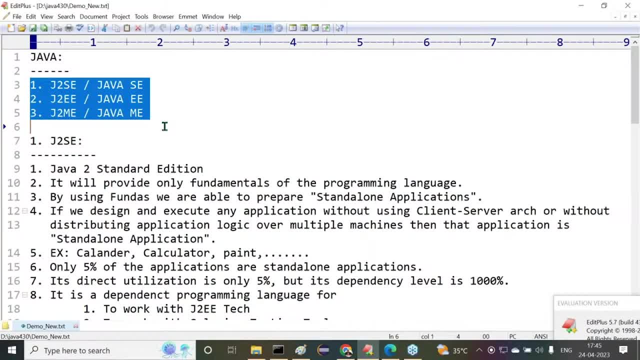 if we prepare and execute any Java application without using client-server architecture or without distributing application logic over multiple missions, then that application is what? standalone application? all right, sir, it's a direct utilization is only 5%, but it's a dependency level. 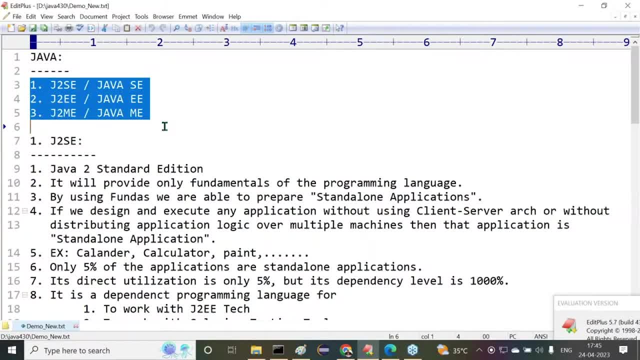 It is what that thousand person is: to learn J2EE, to work with the J2EE applications, to work with the selenium testing, to work with the Salesforce and to work with the Hadoop and so on and so on and so on. 95% of the situations we have to use what their J2EE. so it's a dependent. 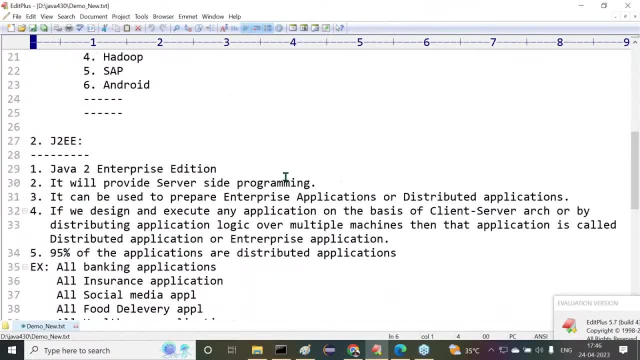 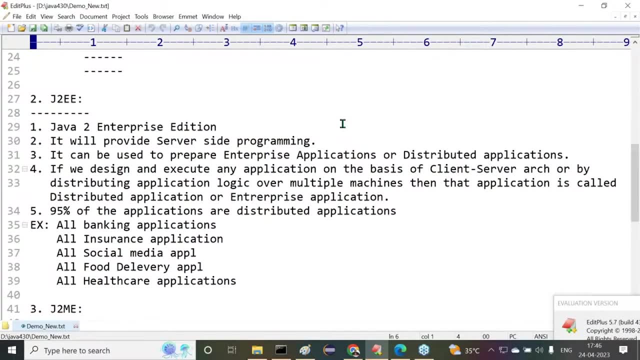 technology. Okay, clear after that. next one is: like what that J2EE Java to Enterprise Edition? It will provide server-side programming. It can be used to prepare Enterprise applications or distributed applications. If we design and execute any application on the basis of client-server architecture or 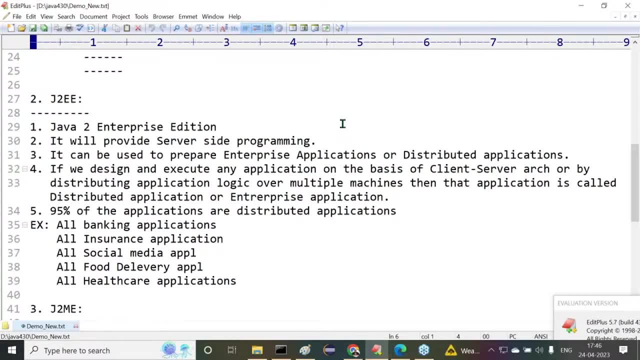 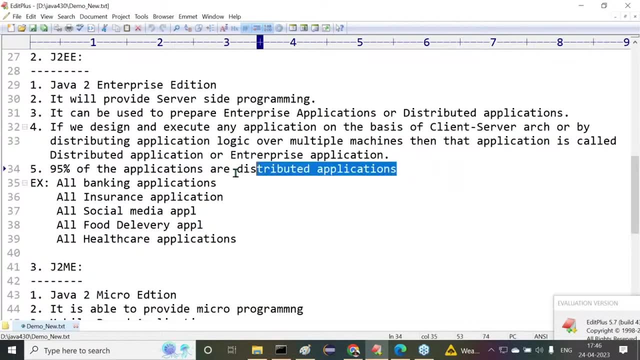 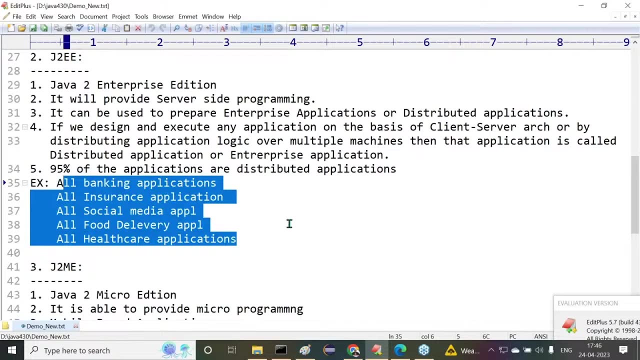 by distributing application logic over multiple missions. then that application is called as distributed application or Enterprise applications. 95% of the applications are what their distributed applications only. examples are given: all banking applications, all insurance applications, all social media applications, all food delivery applications or health care applications, and. 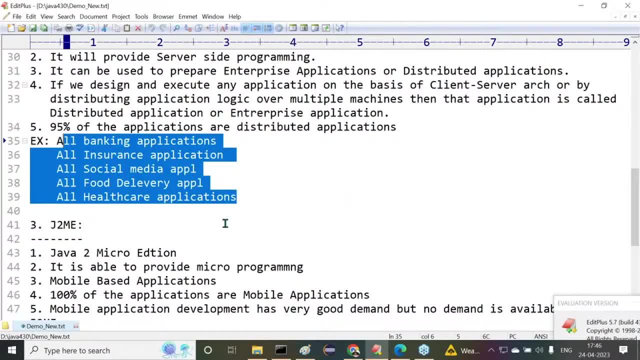 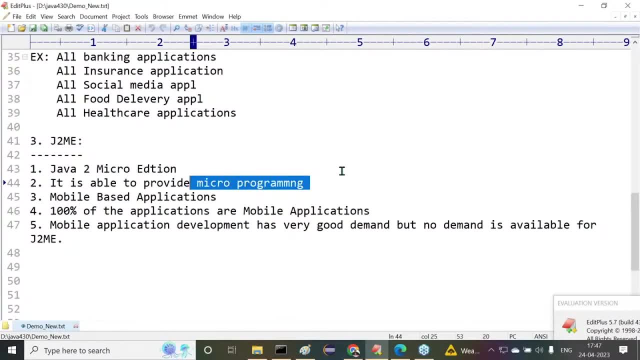 so on, and so on, and so on. All these things are like what they're like: Enterprise applications. only last one is what their J2EE Java to micro edition is able to provide. what programming care? no micro programming. by using this micro programming. what type of applications care we are able? 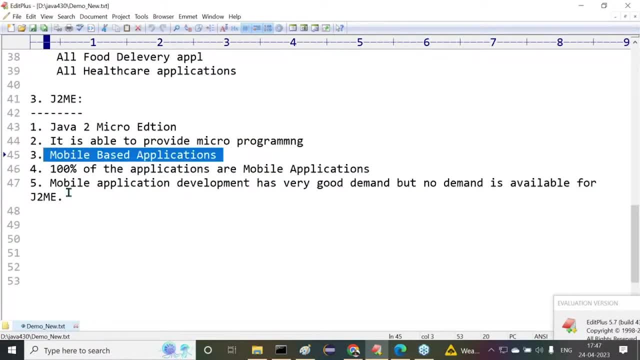 to prepare their mobile based applications. How many applications are mobile based applications nowadays know hundred percent of the applications are what their mobile based applications. all right. next point is what? what we are given there. This is important. Mobile Mobile application development has very good demand in our search, but J2ME is not having. 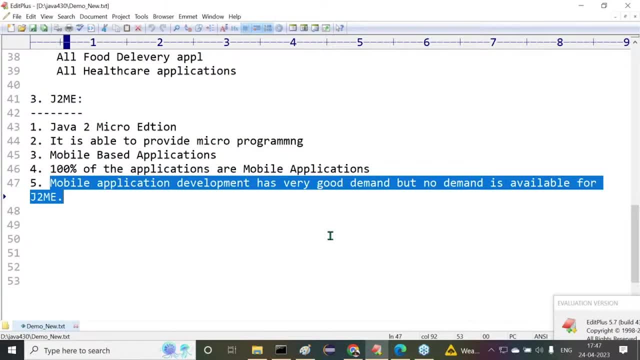 any demand. It is almost all dead in our search. Okay, Right. These are the things here We have to understand clearly about this J2ME patch. right. out of all these things, J2SE and J2EE are live at present in the Java. J2ME is not required in order to learn a J2ME. 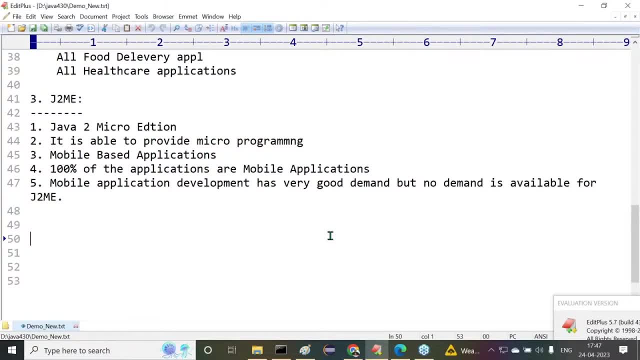 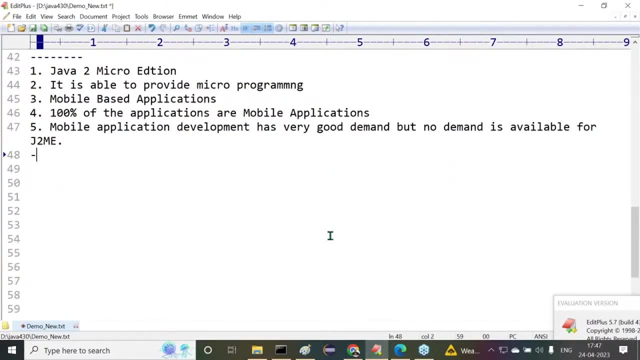 We can leave this one. Okay, Leave this content here, All right. So after this, after completion of this particular one, understand the next one again. today, I think all of you are having syllabus sheets right. I think all of you are having syllabus right, or else even after completion of the class. 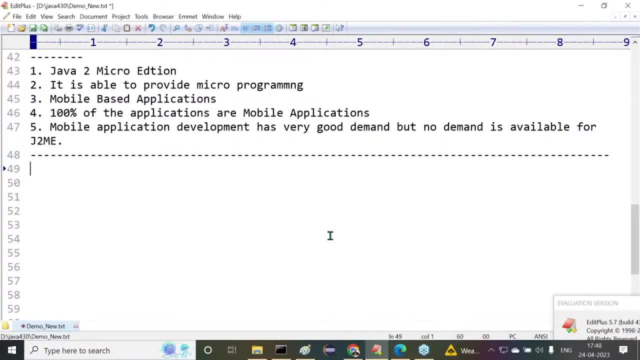 you are able to get a WhatsApp message about this syllabus- no content, but I'm going to discuss with you. All right, If you want to up to this RS, maybe just two minutes of time. if you want to see the syllabus content here: 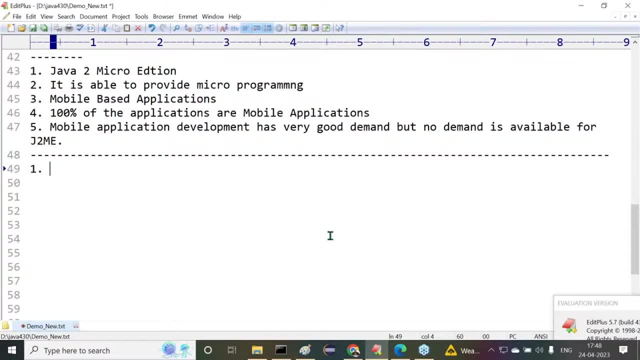 I can give a list of content. So many content concepts are available. I'll give that list of content here. Let me give some list now. after that I'll start our introduction content. clearly, parts of the first one is like what their introduction and the second one is like what their steps. 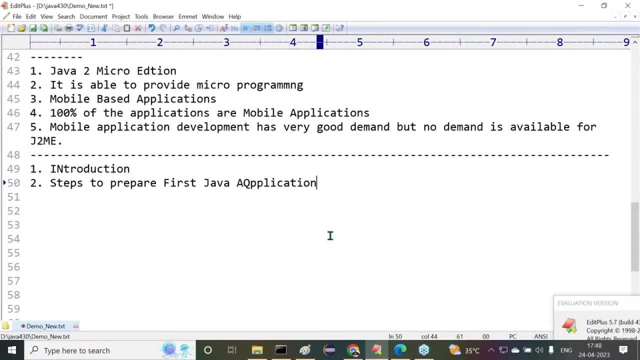 to prepare first Java application, then, after this, steps to prepare first Java application. third one is what their language of fundamentals, after this language fundamentals, object orientation? Oops, This is very, very important. This is the heart of the Java object orientation. Everybody must understand this. whoops without knowing that, whoops we are unable to understand. 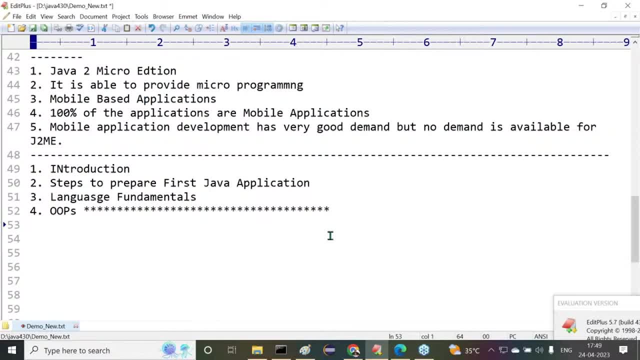 anything in Java, All right. Next one is: after completion of this object orientation, The next topic will be like what their some wrapper classes, and the next one is like what their some inner classes. next seventh one is like what their packages. after this, eighth one is what their string manipulations. 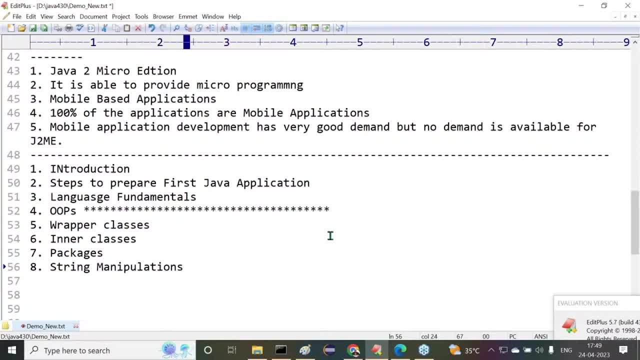 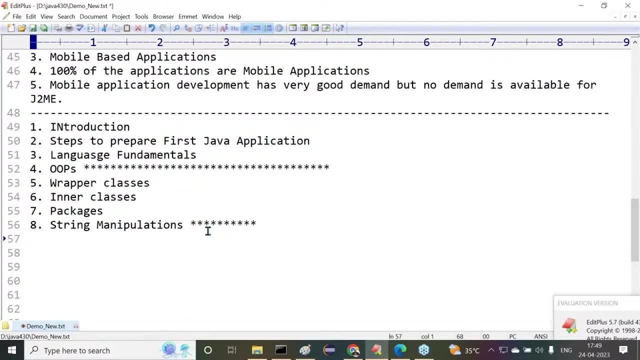 Okay, Next one is string operations. This is also being important content string operation So many times here We are going to use the string operations that in every project as a common, common operations We are going to perform comparing two names, checking whether that email ID is a proper. 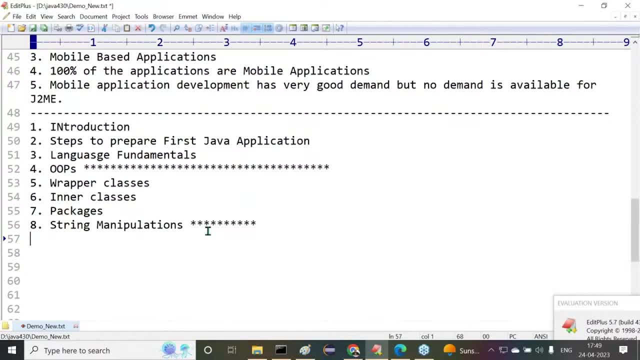 value, proper email ID or not anything- all the things that we are going to do in frequently, we are going to use in our application schedule. next one is: like what the now for this string manipulations? Next one is: we need to go with what their 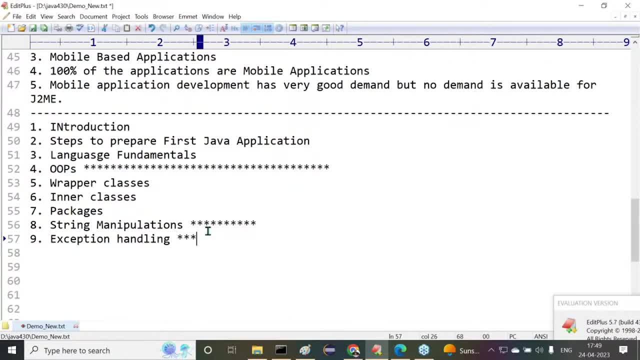 Exceptional handling, this also being another important one after this exception handling. next one is like what their multi-threading- multi-threading is also being another important one after this multi-threading. next one is what their I was streams, I was, seems is okay, little bit, not completely, then little bit important one get. few topics are important. 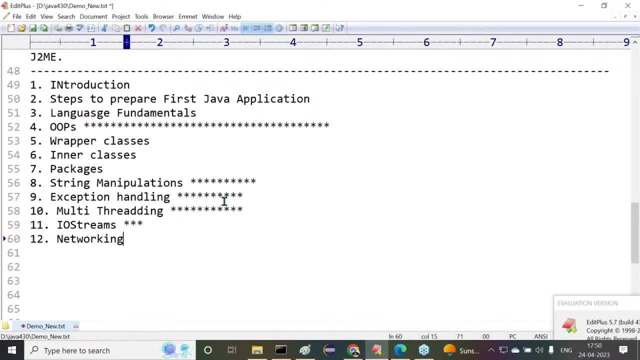 of a completion of this. I was seems wrong. Next one is what? their Networking outdated, but still. we are going to discuss that as part of our content kit. next one is RMI- remote method invocation after this RMI. next one is: like what their arrays? 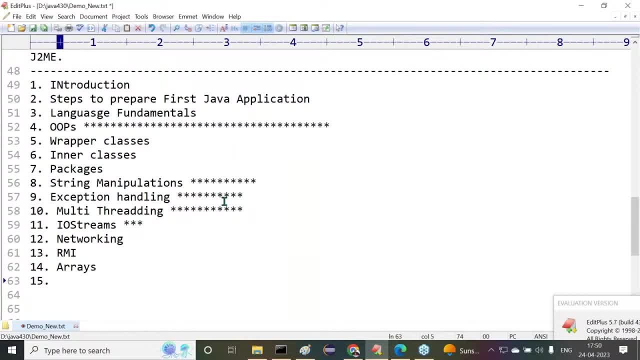 topic I will discuss. get at the 14th topic, 15th one, like what their collection framework. This is another important offer: the object orientation. The second important topic is what their collection framework. next one is what their string manipulations, exception handling and multi-threading are nominal. 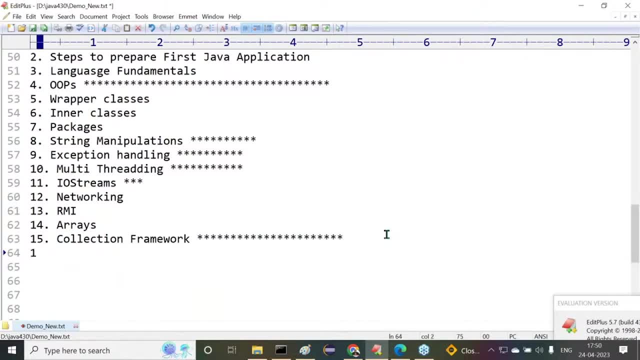 After completion of this collection framework, then what next one? care, we are going to understand, their reflection API. after this, the 17th one: what their annotations? then, after completion of this annotations, The next topic will be like what the GUI patch in a GUI AWD? and next one is like what their 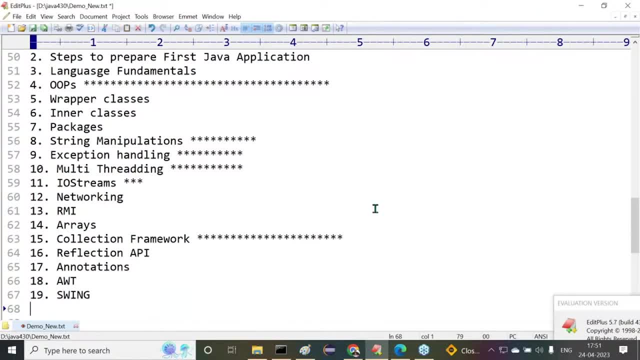 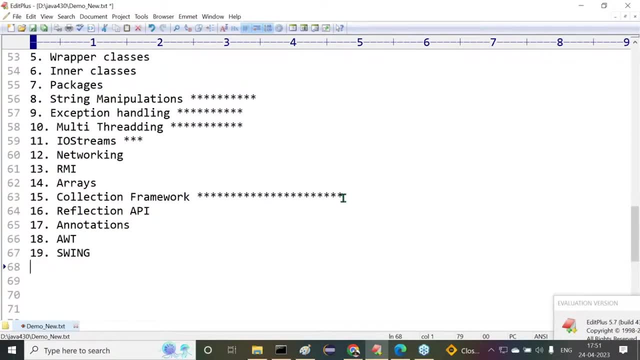 swing, even though they are outdated. but little bit awareness I'm able to provide, or because just idea not utilized in outside, Not just idea I want to provide. their internal topics are important, But It was, it's not required, but their implementations are important. 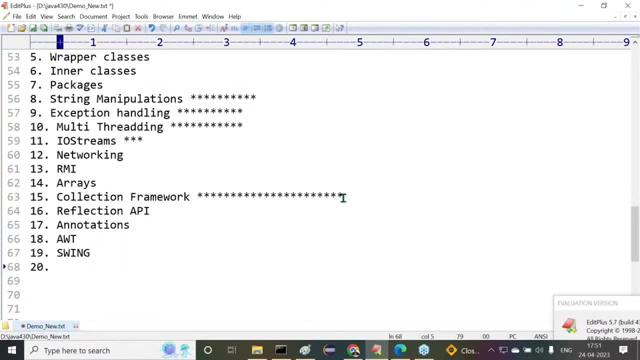 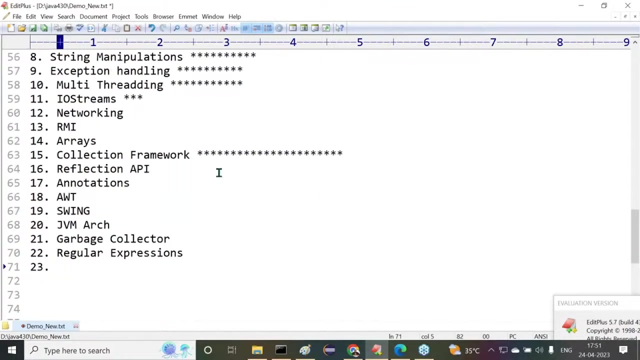 That's why I'm going to discuss about it after completion of this. next one is like what their JVM architecture. offer this JVM architecture, We are going to understand. garbage collector- After this garbage collector. next one is like what the regular expressions After this regular expressions. another topic is like what their right side? 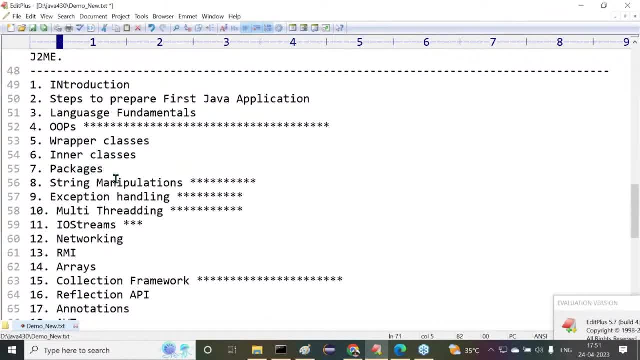 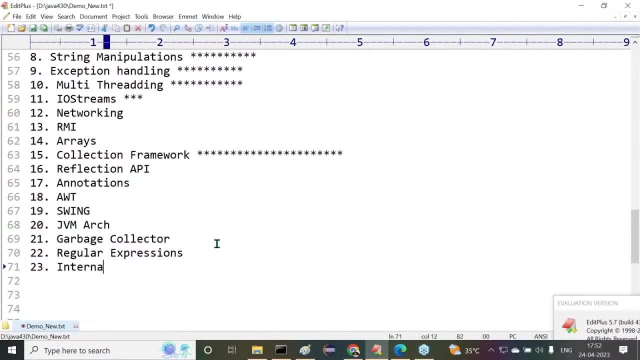 Now get another content care introduction in our class. I covered, okay, fine, JVM, architecture, garbage collecting regular expressions, internationalization, internationalization. then after completion of this internationalization, all right, anyway, in the list of topics here I'm giving there, if any topic if I miss, know then non-flow, I'm going to be covered. get after completion. 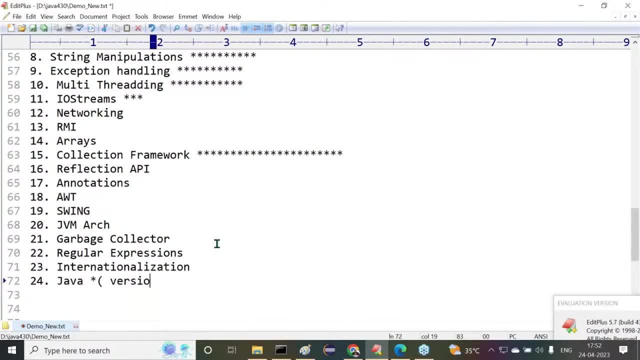 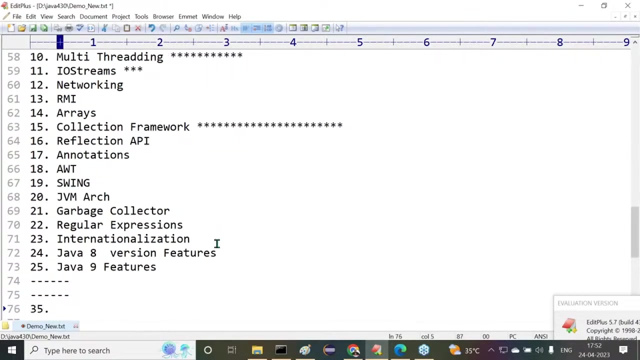 of this content care. Java 8 version features: Okay, Okay, Java 8 version features Right from Java 8 job. next one is like what their Java 9 features, And so on, and so on, and so on, like this, maybe almost 35 to 36 now here. 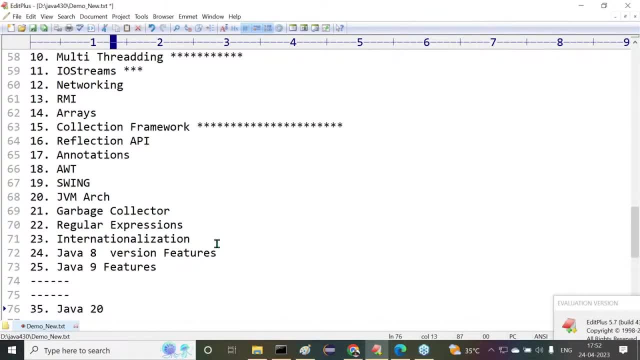 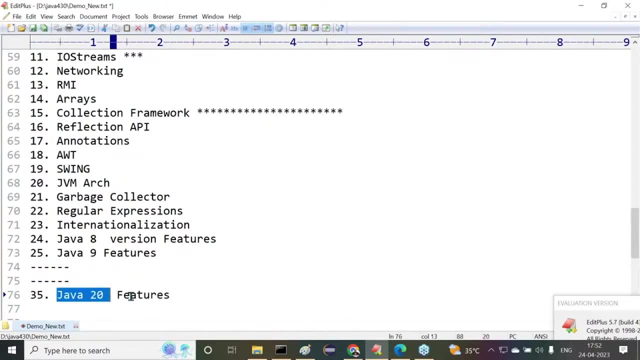 At present. I think so. as per your say, Java 20th version. I think so. it is available. right? you said to me Java 22 features also. I'm going to prepare, I'm going to explain to you, but as of now, on java 20th up to java 19th, okay, but i can discuss that, but i'll update it as a matter of one day. 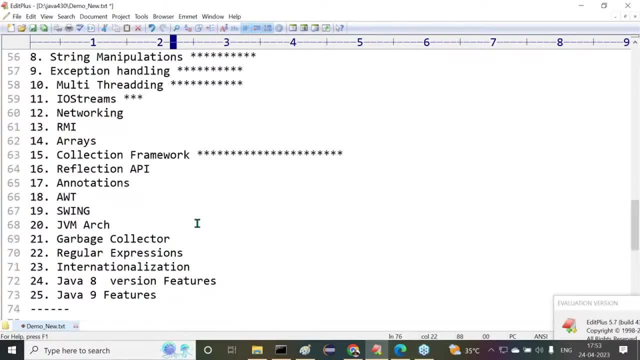 i'll discuss even up to java 20th version there now. so these are overall the topics here, what we are having there. clearly, if any one or two topics might be missing here, but overall content, i'm going to discuss with you. use content, every content. why? because it's a core java fundamental. 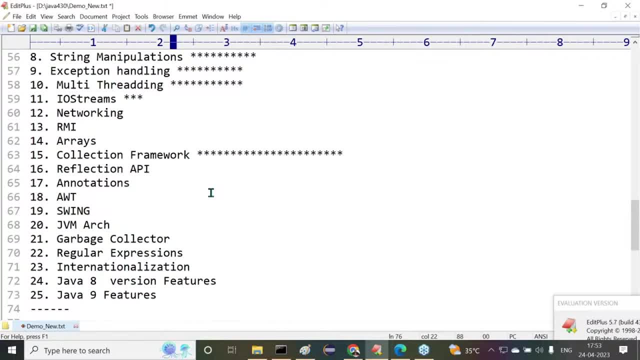 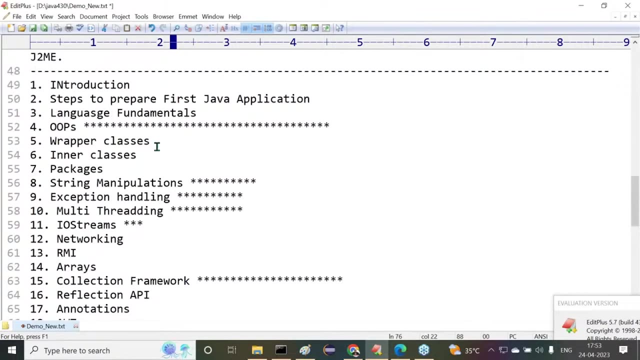 if you know fundamentals, no, then only we are able to understand what their remaining content effectively. without having these fundamentals, we are unable to understand the java in the future. that's why i'm going to discuss more and more about this particular content. got it or not? just only headlines, only titles i have given, if i take each and every title where internally more 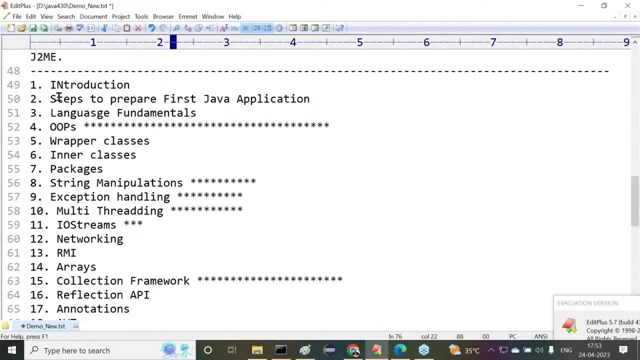 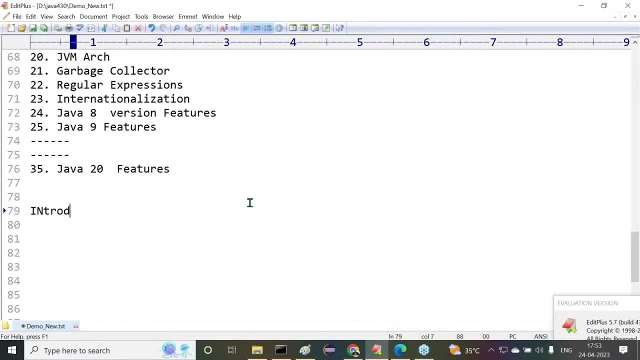 content is going on so that i have to discuss there. clearly. fine, all right. so after that, after understanding this, now let's come for the introduction part today. introduction in the introduction: what topics are available, what exactly the content is available in the introduction part? again, observe carefully. 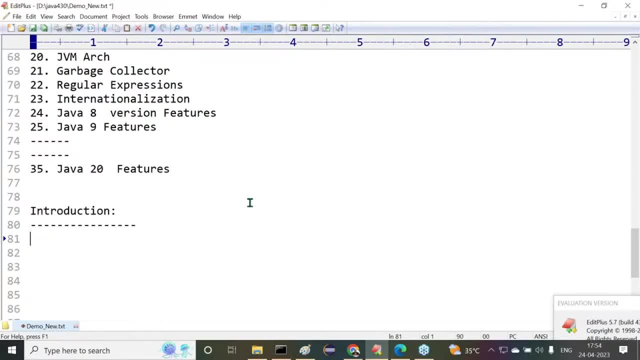 what exactly the content is existed here. observe carefully inside the introduction topic. first one is java history, why java is coming into the picture. who has provided this java? what exactly the work that java people have done to prepare the java programming language- all these points, the content. here we are going. 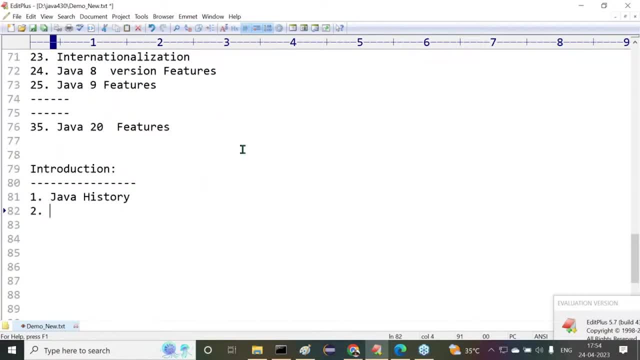 to understand java history. after these differences between java and others here- others in the sense like what they're, c and c plus plus why java is coming- what differences you identified between java and other programming languages like c and c plus plus what differences you identified there why java is the? 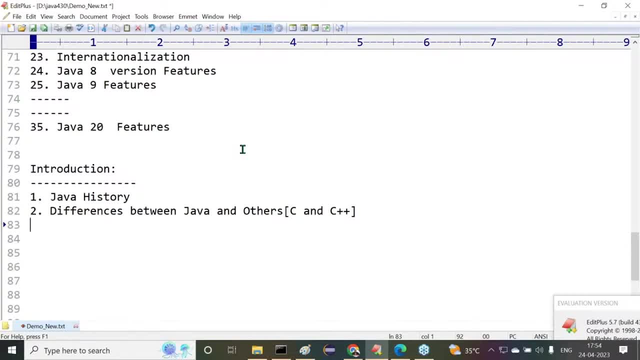 best of when compared with the c and the c plus plus. and, moreover, some people are having awareness and like what there? to learn java first, we need to learn c plus plus. to learn c plus plus first we need to learn a c. people are having this kind of awareness but, strictly, i'm telling you java core. 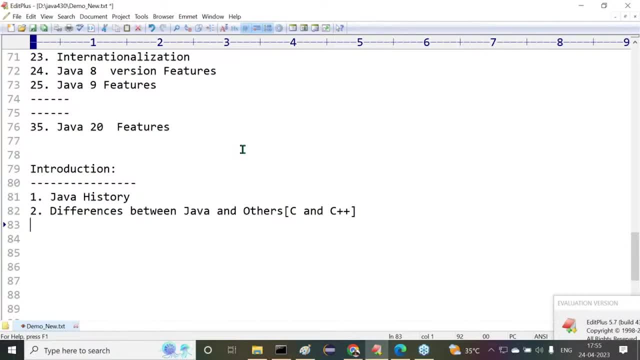 java is a foundation language, fundamental programming language. no need to learn any other prerequisite. core java is a prerequisite. core java is a fundamental topic for this fundamental language. no other prerequisite is available directly. we can start with java. so to specify this particular point only, i'm giving some comparison like what there java with the c. 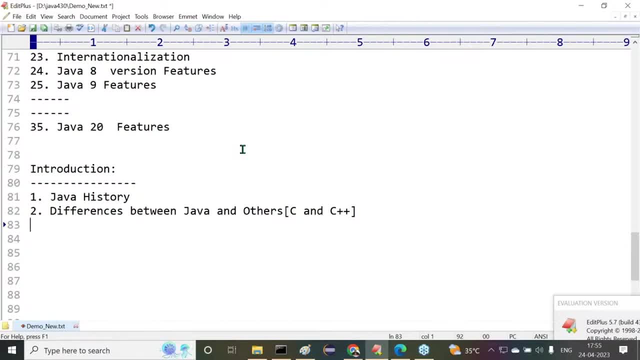 c plus plus, what exactly the differences are available, what differences you understood. we are going to say clearly why java is good when compared with the c and c plus plus all the things you are going to be covered there. that is one thing now. after that, after completion of this, 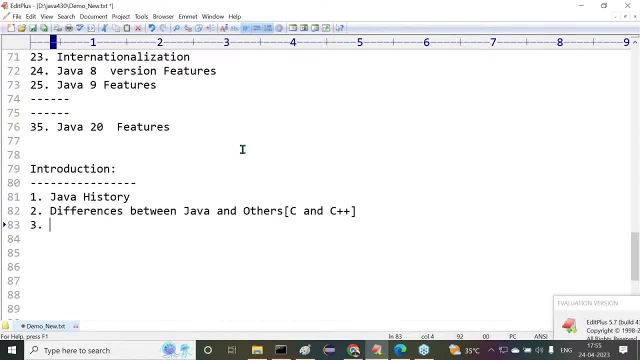 after understanding the differences, no. next one is like what there? java features in five minutes of time. in five minutes of time, what is java? if you want to know what exactly the behavior of the java, what is the nature of the java, if you want to know within. 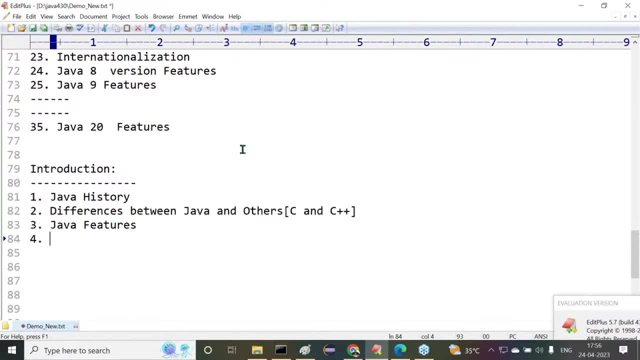 five minutes of time, then we have to go with what their java features topic. java features the topic. here we have to understand if you want to know what exactly the meaning of java. leave this one after completion of this next one is java programming format. java programming format. 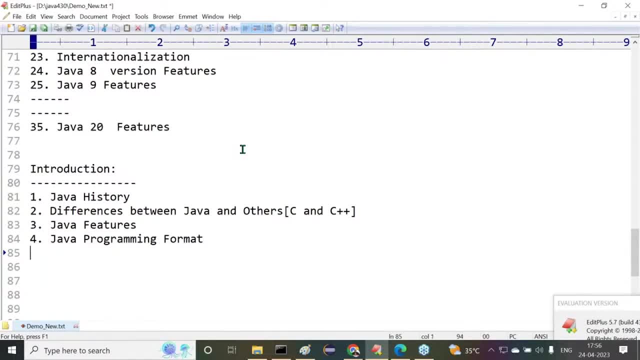 java programming format like what they. if you want to write a program, what exactly the format here we have to follow, what is the structure we have to follow to write java program that we are going to understand inside this java programming format. after the java programming format, now the next one is like what their? 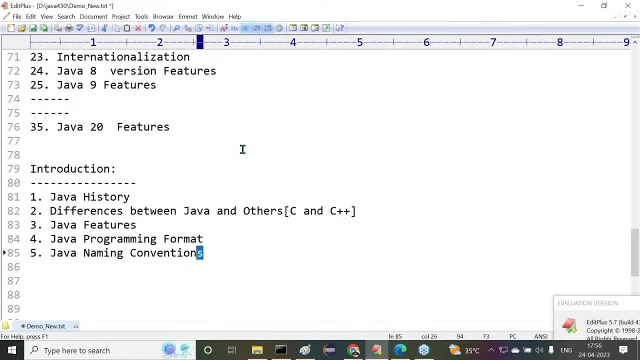 java naming conventions- or else maybe i'll make it is a fourth one, because i want to say fifth one- java naming conventions where to use lowercase letters and where to use uppercase letters. that i am going to discuss after that. here we are able to see like what their java programming format that's overall. these are the topics which are available inside. 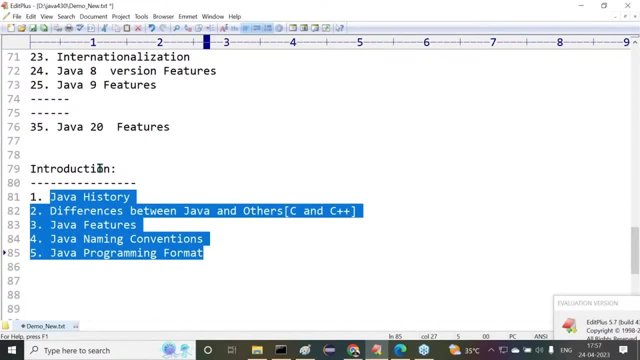 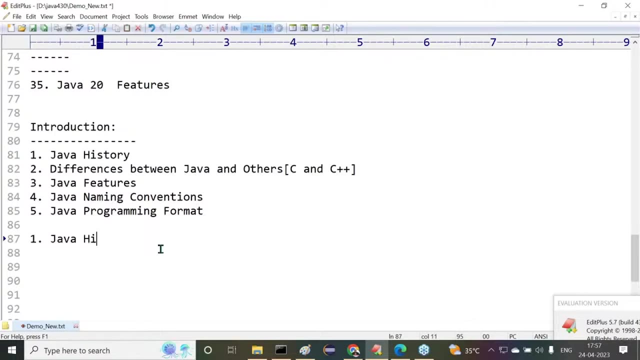 like what their introduction part? i said all if you're following or not, there's only titles. when i have given up to know nothing, i started again. okay, now shall we start the first topic now? no, there's a response, right, and the first one, very first one, is like: what their java history actually understand it? 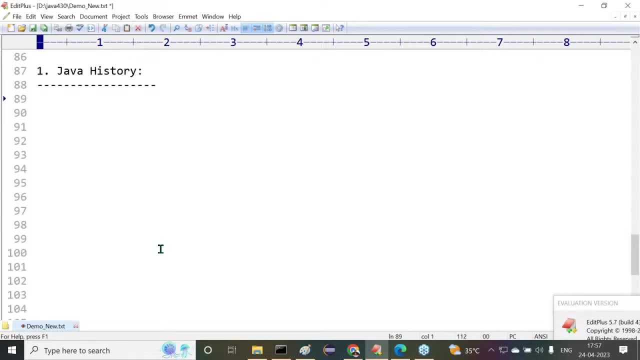 before starting this topic, i'm giving clarity. this topic is only knowledge purpose. nobody will ask questions on this. not at all important in the point of project work, not at all important in the point of interview. but every java developer should know what exactly, the reason why java is coming into the picture, who has provided java, why the java is coming. basic awareness that. 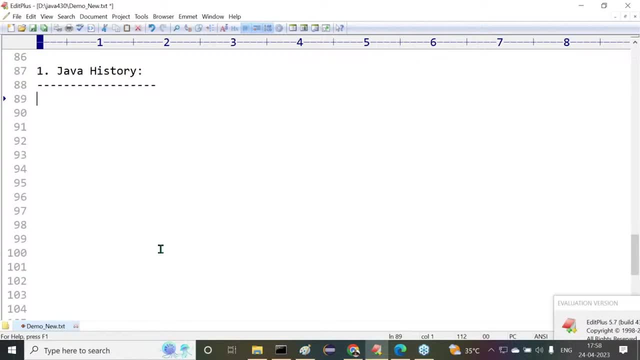 i am going to discuss now, right, i'm so carefully. tell me, guys, all of you know, tell me on which year java first version was provided to the market: 1990, 1995, 1996 is a confusion, right, 1991, no, right. anyway, i'm giving clarity. 1996, january 23rd. 1996, january 23rd. 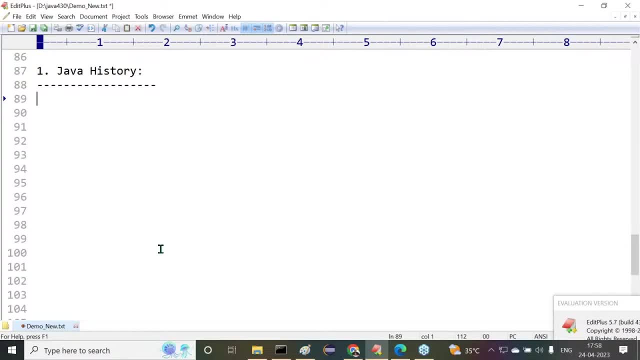 the very first version of the java was introduced to the market 1996, january 23rd. the very first version of the java was introduced- i'm so carefully. java was provided in 1996, january 23rd, in the sense preparation was started before 1996. 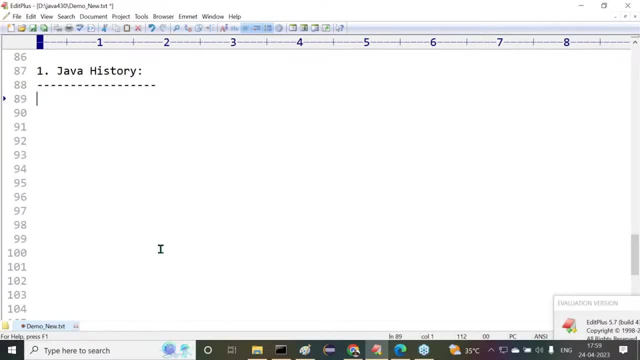 preparation for java programming, lang, was started before 1996. but when it was started, what are the roots for this particular one? i'll look carefully. in 1991 exactly, you remember the date exactly. but that is not the startup point of the java. that is the point here. understand it clearly. in 1991 sun microsystems had a requirement. 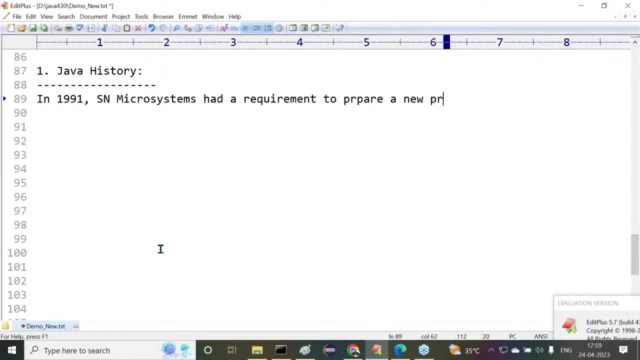 had a requirement to prepare a new programming language, to prepare a new programming language in order to prepare, in order to prepare softwares for the electronic consumer devices. like what are the electronic consumer devices? care like cable tv switch boxes, next, remote controllers, and so on, and so on, and so on. electronic consumer devices. 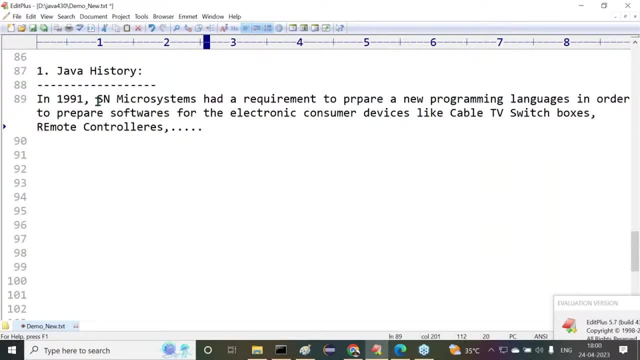 In 1991, Sun Microsystems had a requirement They want to prepare a new programming language in order to prepare softwares for the electronic consumer devices like cable TV, speech boxes, remote controllers and so on and so on. This is actual root for Java programming language. 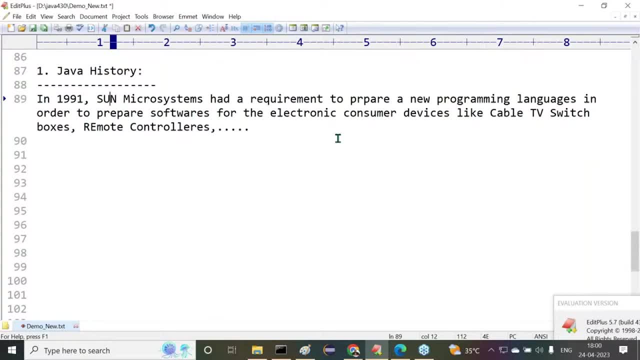 This is a requirement by Sun Microsystems wants to prepare a new programming language. Right or not right? observe carefully, understand it clearly. This is actual requirement. for this particular requirement, Sun Microsystems has gathered 30 engineers. Sun Microsystems has gathered how many members there? 30 engineers as a team. 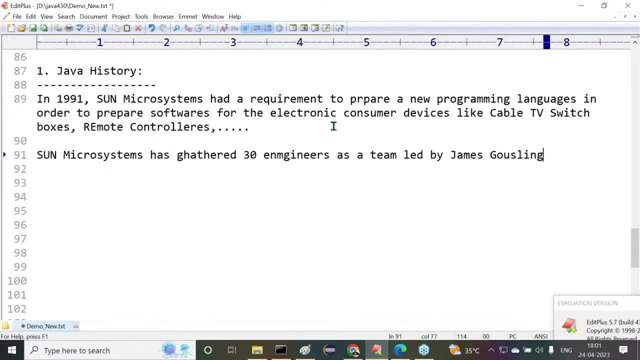 Led by James Gosling. led by James Gosling- I think you already aware about this name. right, familiar Sun Microsystems has gathered- nearly as gathered- 30 engineers led by James Gosling and Patrick Norton. Patrick Norton is another person. They are the two members lead for this 30 members team. 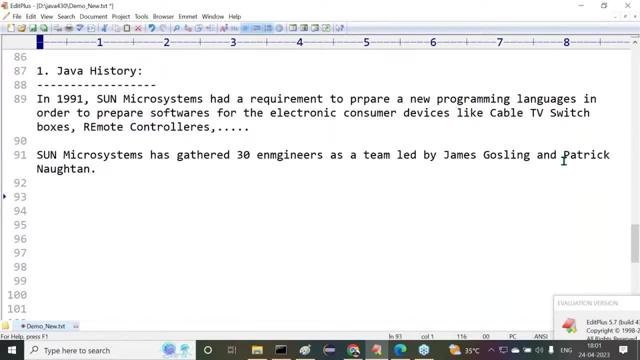 Right or not. all right, with the 30 members team, Sun Microsystems has started what they started. that Sun Microsystems started a project, a project named as green green project. It is 30 members team. Sun Microsystems has started a project named as what they started. 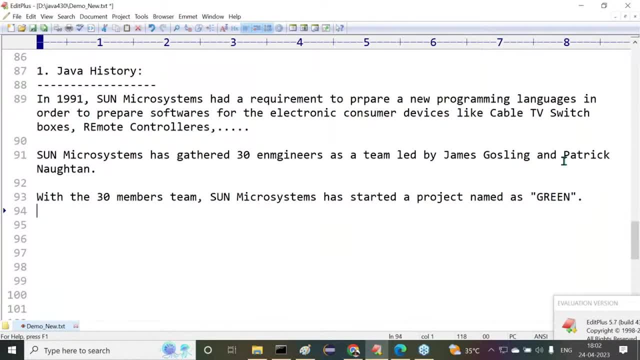 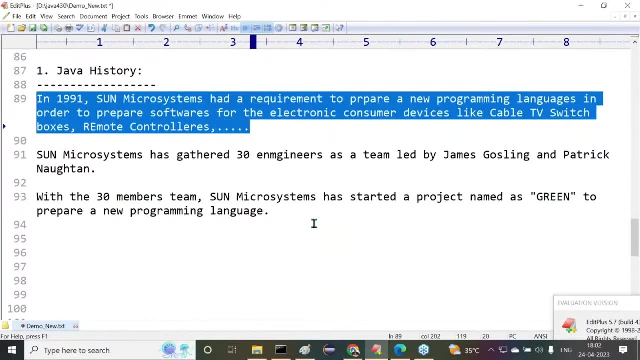 A project. They started a green project to prepare a new programming language. Come again, What exactly the requirement of the Sun Microsystems? at 1991,, Sun Microsystems had a requirement to prepare a new programming language in order to prepare softwares for the electronic consumer. 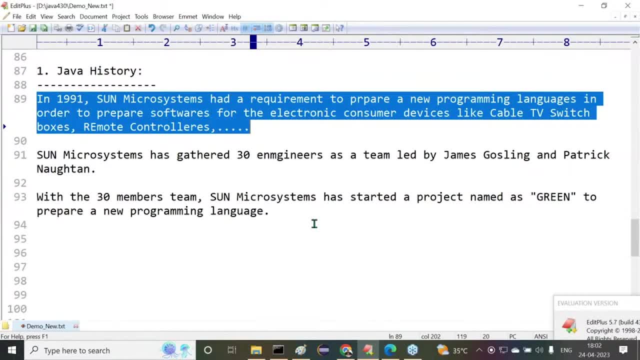 devices like cable TV, switch box, remote controllers and so on. See, it's a matter of electronic devices. Okay, For electronic devices. Sun Microsystems wants to prepare a new programming language. That is a requirement of Sun Microsystems in 1991.. 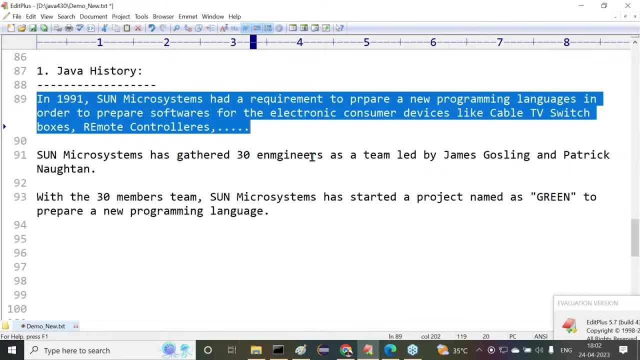 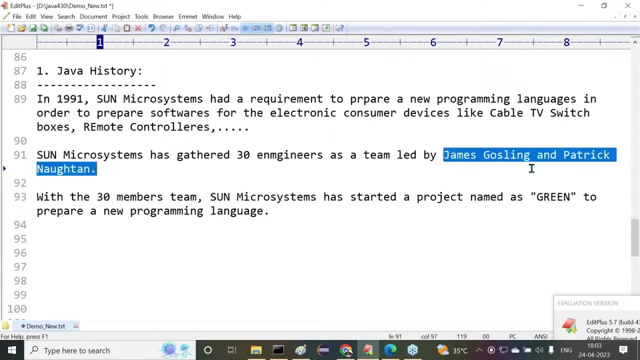 Clear. Sun Microsystems has gathered nearly 30 engineers as a team to prepare this new programming language. The team leads are James Gosling and Patrick Norton. I was a carefully James Gosling and Patrick Norton. Actually, Patrick Norton is a key person there in Sun Microsystems. 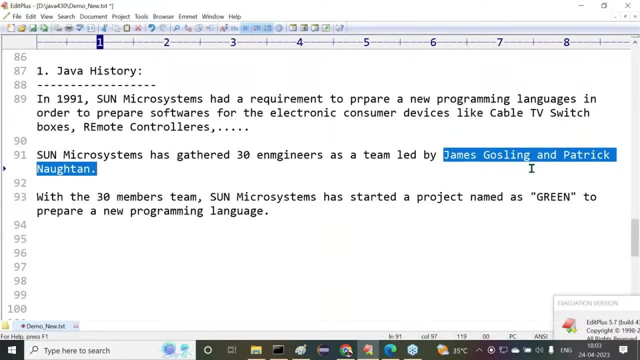 But the whole credit. Okay, He's available with what their James Gosling. strictly speaking, James Gosling was available with the Sun Microsystems up to Java third version. only after the third version he left from Sun Microsystems. He went to some other organization. 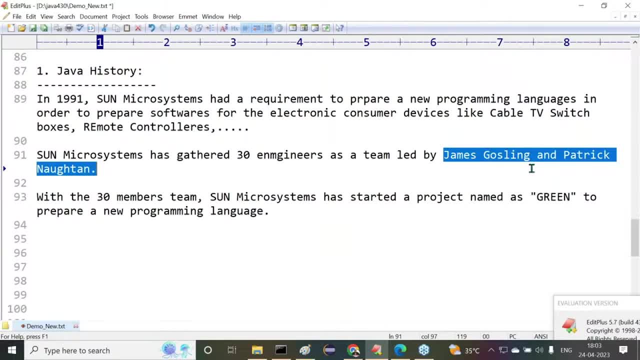 Now he's not with the Sun Microsystems or Oracle corporation, but up to third version of the Java, only James Gosling was available at the startup point of time. James Gosling is the lead for it, But actually key person in this entire team. 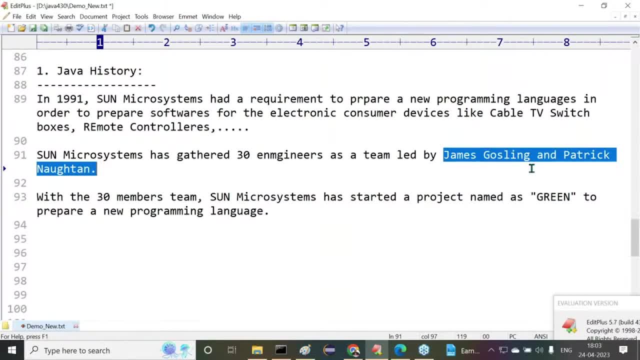 That total Java journey is what their Patrick Norton still. Patrick Norton is available with the Java Still is a part of the Java. Understand it? No, Okay, Leave this one, But most of the people are saying that, father of Java, who is the father of Java? James. 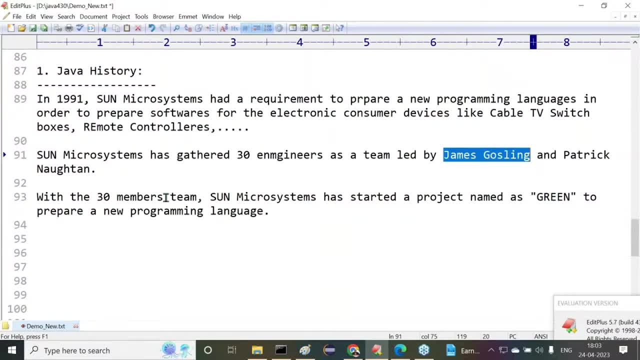 Gosling. James Gosling is the father of the Java. Okay, It's okay, Fine. Next one is with the 30 members team. Sun Microsystems gathered, or started, a project named after James Gosling. James Gosling is the father of the Java. 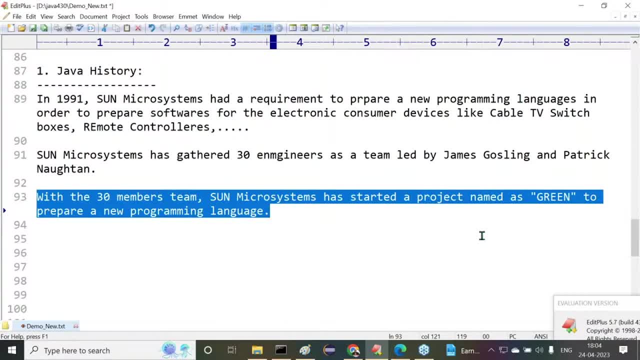 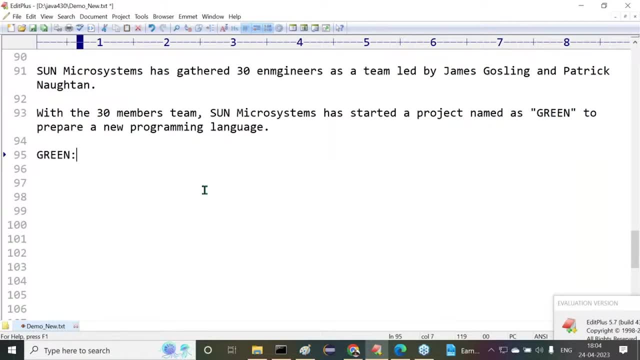 Okay, It's okay. Fine, Let's name it as what: their green project. Okay, Fine, In a green project, they want to start a new programming language. They want to start a new programming language. In that new programming language, they want to see three main features. 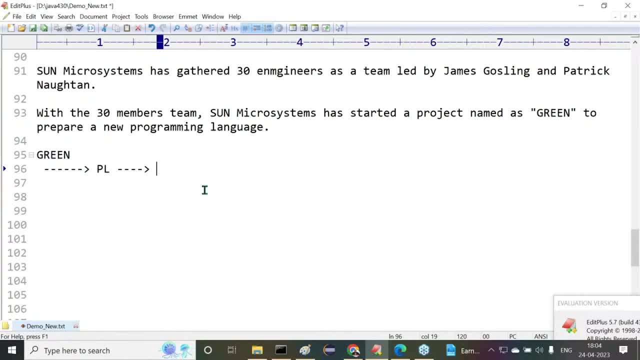 Understand it gets to their analysis mode. only Just think of it. We are at 1991.. We have an intention: We want to create a new programming language. But before going to start to prepare New programming language, Before starting its implementation, first we have to analyze it. what features we want? 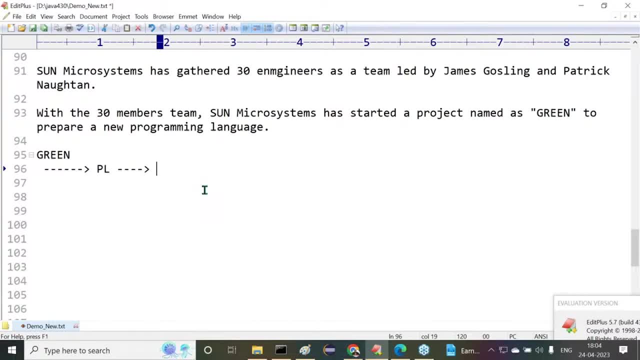 to see in that new programming language what we want to implement in this new programming language, that, if we come for this point, Sun Microsystems wants to see three main features in their new programming language. What are the three main features they want to see on their new programming language? 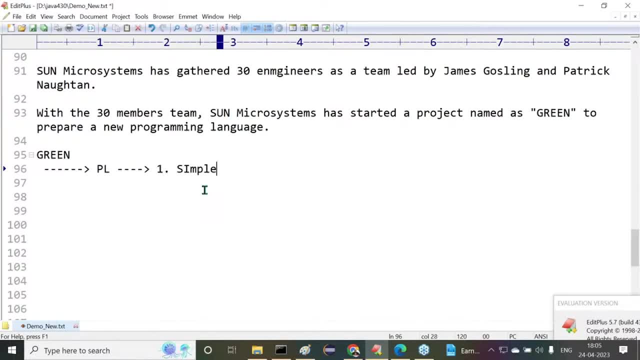 First one is a simple programming language. Come on, sir, Then what is this? First one? you know, a simple programming language. And the second one is tight-coded programming language, tight-coded programming language. And the third one, they want to see architectural, neutral programming language, architectural. 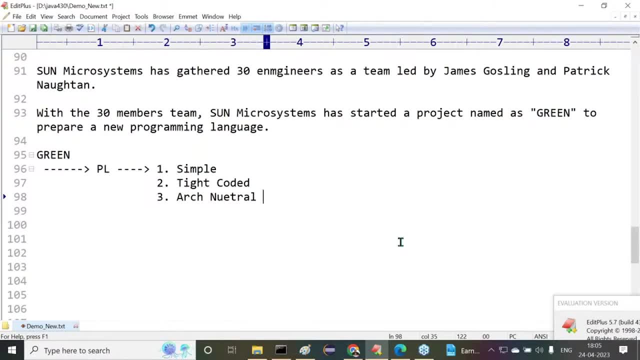 neutral programming language- these three features they want to see and their new programming language. They don't started to prepare new programming language. still there in analysis watch the team was formative. They gather They started a project inside this. They want to see on paper what features they want to implement. 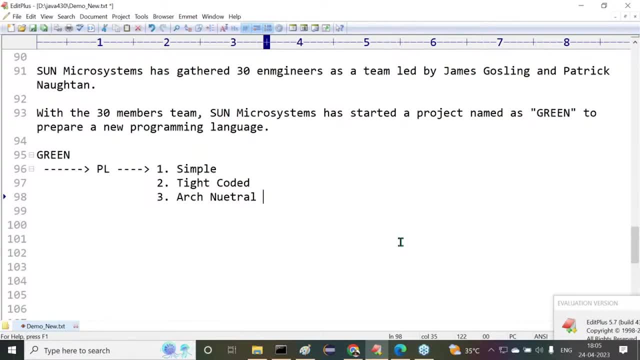 Finally, they identified three features they want to provide in their new programming language. What are the three features they want to say in their new programming language? First one is what they're simple. Next one is what they're tight-coded. next one is what their architectural neutral programming. 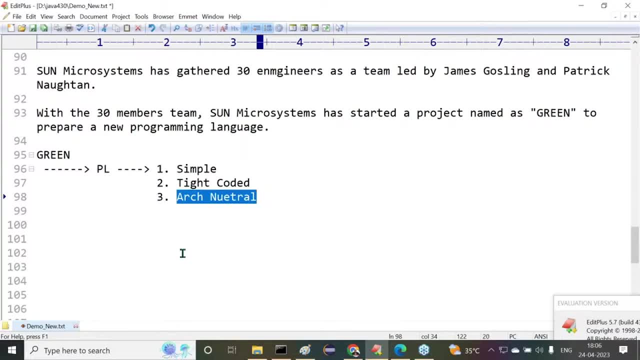 language. No, we are going to analyze, No, we are going to elaborate. We are going to elaborate. All right, sir, Why that programming language is a simple programming language, How that programming language is a simple programming language, how Java people are. 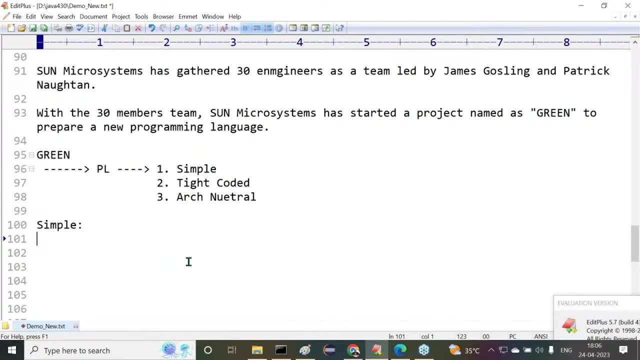 saying that their programming language, how Sun Microsystems, is saying that their programming language is a simple programming language. If you come for this point, they are given some reasons. what are the reasons they have given? their first one is: The programming language must take less execution time. 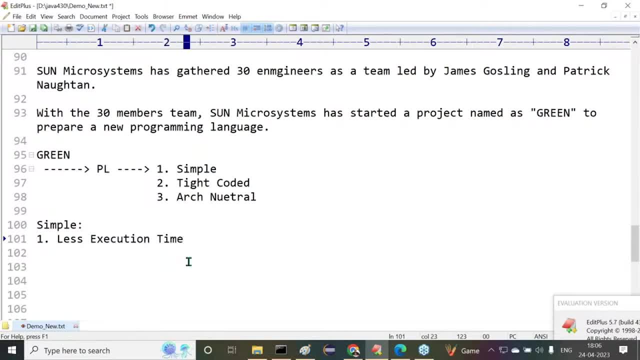 The programming language must take what they're: less execution time. within less execution time that enter program has to be executed. And second reason they are given that the programming language should take less memory, Less execution time. Another one is what they're less memory. 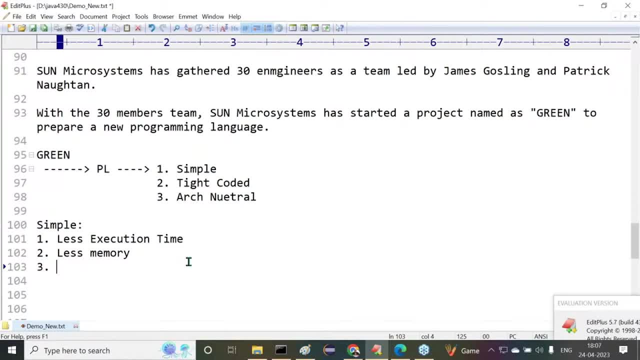 And the third one. third one is a funny thing- Even myself also initial I didn't believe it- That- For getting information from Sun Microsystems documentation. I came to know that, Okay, This is also a valid reason What they're given the less power consumption. 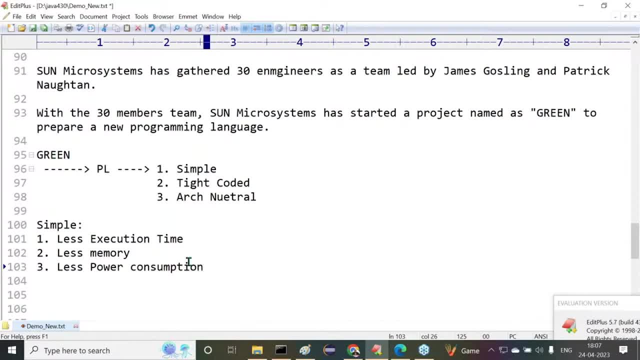 I thought of it. What is the relation between programming language and power consumption there? But they had given some kind of reason. What was the reason that we have to understand clearly, Right, sir? Anyway, I'll talk about it clearly. Let's come for this one. 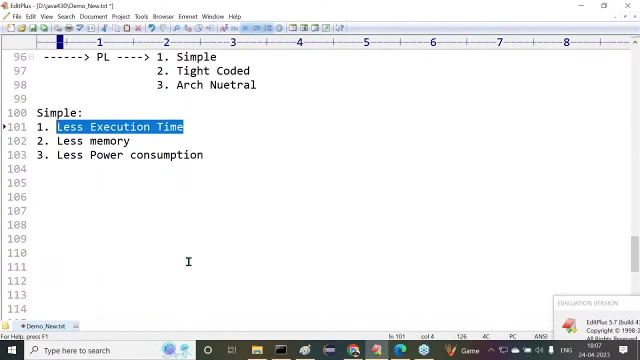 What is this first one here? No, It says the less execution time. less execution time. What's the impact of this less execution time? No, simple example is: a lot of chips are careful. There is a simple point, For example. So I'm watching a football match in my TV channel. 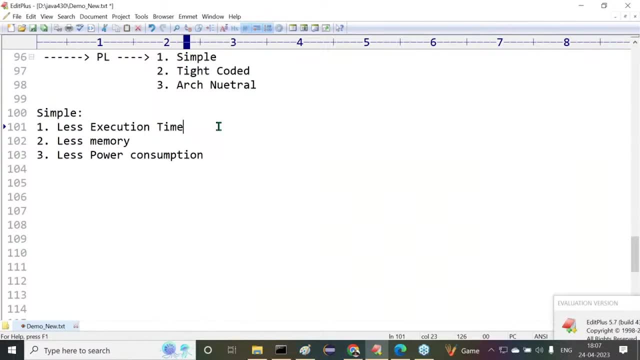 The channel number is what? there ESPN is available at 72 channel number. What is the point? Is it real? I don't know. Are you asking me watching a football match? my friend made a call to me, just had a small discussion then after that he asked it to me. 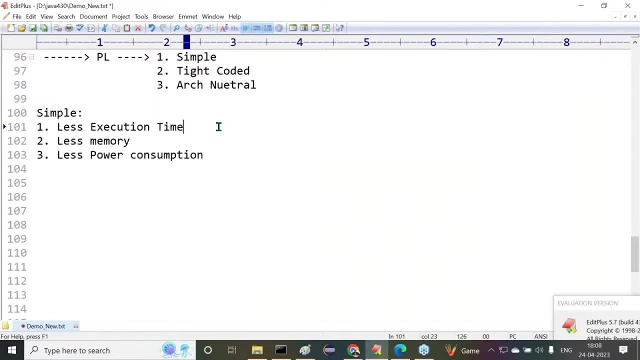 then what we are doing at present. as i said to him, yes, i'm watching a football match- immediately, said to me, are a fool why you are watching that football match. at other channel, star sports one channel, there is a cricket match between india and pakistan. the match is going on. effectively, pakistan were batted. they got nearly 321 runs. 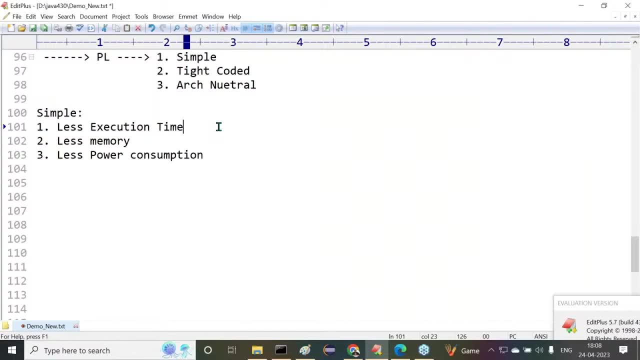 indians were started batting. almost all 49 overs are completed. last war is remaining in last over 21 runs india has to get. at one side, crease dhoni is there. at other side, ishan sharma is another failure. they are the two batsmen they are. might be they are fighting for. 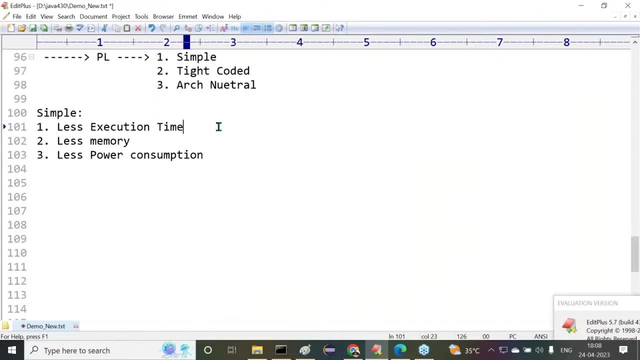 win. now, while you are watching that football match, then try to change your channel and watch that cricket match. my friend has given this clue for me. then, immediately then, as for my friends information, i'm getting crazy. and what their cricket match? obviously i want to change my channel and i've 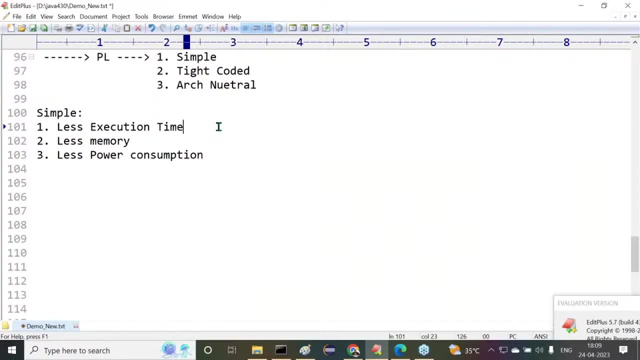 taken remote controller, remote controller. again, i know that the dspn channel is what this 72 star sports one is going on at 75- 75 channel. so i've taken my remote controller where i typed a seven and a five on the remote controller. then what is going on at 75- 75 channel? so i've taken my remote controller where i typed a seven and a five on the remote controller. 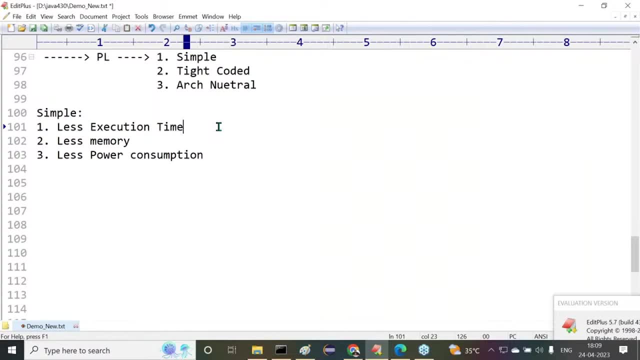 on what is happening there. it has not switched immediately after sometime. it has switched after sometime when it was featured when i absorbed the cricket match. then what happened? man of the match presentation is going on. dhoni is getting man of the match. i thought of it at least. i want to see the last power. 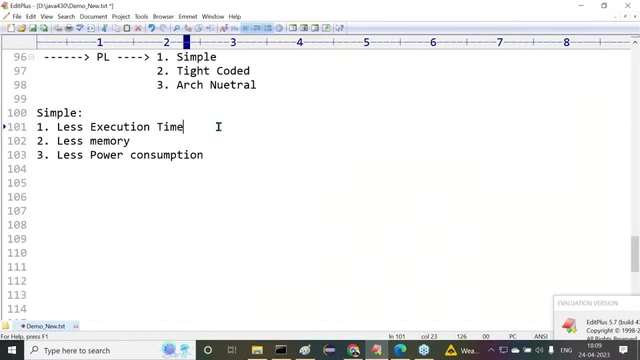 i? i on time only. i have taken remote controller and i changed the remote and i changed the match channel, but my tv was not switched immediately. it has taken some time. the moment when it was switched, when i observe there what's going on, their man of the match presentation is 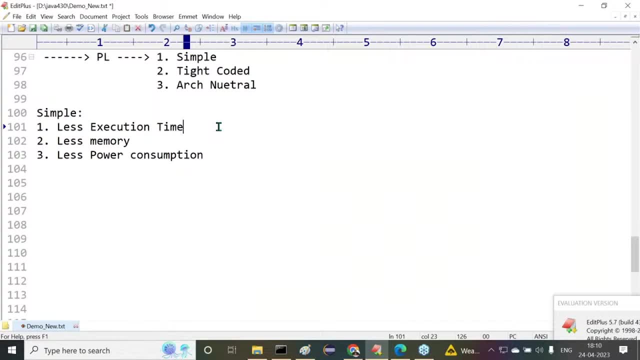 going on. ms zone is getting man of the match. he got nearly 70 plus runs. where is the problem? watching football match is a problem for my search. giving late intimation by my friend is a problem and match between india and pakistan is a problem- all right, so the problem is where. remote controller is a problem. 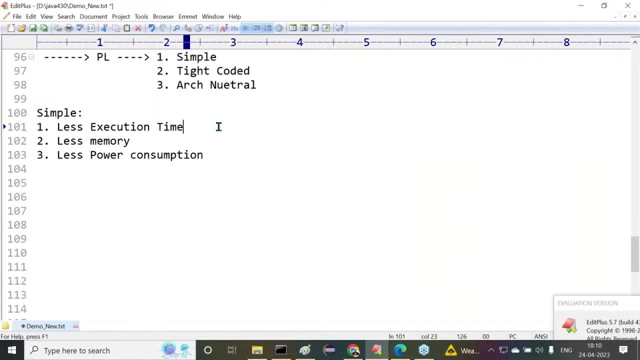 not with the tv remote controller is a problem. understand it. inside the remote controller. what happened there? inside the remote controller, when i type a 7- 5 channel number immediately it is not performing its functionality. it has taken some time. it has taken some time to perform its functionality means that internally there is a. 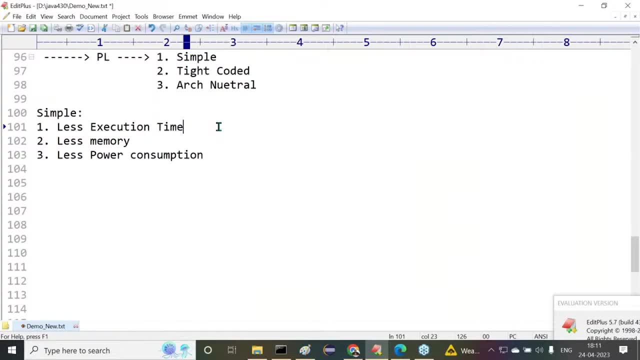 program inside the remote controller there is a program. when i type 7 of 5 internally, that program has to be executed. that execution time of that program is taking more. when it has taken more execution time. when it has taken more execution time, performance of the remote controller is: 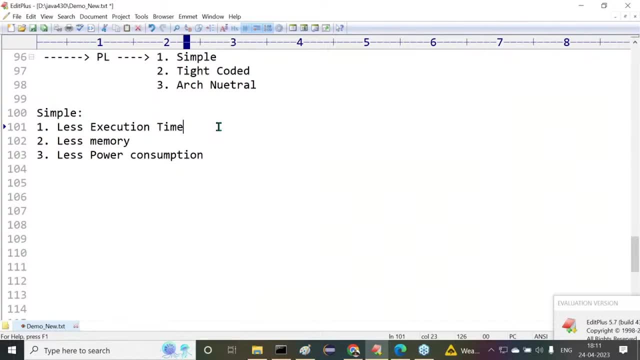 reduced. when more execution time is taken, performance of the remote controller is reduced. when a performance of the remote controller is reduced automatically, end user will not satisfy about our product. whatever the remote controller product here we have taken, i am not satisfied about my product. in the next attempt, if you want to take any remote controller, i will not. 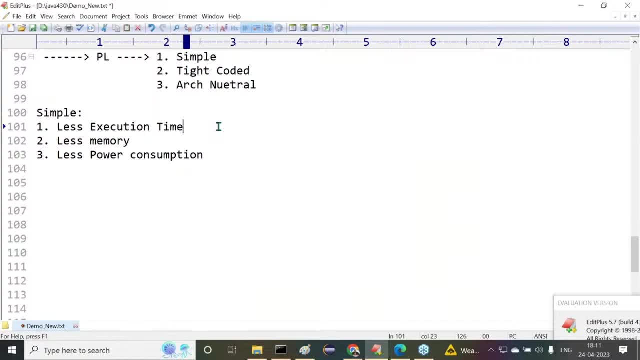 take this particular remote controller, i will buy some other remote controller. i forget my pointer, nerd. so your understand point. when execution time is more automatically, performance of the application is less. when execution time is less automatically, performance of the application is what they're more. understand it clearly. one more example i'm taking then. 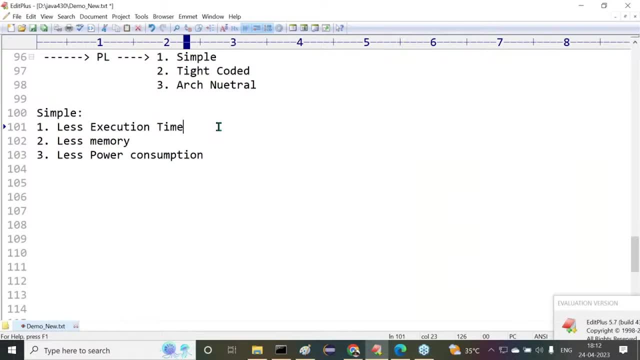 previously. i have a tab, samsung tab. when i want to go for some hotel or somewhere else, when i want to pay the bill, i need to scan. then, through phone way, i want to pay the bill. i need to scan that qr, qr code or whatever it may be. i want to scan it. 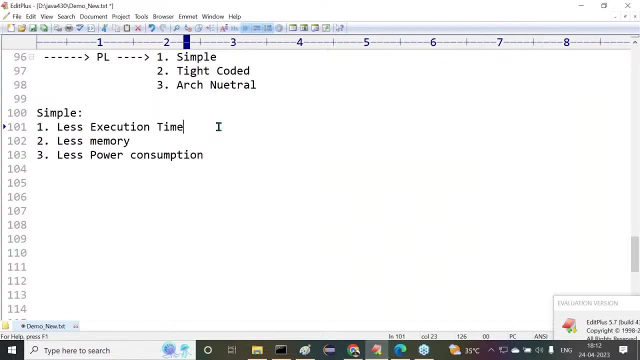 when i'm trying to scan it now, then it may take one or one and a half minute of time. i need to adjust that scanner. then only i'm able to get it. is it got it or not? okay, after that, when i type the payment, when i click on pay, maybe some circle is rotating, rotating, rotating, rotating. after that, 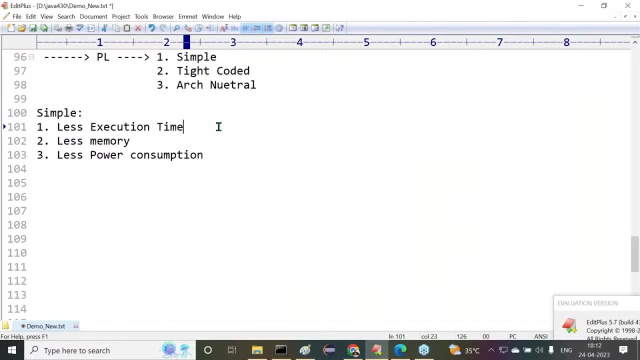 only it might be paid. then after that time i have to monitor it, i have to check it. how much time in some situation that phone pay problem may be? that circle is rotating, only it is not completing it. is it got it or not? so finally i got irritation over my tab. i decided i 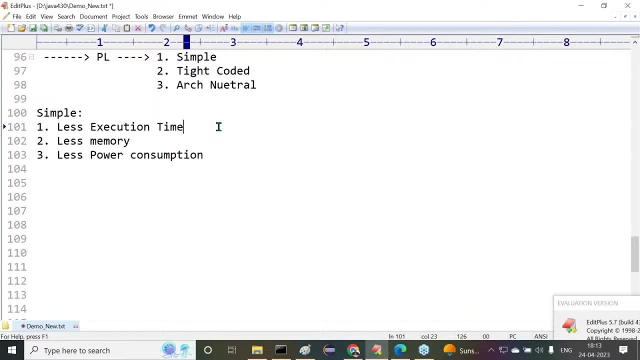 don't want to use this tab. then i want to buy a new mobile phone. i want to take a new mobile phone. after that, i waited almost all six months of time to buy a new mobile phone, but very good mobile phone i want to take. it is a real-time example. i'm telling you i experienced it with that. 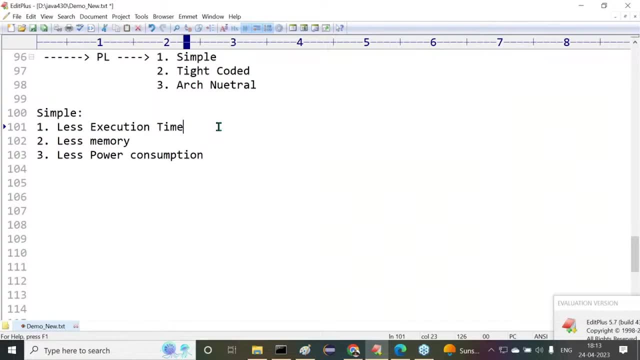 then, finally, i came to know that most other people are suggested to me try to take iphone. but i enquired about it. iphone is very good phone, but the problem is, what are they? all operations are total in reverse. then i recognize it up to at least one week. 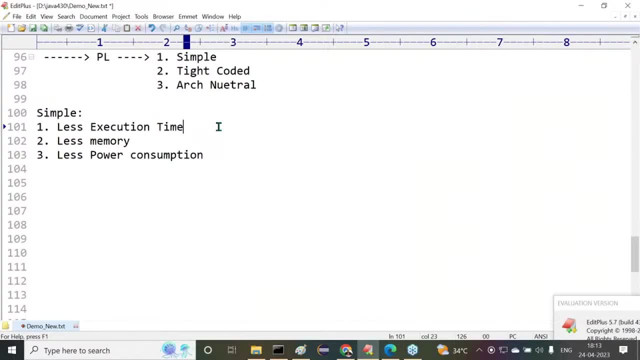 item. i have to spend my time to understand the functionality of that mobile phone, but i don't like it. when technology is increasing flexibility i have to get, but again i have to sit separately for that phone to learn, in the sense, who will assign that one week of time? i thought of it. next level, best phone is watch some other. 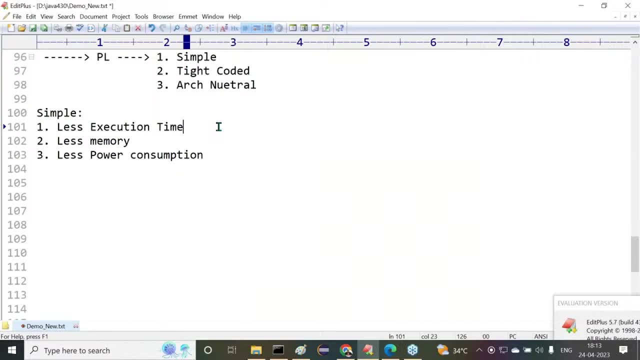 people have suggested to me take one plus mobile phone. that's okay, that that is good thing. in one plus also, which one is the top end there? i identified it, so i checked it for it. one plus mobile phone might be there. some variants are available: 4gb ram, 8gb ram, 12gb ram, but one more. 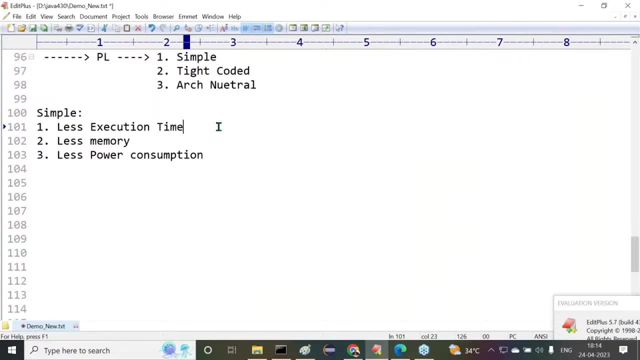 variant is available. that is what their 6gb ram- yeah, that i want to take. when 6gb ram- in the sense somewhat speed- is coming there, then i've taken right. this is a mobile phone, i have taken it. one plus when i take in this when i go to the restaurant, now, when i want to scan it, no even. 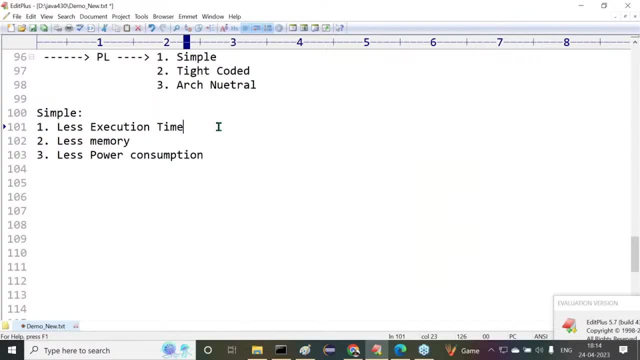 just like in a flash, if i, if i rotate my mobile like it, my mobile phone like it, automatically scanning. now tell me understand the difference. no, previously my tab i have to rotate like it is a fraction of second. just if i, if i show, like this automated scanning, which one is better. no, 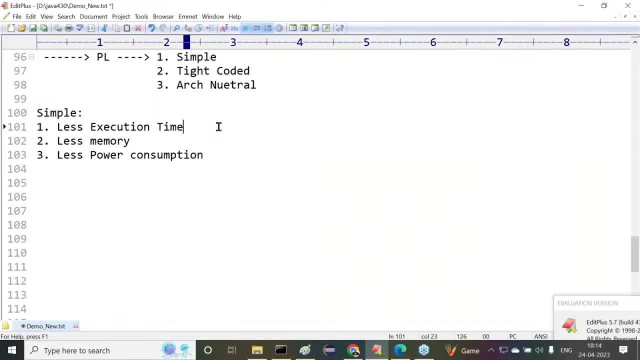 forget about money. which one is better? no, mobile phone, this one plus mobile phone is better or not? or maybe apple phone, iphone is better or not. see that that is the end user, end user feeling and the user has, he's, he's a satisfying now and the user must be satisfied. 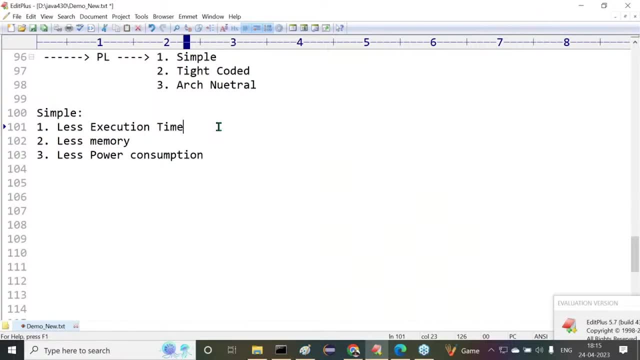 so here the point is what they, and moreover in my phone, pay when i click on it. as for this 5g network maybe, as for this phone, new mobile phone might be- when i click on, even my finger is also not touching on that icon, app icon: automatically it is open automatically. 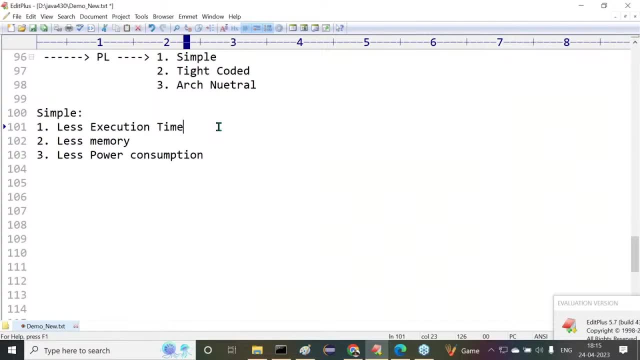 it is asking about the money. when i type it now, within fraction of seconds, that payment is going on in my mobile phone. nearly 28 gb ram is there. section gb is a physical ram and 12 gb is virtual ram. understand it clearly what i'm telling you. the point is not like mobile phone and not like 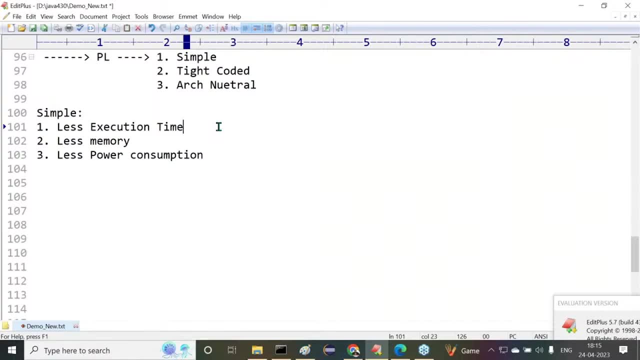 another one: less execution time, more performance, and the user is happy. more execution time, less performance, and the user is not happy. we are preparing all these software products and everything for the sake of satisfying end user. when the end user is happy, then the product is getting very good demand. when any user is not happy, product is not getting or not getting demand. 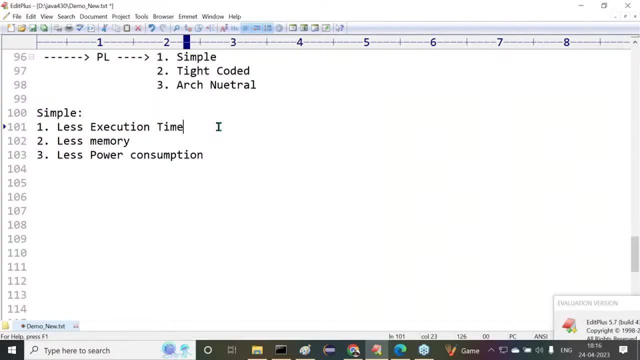 that's why, now the execution time is providing impact or not. execution time is important, factor or not. so because of that reason, sun microsystems wants to prepare their new programming language. sun microsystems wants to prepare a new programming language. it has to take less execution time and it has to provide 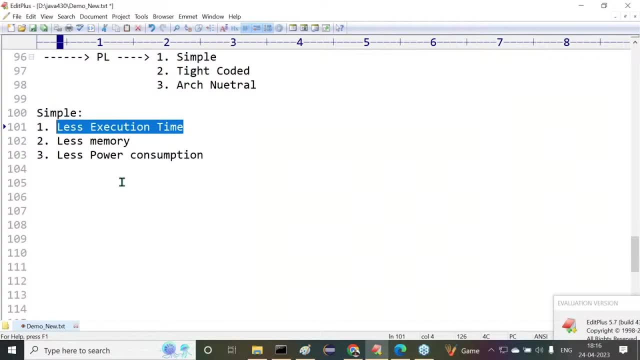 more performance for their applications. that is, sun microsystems wants to prepare a new programming language. it must take less execution time and it has to provide what their: more performance. this is clear-cut information. care what i'm telling you. this is a punch here. next one is: what after? 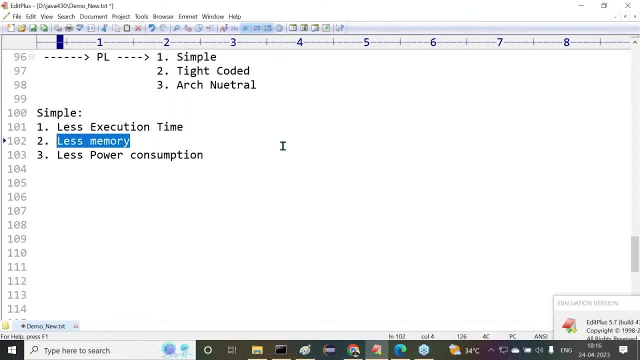 completion of this lesser memory. all of you guys object. carefully, what next one? get less memory. what is this less memory actually? what you are thinking about- less memory- everybody understand it clearly. for example: for example, i want to take a computer. guess, i want to take a laptop. 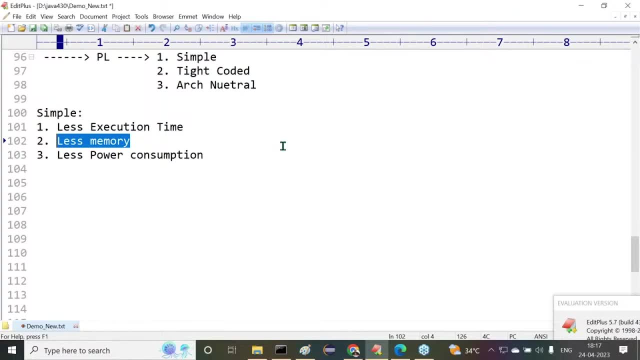 again this example: just one year back. i've taken this laptop previously. i had all in one pc, in the darling one pc. what happened there? by default, they have given memories what they're only four gb ram, lenovo all in one piece. four gb ram they have given. 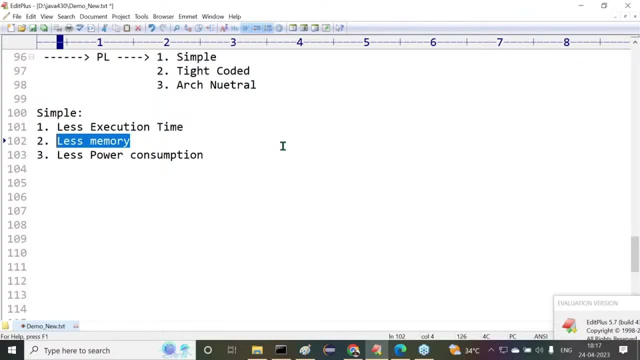 when i'm trying to open my enterprise applications home, then myself is a person i used to take the classes for enter java, maybe advanced java, like what? their frameworks like different, different things. when i open oracle database in my laptop. now it's getting some delay. slow down, totally slow down. 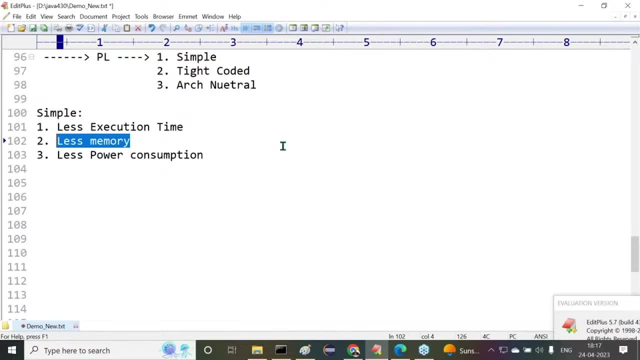 when i open my server, web logic server and uh oracle database, there is totally slow down when i click on this execute button button. there it is taking some time. care, even that eclipse side is not responding in some situation, so i faced a lot of problems there. now, then after that, i 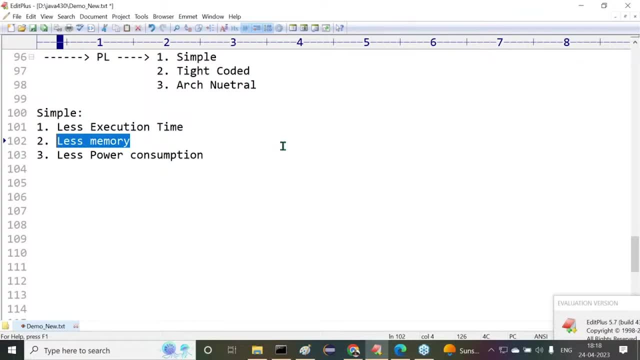 decided i want to take a new laptop. i went to the computer shop. the computer shop might be. there is a representative. i asked him. i want to take a laptop. can i give some like quotation for my laptop? fine, he has given a quotation. what was that quotation he has given there total, all the motherboard and ram. 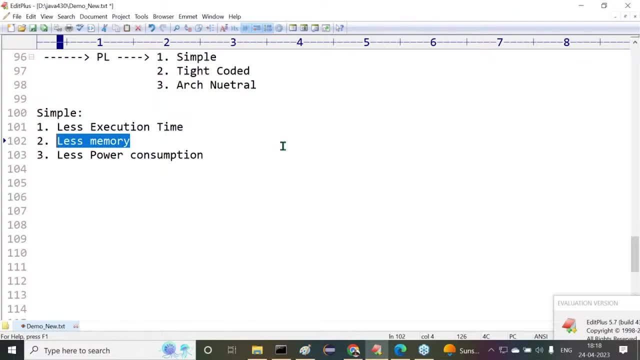 like rom, all peripherals i think he has given there. and finally he said to me the cost of the laptop is 48 000 lenovo, where i've seen that 48 000 they have given. then i observed it, what components they have included. my laptop is 48 000 lenovo and i observed it, what components they have included. 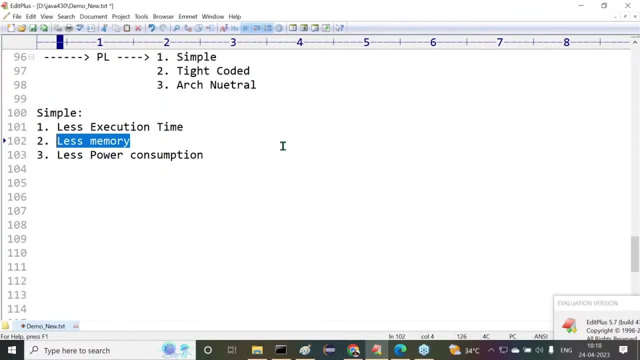 bypassłem, and we've discussed the thought of it actually previously- 4gb ram. it was totally slow down. again, if we take 8gbram, if you open two to three other softwares, no, again it is getting slower or not. again it is a slow. down or not. so now with 8gb ram is the best. I think it is not really Tech, Bénet. if you open, it is just too low. again. what about the como? if you open actually still, six gb ram is showing better generally if you plan to test it. another sentence can change problems and it might take very little. it may close or take other years. if you open 6gb RAM for that it is star. 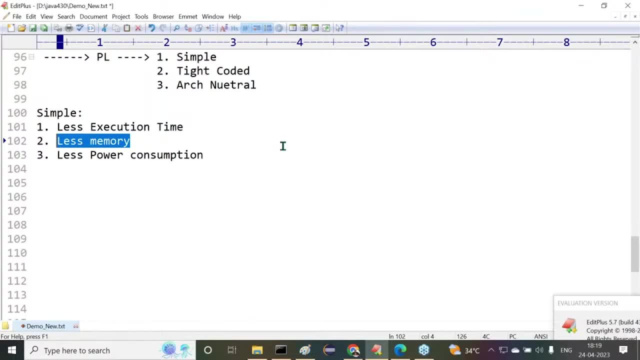 i'm not satisfying with that. just i requested game. can you make it is a 12 gb ram or 16 gb ram like this? yes, okay, no problem, i can take this. you can take directly this one. later i have a service center in my service center. i'm going to make it is 16 gb ram like this. okay then. okay, i accepted. 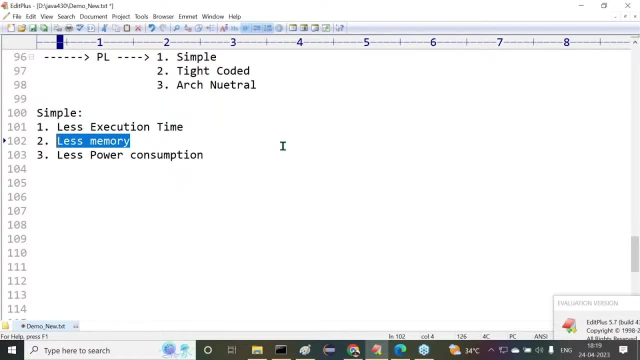 it then immediately has taken that quotation paper where he changed the cost. of cost of the laptop is what they're now this time: 55 000. previously, 48 000. now it is what they're: 58 000, 55 000. what happened? when memory is increased, automatically cost of the product is increased. 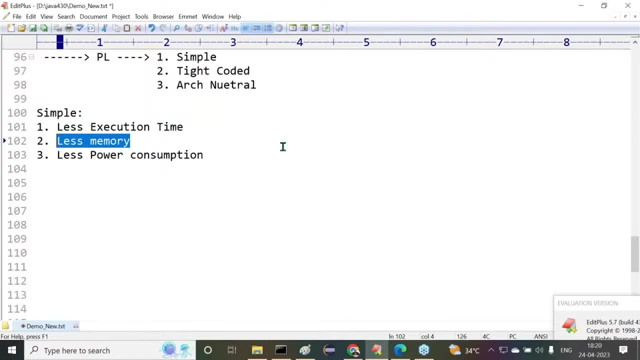 or not. memory is a cost of. when memory is increased automatically, cost of the end product is increased or not. now my laptop- previously 48 000, when i make it is when i made it- is a 16 gb ram like this. okay, now i can take that quotation paper where he changed the cost of. 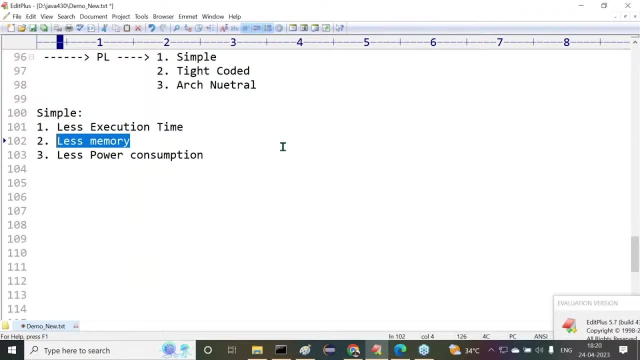 gb ram. automatically it is increased, its cost is increased to 55 000.. so now tell me, if it is more cost, who will take that particular component? we will take that particular product, if it is more cost, who will take it? no, one simple example one. 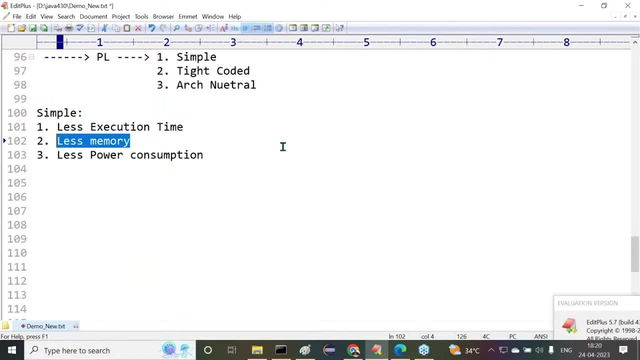 more example i can take the same one plus phone. originally it has number of variants: 16 gb ram, 256 memory. at the same time, 16 gb ram and 512 memory is also available, but that one plus providers have not released 512 memory variant inside in india. why they? 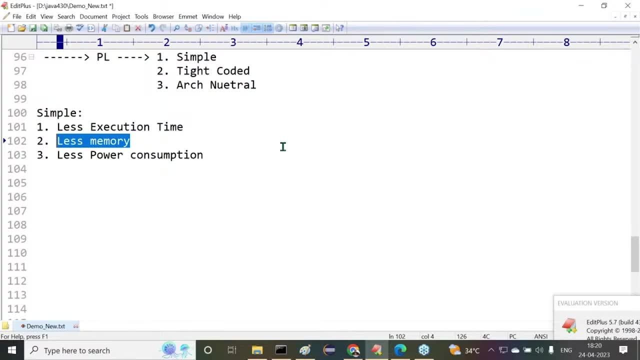 are not introduced. what is the reason for it? no, as for the indian market, 16 gb ram max. as for the indians, psychology, max, majority of people- they are going to buy the mobile phones within the range of like 20, 000, 25, 000 max, 30, 35, less number of people are going. 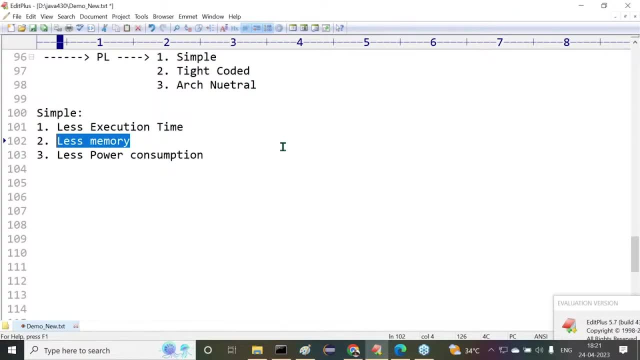 to take the mobile phones up to 50 000 or maybe 70 000.. market is not going to be high for the 70 000 like this 512 variant is having. the cost is nearly 59 000, 60 plus 60 000 plus. 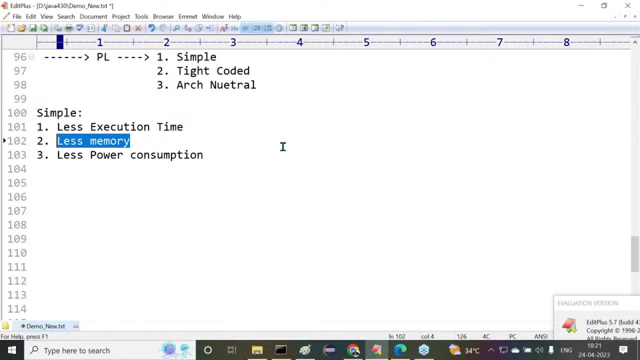 they understood that people are not going to take that mobile phone, they stopped it that variant. they stopped it lower variance. they released it. but in china they are released it and yes, it was released there, but in india only they are not released. why they understood the business, business of indian people, the psychology of 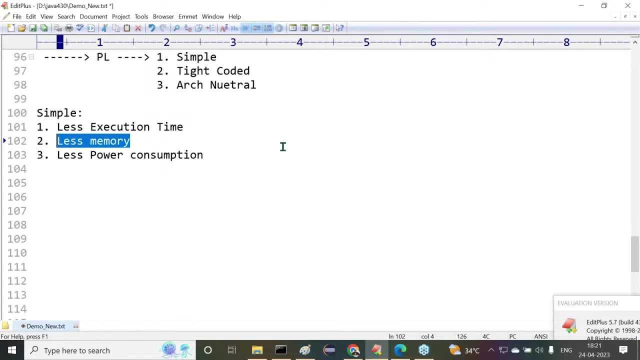 indian people. so which is not going to be taken more because of that, isn't they stopped that variant? you know, memory is the point. is what their memory? and so my point: can, if the cost is more, people are not ready to take that reasonable cost is required or not? okay, 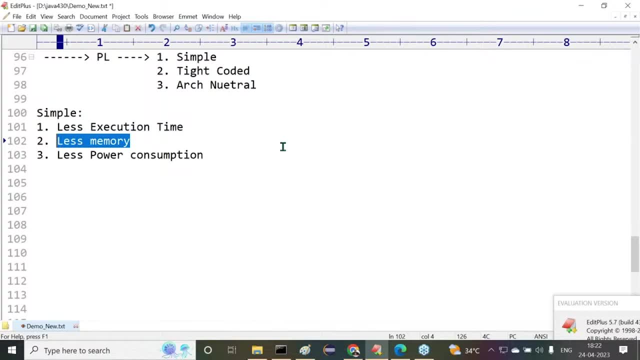 when cost will be increased. when memory is increased, when memory is increased, when memory is reduced, cost of the product is reduced. am i right or not? when memory is increased, cost of the end product will be increased. when memory is lesser, cost of the end product will be lesser. because of that reason, sun micro systems wants to prepare a new programming. 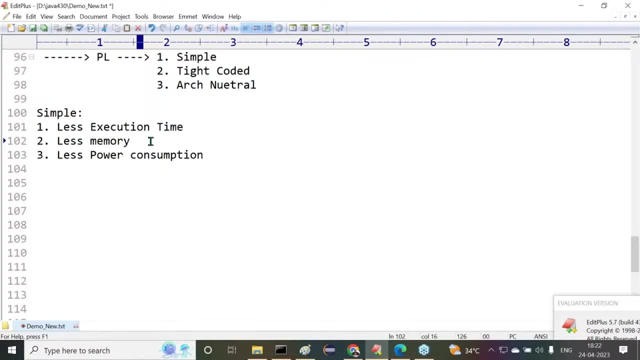 language. it should take. it must take less memory for executing its applications. some micro systems want to prepare a new programming language. it should take. it must take less memory, not more memory within less memory that programs have to be executed in that way. sun microsystems wants to. 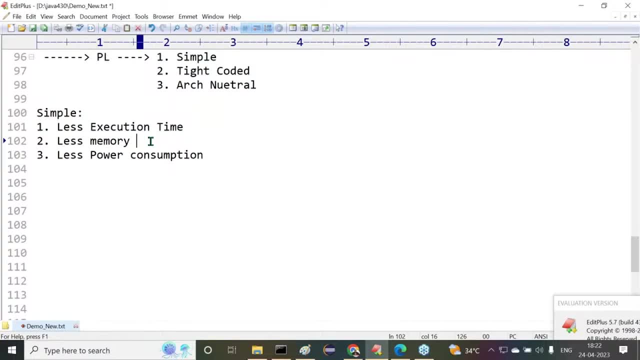 prepare a new programming language. sir, all of you get my point or not? that's okay, fine, let's come to the third point here. what about this third point here? understand it clearly: lesser power consumption. now, this is a punch now coming for this point. what i identified, the content. now try: 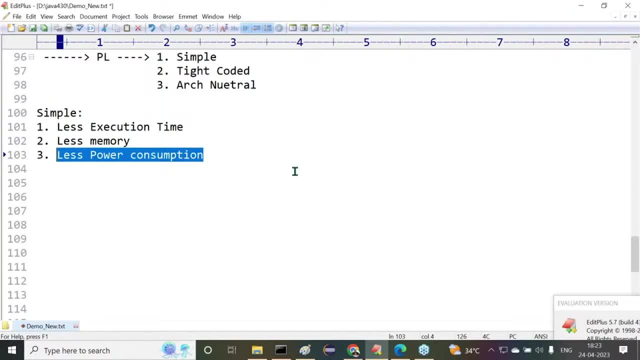 to understand it clearly. for example, if we take remote controller, for example, understand remote controller. remote controller is working on the base of the batteries or not. inside the remote controller, some energy is required or not. so power consumption, power is required or not. that is through batteries that energy will be provided. 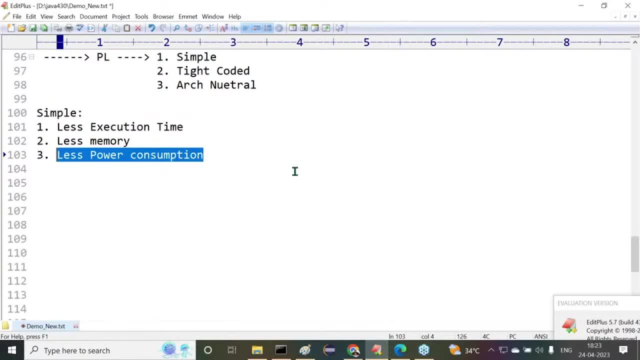 or not. okay, listen carefully. at present, my remote controller must require two batteries. their lifetime is six months of time. for every six months of time i have to change the batteries. the cost of the battery is 100 rupees. so for every six months of time, 100. 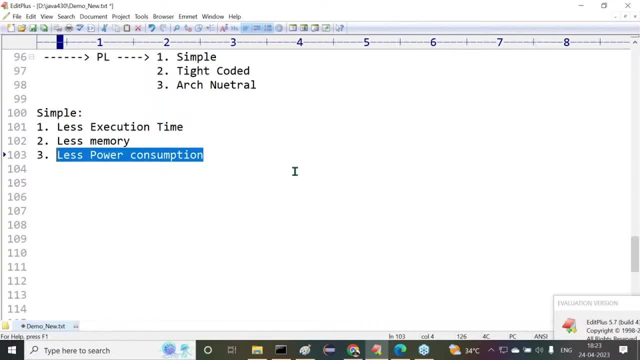 rupees i have to spend for what they're my remote controller. that means maintenance cost of my remote controller for every six months of time is what they're: 100 rupees. listen, clear cut information. okay, fine, leave it after that. if we observe inside the remote, 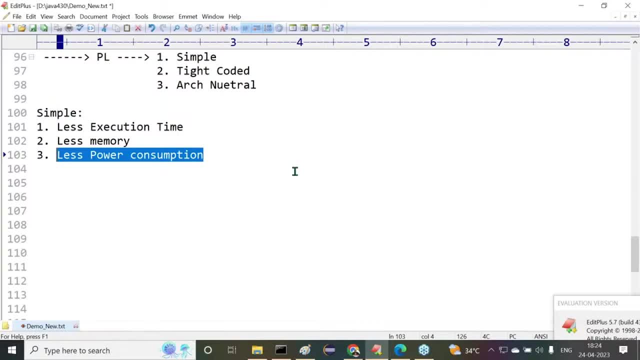 controller. two things are available. one is a software, another one is a hardware. am i right or not? two things are. are available inside the remote controller, software, and hard in every electronic consumer, in electro, any in every electronic device. these two things are mandatory software component and hardware component. when i type some number 7 to previous example,